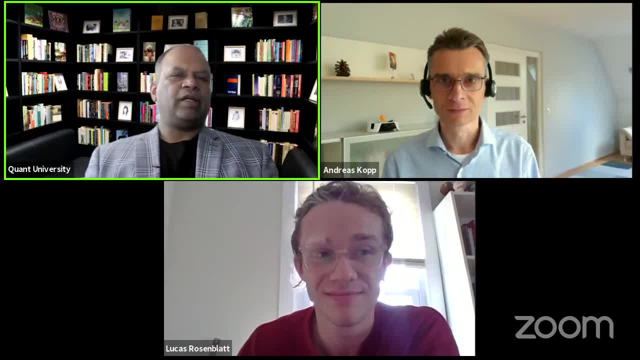 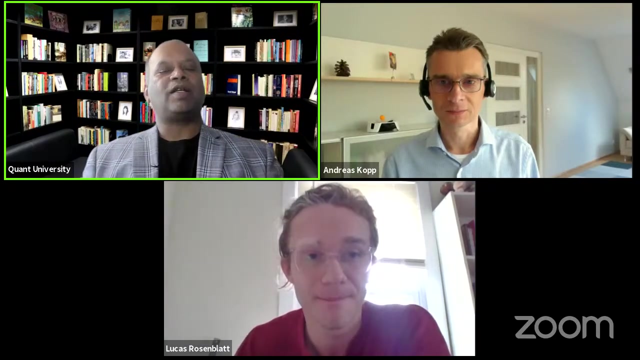 is becoming extremely important, especially in regulated industries like healthcare, finance, government, wherein data security is extremely important, And the last few weeks I've been hearing a lot of discussions wherein people have been pivoting from focusing primarily on the model to looking at the data and looking at how to make the whole pipeline for processing the data more. 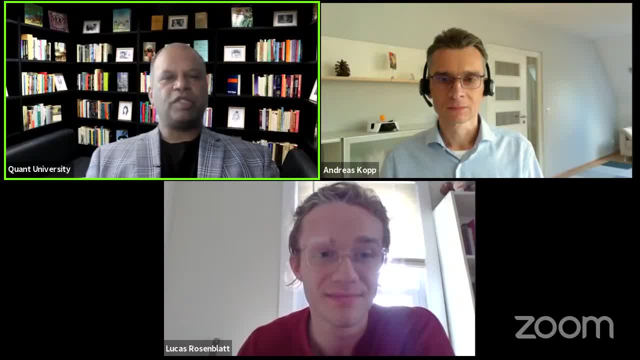 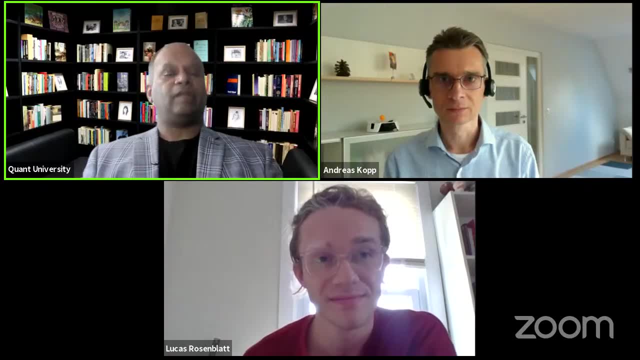 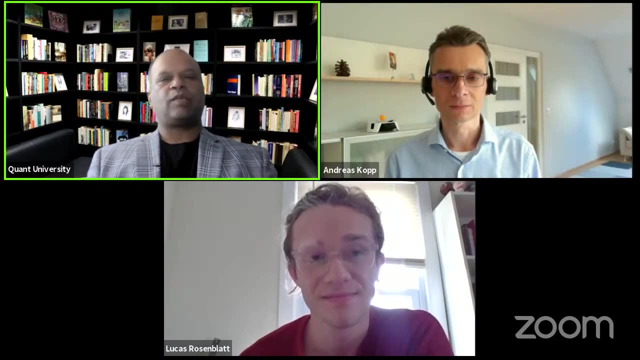 robust. That way, as we productionize more and more machine learning applications, we can think about the ways in which- especially if the data cannot leave the source or the place where it was originally generated, and also aspects about how much transparency we need to. 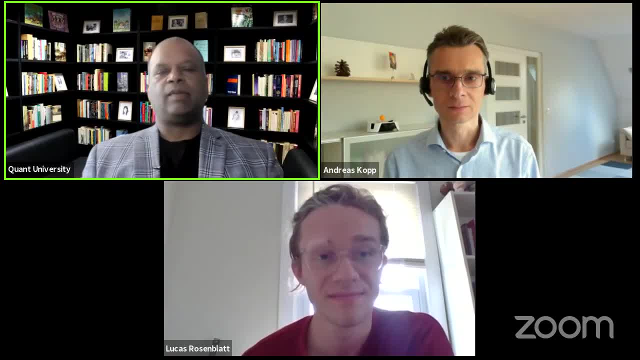 bring into the whole machine learning workflow to make data more and more important as a part of the puzzle. So welcome Andreas and welcome Lucas And for people who are joining in, welcome again. So I would love to kind of start out with our regular way in which we start out. 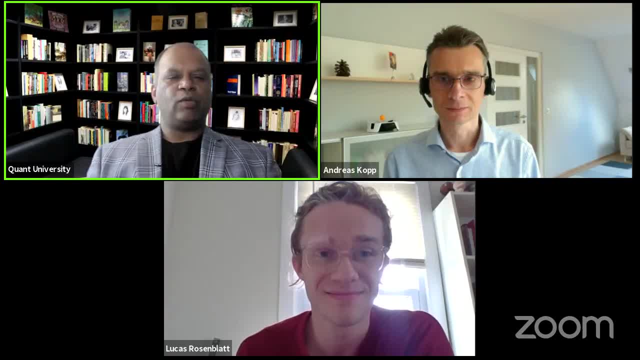 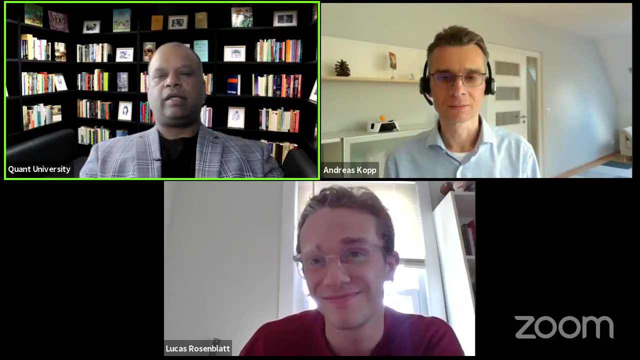 the session. So if you would take a minute and put it in the chat window where you're joining in from, I'd very much appreciate that. Okay, So just take a minute and type in where you're joining in from. I can say Boston. 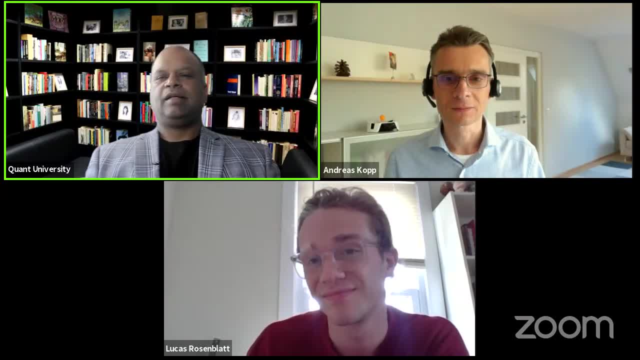 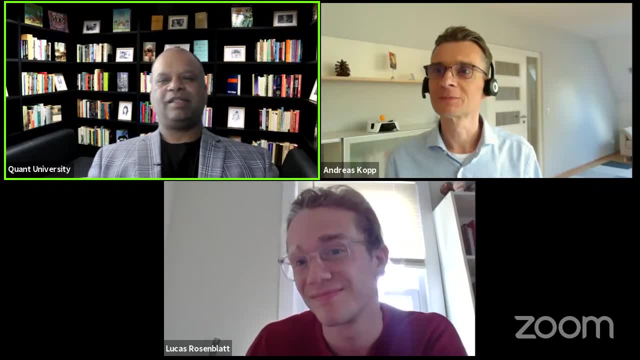 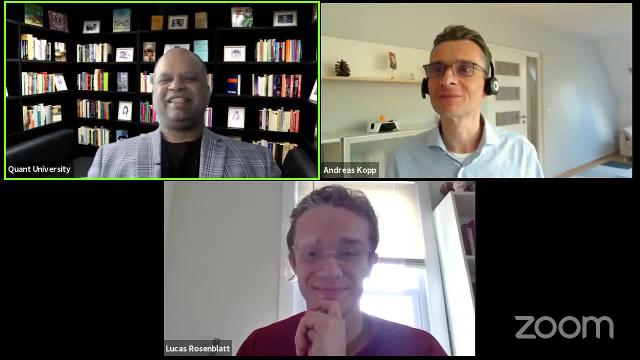 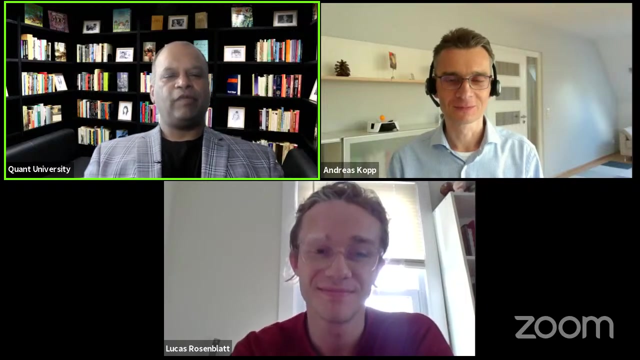 So we have Boston, we have Atlanta. many people from Boston, Baltimore, Montreal, Hamburg, San Jose, Toronto. Yeah, nice to see people from various places joining in, So welcome again. And before I hand over the stage to Andreas and Lucas, just to let you know a couple of logistics. 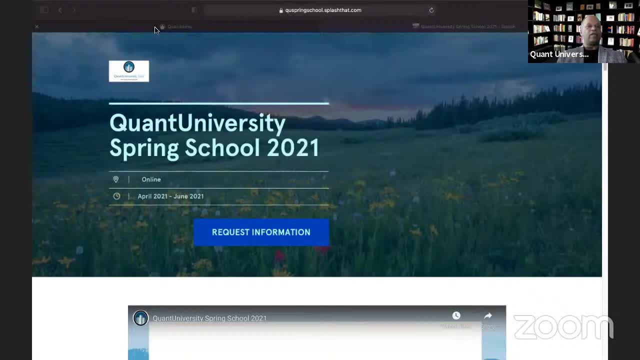 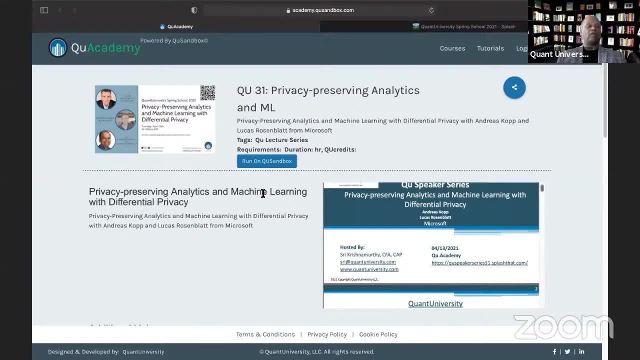 I'm going to make the slides and the video of today's session available on QA Academy afterwards for people who are registered. So if you have not registered to QAAcademy, please go ahead and register And I'll see you in a minute. 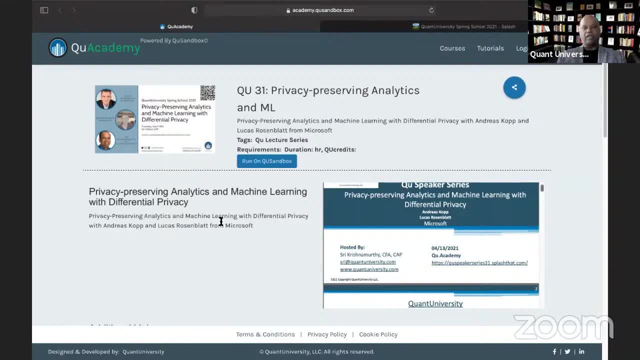 If you create a login and register, you'll have access to today's session and also all the prior sessions and the slides we have been collecting and putting on the platform. So, as we discussed briefly earlier, so today's session is going to be a 90-minute session. We are going to have 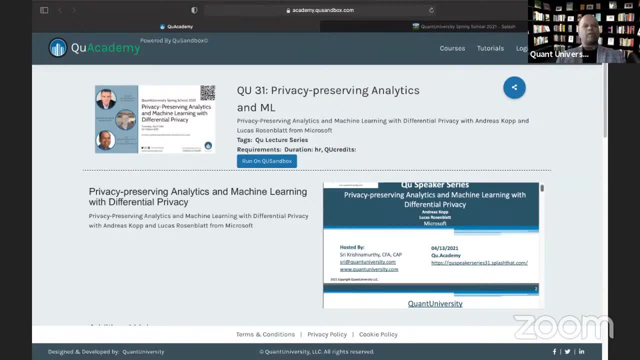 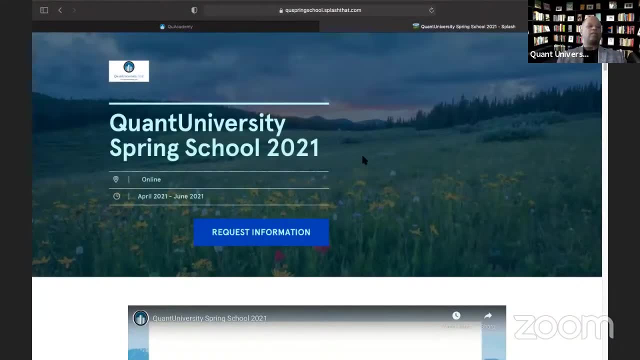 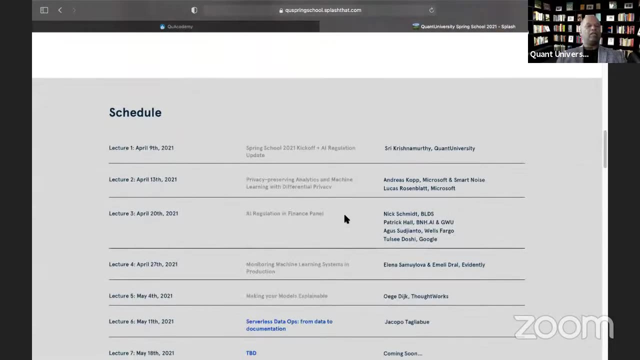 Andreas and Lucas talk about the whole framework about smart noise and differential privacy. For people who are new to the Quant University world, so welcome. So we've been hosting the Quant University Spring School And as a part of the Spring School we have invited eminent speakers and researchers from various institutions throughout the world. 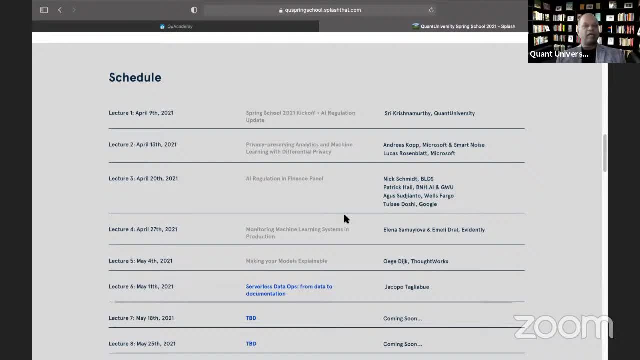 So in today's session we are going to be having the session from Microsoft Next week. we have Nick Schmidt, Patrick, Hall, August, Sugianto and Tulsi, So they come from a diverse perspective. So, Nick and Patrick, they primarily focus on responsible AI-related topics. 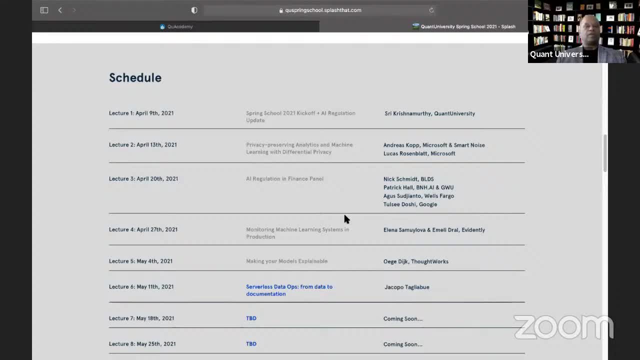 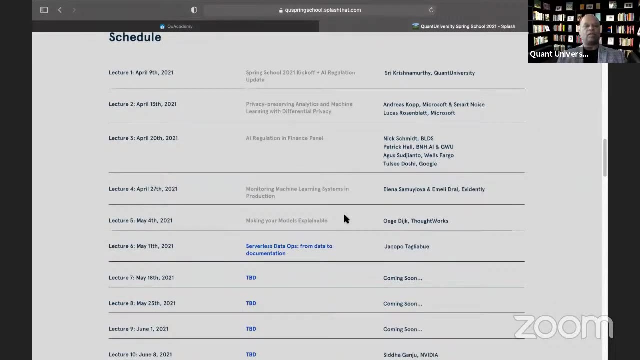 Both from a legal and policy perspective. August, as most of you would know, is at Wells Fargo. He has risk management efforts there And Tulsi is at Google. So she works on the responsible AI side of things, And in April 27th we have a session on monitoring machine learning applications by 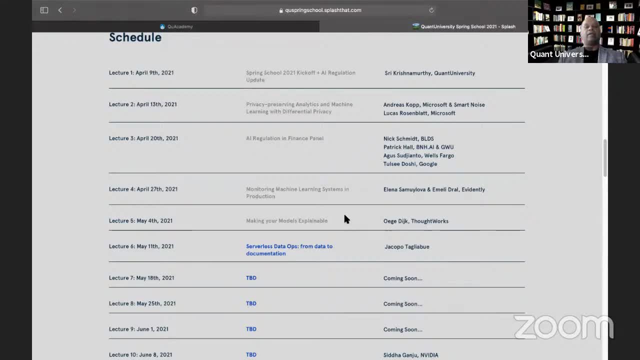 Elena and Emily from evidentlyai, And they are based out of Germany and St Petersburg, Russia, So I'm looking forward to that session And after that, Oge Deick from ThoughtWorks. he's been working on this explainability dashboard. 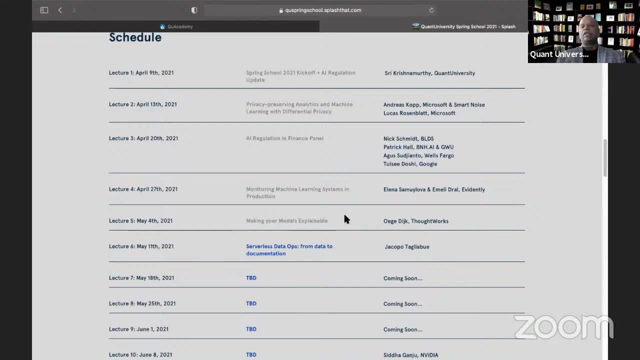 And he's going to be presenting on a session on how to make models explainable. So if you're interested in explainability and you're looking forward to some open source tooling on explainability dashboards, So that's the session you would like to attend. And then, on May 11th, Jacopo. 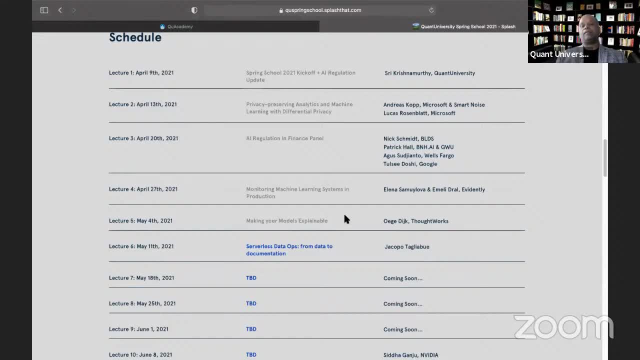 Tagliabue. he's actually currently in Italy and Oge is in the Netherlands, So we have a whole diverse set of speakers from various parts of the world coming to the Quantity University Spring School session. So he actually has a whole session on serverless data ops and I'm really looking forward to that session. 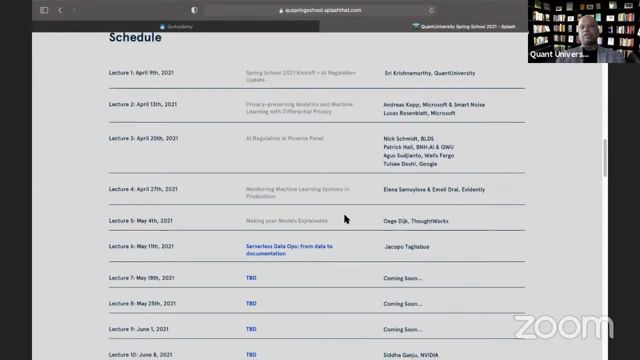 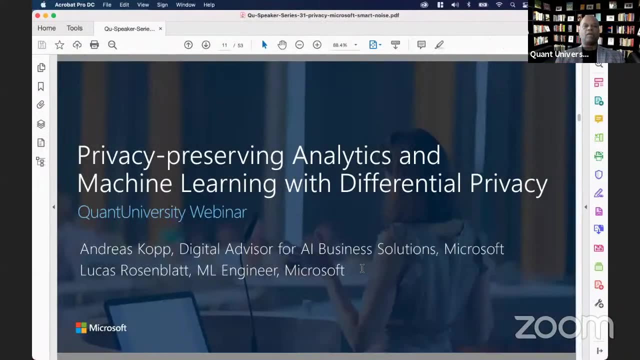 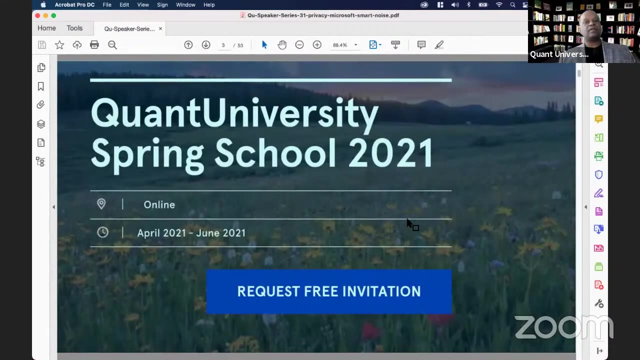 And please look out for the rest of the sessions in the season, which is going to come out soon. I also want to quickly talk about today's session. As you all know, we have been hosting these sessions since summer of 2020, since COVID hit. 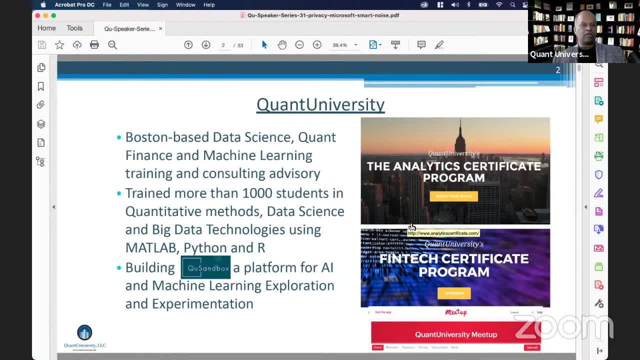 And most of you know that Quantity University is based out of Boston, Massachusetts, And we used to do a lot of live sessions at various parts of the world And since COVID hit, we have been taking all these sessions online And we have had more than 10,000 people attend various sessions since. 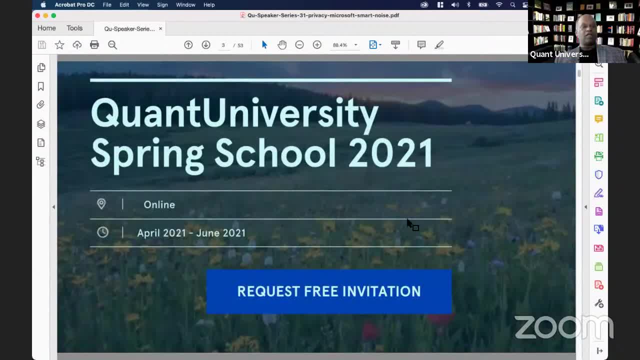 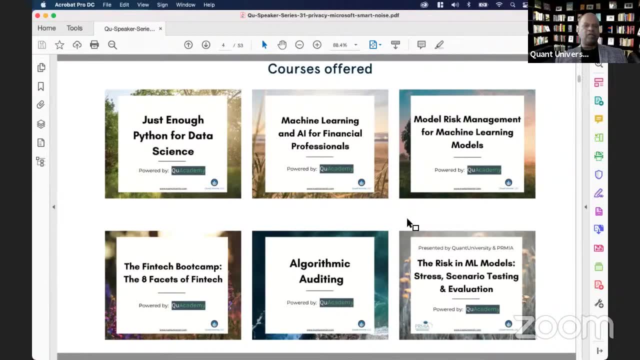 Summer of 2000.. And we are now launching the Spring School and we have a bunch of different courses. We have partnered with Premier And if you're interested in any of the courses, just go to the Premier website or go to our website and you should be able to see all these courses. 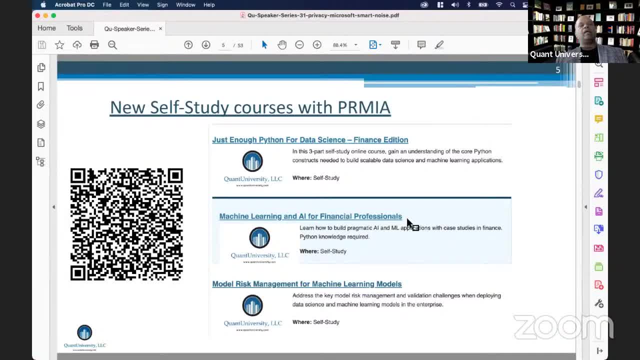 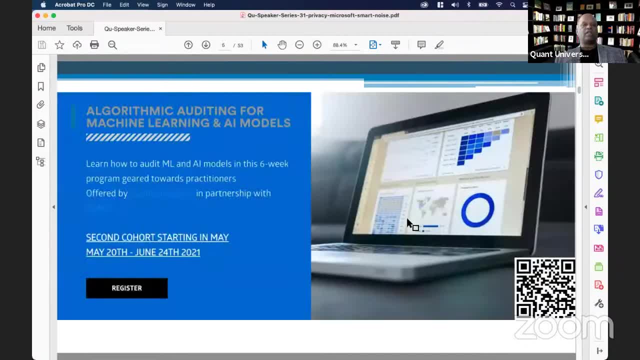 There's also a whole certificate program if you're interested in learning or taking a self-study course in machine learning, primarily focused on finance and associated with model risk concepts And the two courses. There are two courses which I'm extremely happy and we are going. 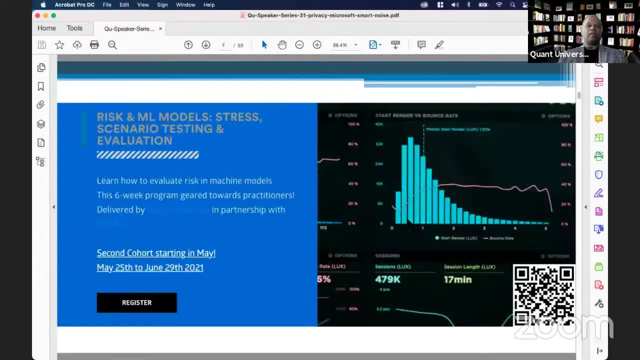 The first cohort is the algorithmic auditing course and another course on risk and machine learning models. So these two courses, the first cohort- we have had people from 11 countries join us and also from various organizations like Ernst & Young, from CIBC, from ING, from Schoenfeld. 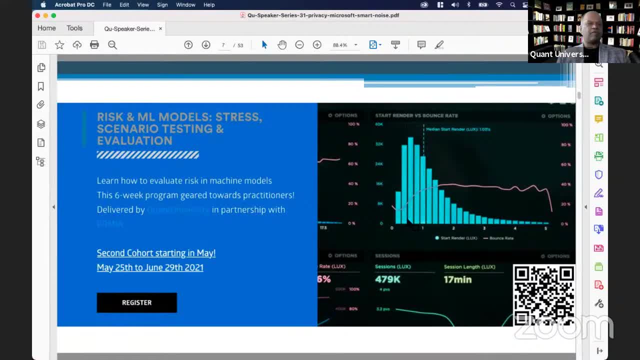 A lot of different companies have taken this course And we have people from South Africa, from Singapore, From India taking these courses. So the second cohort is going to start end of May. So if you're interested, please take a look at our website and you'll have more information there. 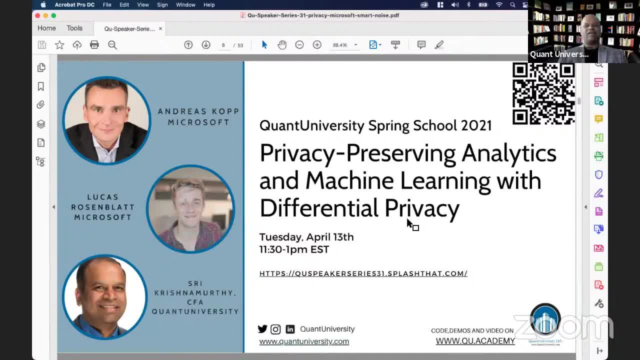 Okay, so today's session, without further ado, will be delivered by Andreas and Lucas. So, Lucas, Andreas, welcome again. Thank you so much for spending your time in the afternoon and also late evening. Andreas, for you for joining us in this session. 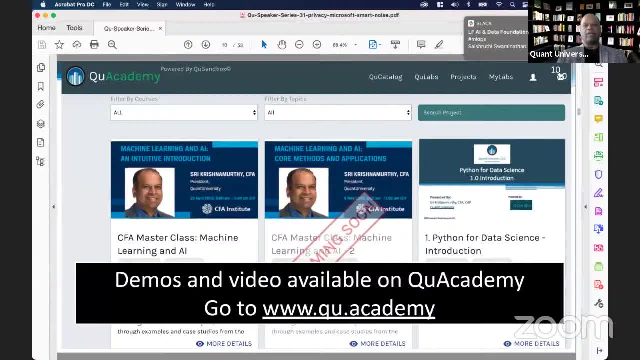 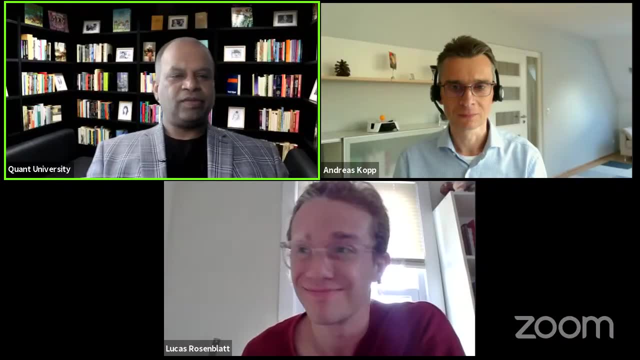 As I mentioned earlier, The slides will be on just a second. let me just remove my notifications will be available on QRata Academy for people who are joining in, So, without further ado, please take it away, Andreas. I'm going to enable you to. so, Andreas, are you going to be starting the session? 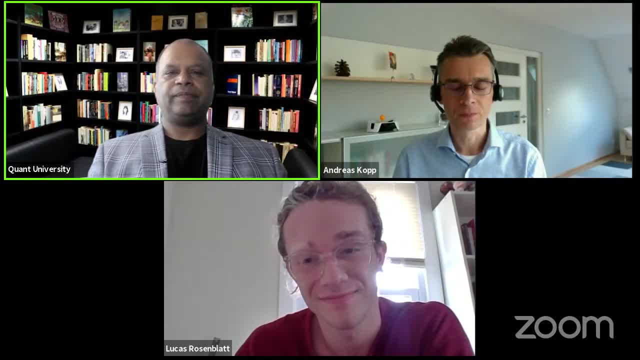 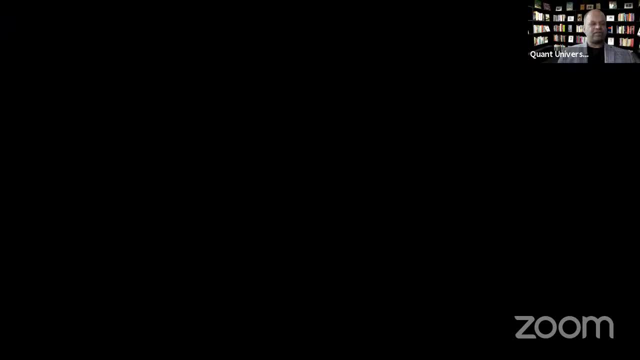 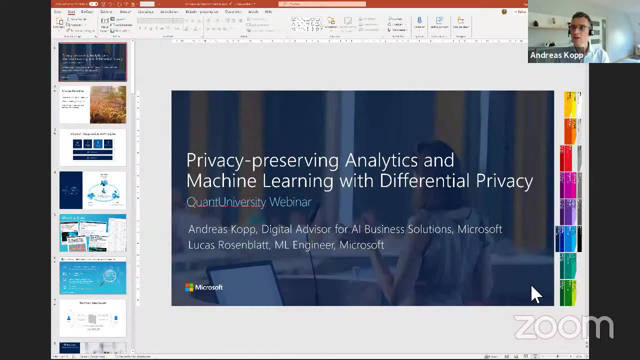 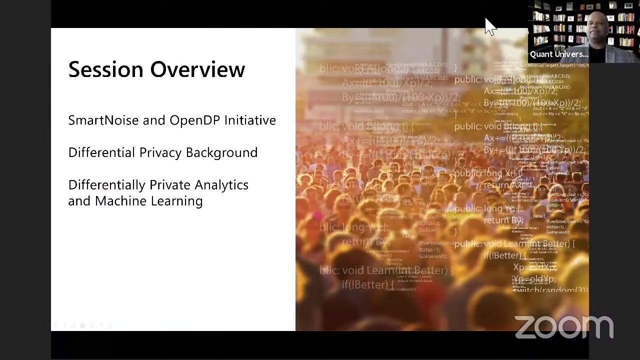 Okay, so I'm going to make you the presenter, Okay, Okay, So you should be able to share your screen, Andreas. Yeah on it. So can you see my screen? Yes, we can see your screen. Perfect, Oops, sorry. 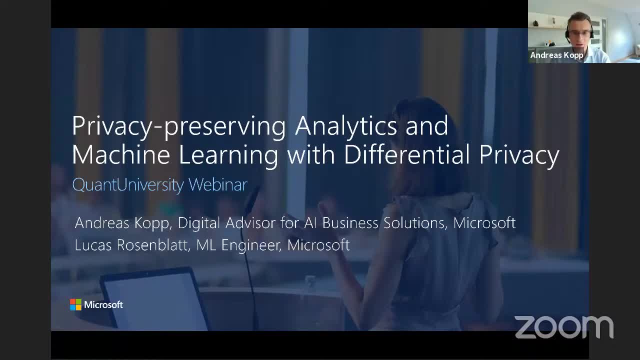 Okay. so first of all, thank you so much for having us really excited to be here, Maybe. Okay, So we're going to have a quick introduction about ourselves. So my name is Andreas Kopp. I'm actually working in the Microsoft Consulting organization. 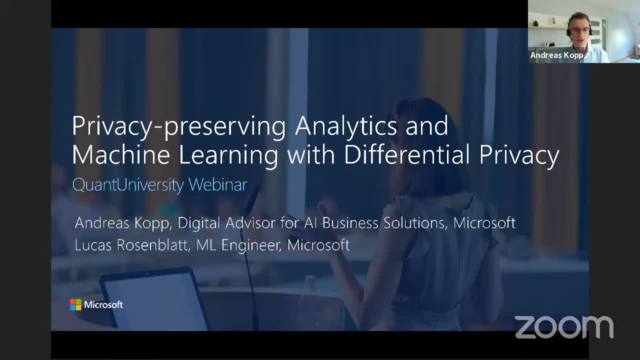 The role is digital advisor, which is actually kind of a generalist role, So I'm providing strategic advice typically to executives of our enterprise customers, So really the large enterprises in Germany. Many digital advisors have one specific topic And in my case that's AI and in particular responsible AI and also the tooling in this context, and differential privacy is one technology which we position there within the overall framework of responsible AI and the toolings. 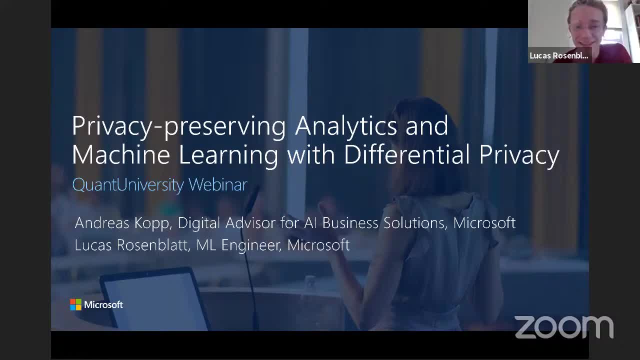 Yeah, so far about myself, Lukas. Yeah, and I am a machine learning engineer on Microsoft's AI development acceleration program team, So that's rotational program And you know it's also sort of a generalist role, but specifically focusing on machine learning across the company. 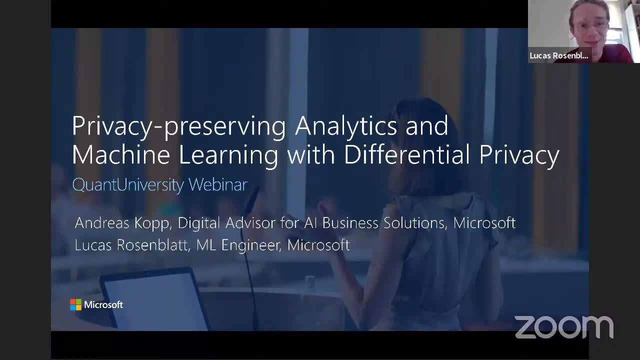 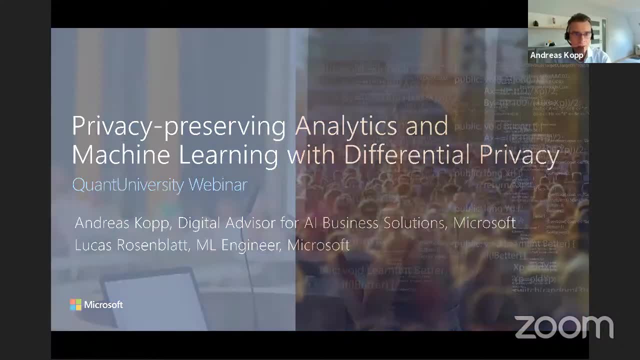 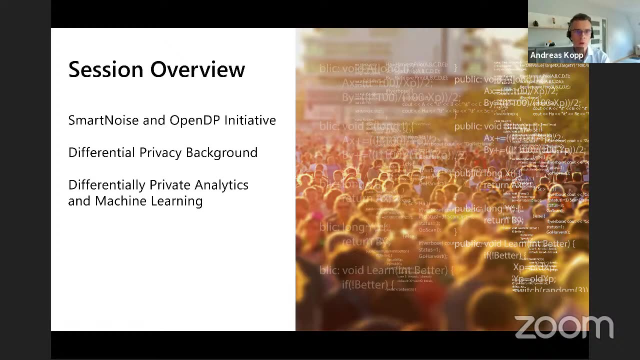 And I found myself focusing on responsible AI as well, So I find myself Great. So what we've prepared is three parts. First, we want to briefly talk about over about our responsible AI framework And how we position things like smart noise or the differential privacy product Microsoft is working on together with Harvard and the Open DP initiative. 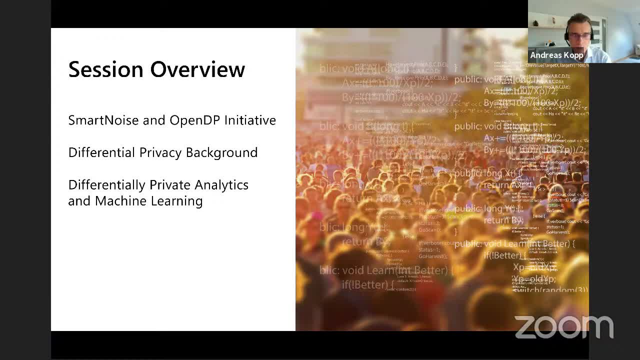 Then we talk a little bit more about the differential privacy background, So really giving an intuition what it is. So this session does not assume any background knowledge when it comes to differential privacy, And then we dive deeper into a couple of use cases For analytics and also machine learning. 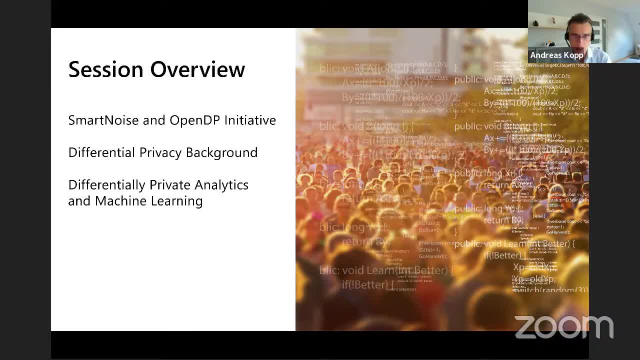 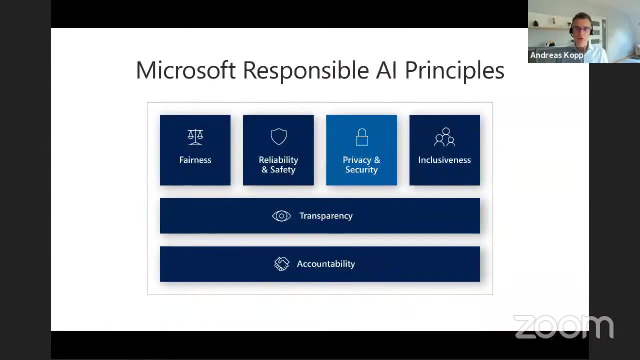 So we have, I think, two to three demos included, So it's not only slides, but you also can see the concept and action. Yeah, And with that I would say, let's get started talking about the bigger framework. As I already mentioned, Microsoft is positioning differential privacy as other topics within the broader context. 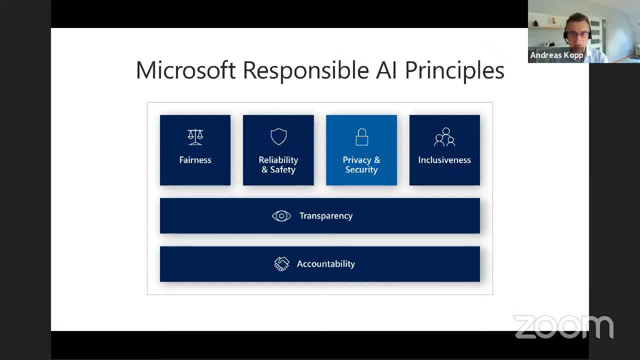 So I see in the code I now have a couple more steps in the skills-based practice group- Beautiful, Thank you, Jimny. Awesome, So we have solving all. let's see just some other example. So let's start with Erg後 and then I think we can start. 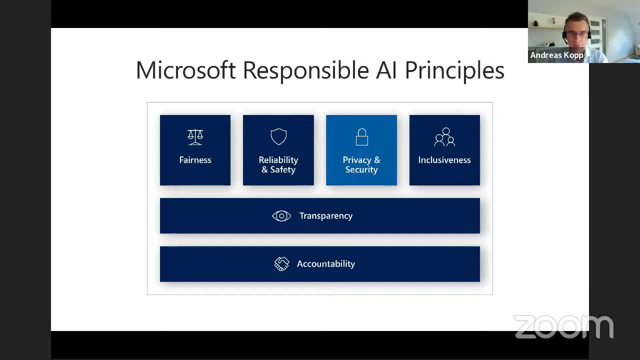 Okay With that. Yeah, So let's take a few minutes. So I want to ask: don' diminished, if you feel project that we are doing and this is what I experience every day. There is also a kind of monitoring of projects if we are engaging with customers and there are potentially sensitive. 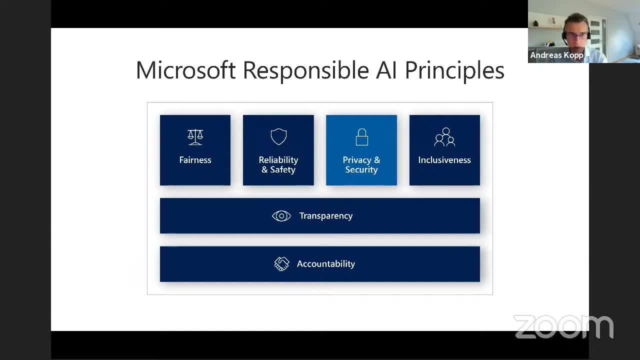 uses related to AI. This has to be approved by a particular board to ensure that these principles, these AI principles, these responsible AI principles, are also followed not only within the product development, but also in our customer engagements. We have these six principles, I think. 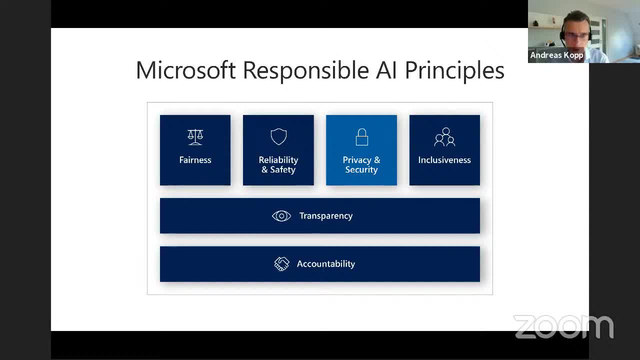 if you look at them, all make sense. Probably everybody would agree. Fairness makes sense. AI systems have to be reliable and safe and also privacy preserving and secure. On that high level, everything is fine. The question always is: what can customers do to set these principles into? 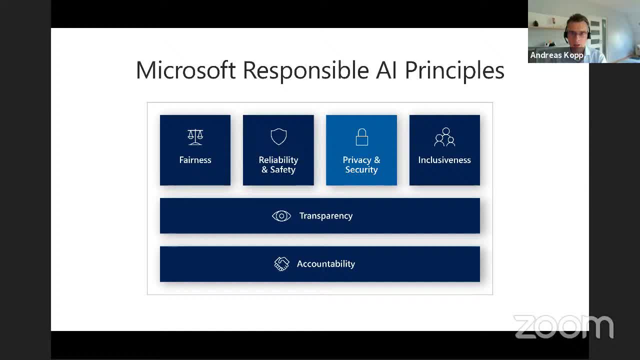 action. What are you doing with that? We have kind of frameworks which help to approach, to realize those principles and projects, like a kind of harms assessment, really to identify what are the stakeholders for an upcoming AI solution, Maybe also including stakeholders or affected people we did not think about at first, and then find out: is there potential harm to these people and what? 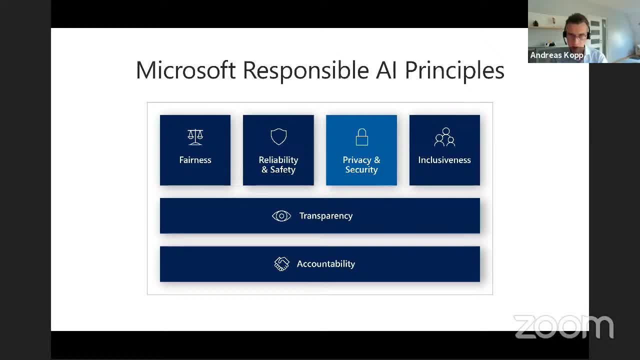 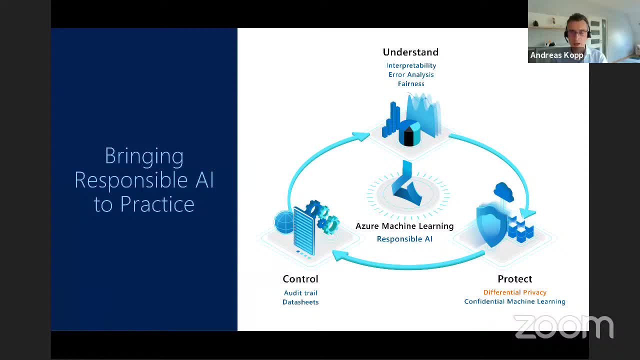 can we do to make sure that we are able to do that? I think that's a really good question. I think we have to work out what are the main aspects that we are able to do to minimize harm. This is more the framework part, the organizational part, but then there is also a tool set part. Really looking. 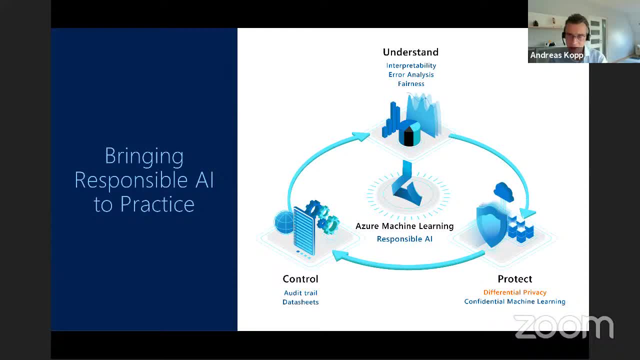 into models, for example, to understand how they behave. We structure the tool set into three buckets. One is understand. This is about explainability: interpretability, Really providing models, but also providing black box explainers to really understand the behavior of models. 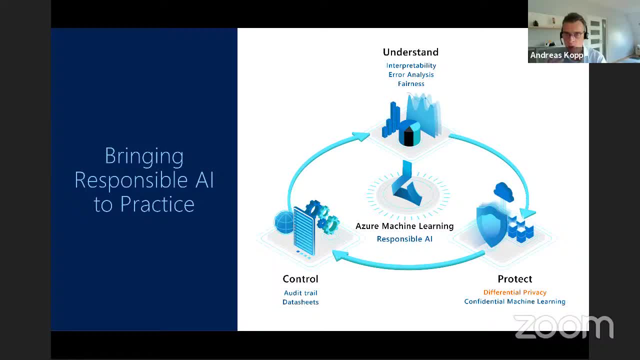 overall, but also understand what was the driver behind a specific prediction. Then there is a new tool which has been released just a couple of weeks ago, the error analyzers tool, which helps you to identify specific error behavior within specific cohorts in your data set. 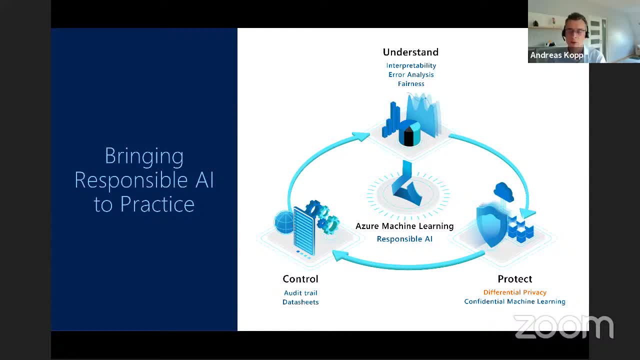 So maybe you look at the classification report: overall everything looks good, but then you find out that for a specific cohort, for example, for women of a specific age, the model does behave significantly worse than overall. And then we have things like FairLearn, which is about identifying bias and also mitigating. 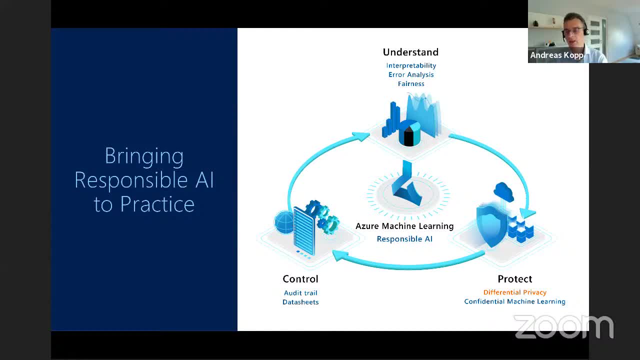 bias within machine learning models And in the context of Protect, which is the second pillar, we have capabilities like confidential machine learning, but also differential privacy, which is the topic of today's talk, And when it comes to control, this is more the process part. 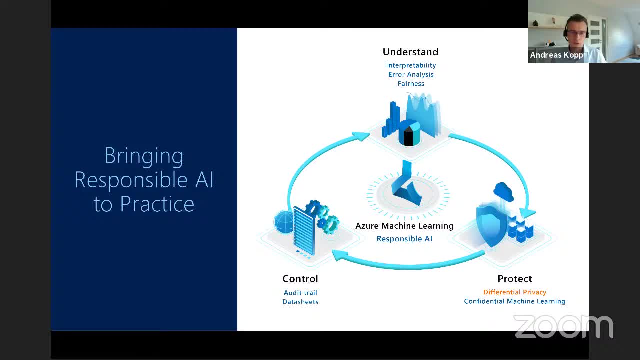 So how do you manage your data sets, How do you manage your experiments and also your models, so that you find out, let's say, 10 months after your model is in production? Well, how is this model? How was it trained? 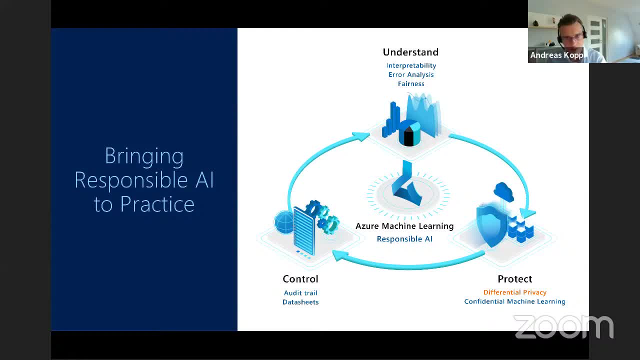 Which were the hyperparameters, Which were the data sets. This is more supporting the overall machine learning life cycles. All of these tools are open source, So there is a clear strategy to provide them as open source tools first, but also to integrate them in the Azure machine learning platform. 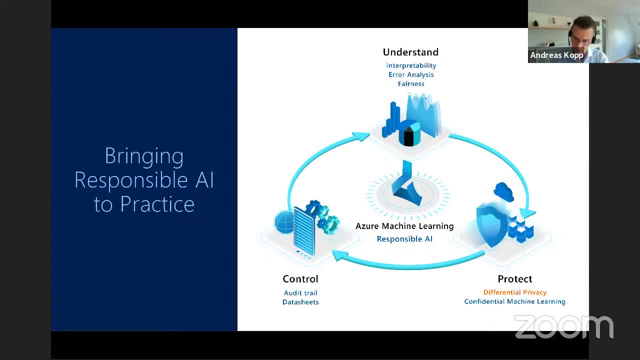 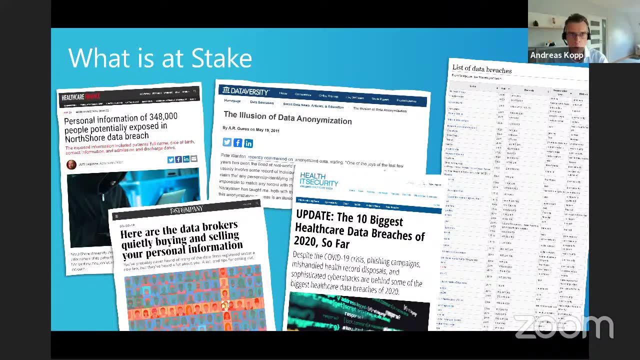 So that's So that they can be used from Azure. And yeah, when it comes to privacy, I don't think that we need a deep dive discussion why this is relevant, If you look at various headlines in the last couple of years or in the last couple of months. 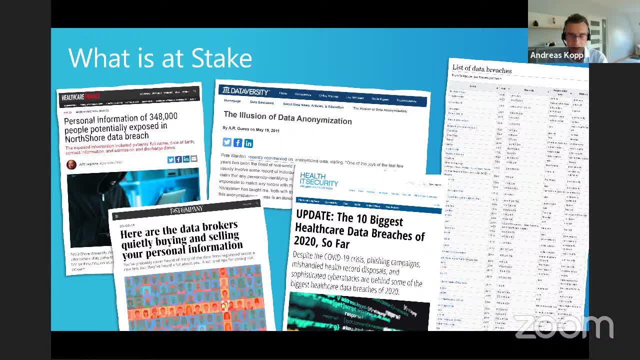 it's a big issue. There are so many data leaks. On the one hand, data is extremely valuable for progress, for research, for society. If we look at The insights we get- COVID-related, for example, it's extremely valuable. 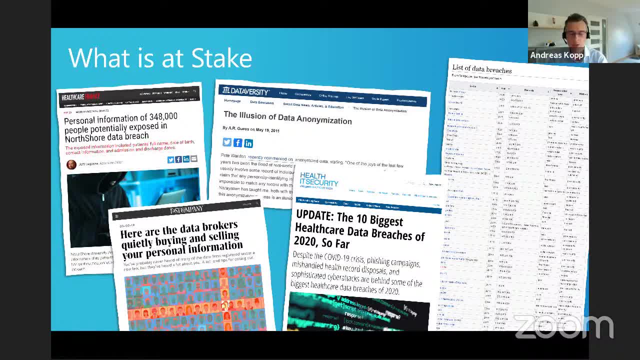 On the other hand, there is a big risk to the individual because we provide more and more data about ourselves and various networks and various social networks And what we find out is that it's relatively easy for adversaries to combine data sets to really learn things about you that are sensitive, that are private, that you don't 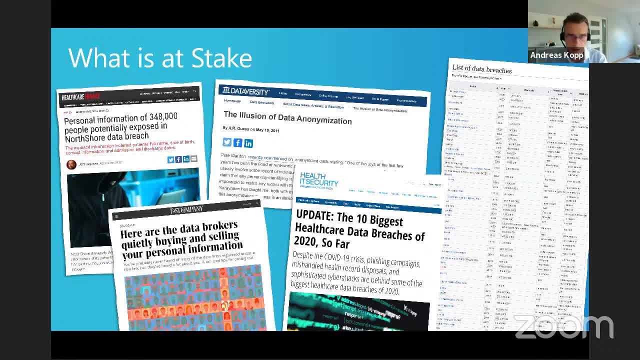 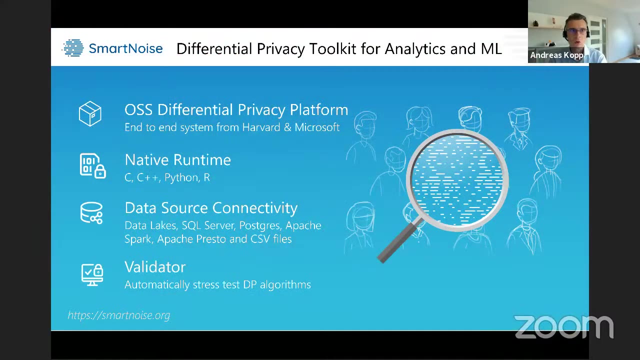 want anyone else To be known about you. So it's a big topic, And this is why differential privacy, which is considered as the new or the upcoming gold standard for privacy protection, is such an important topic. We already mentioned that the product which we provide to the open source is called Smart. 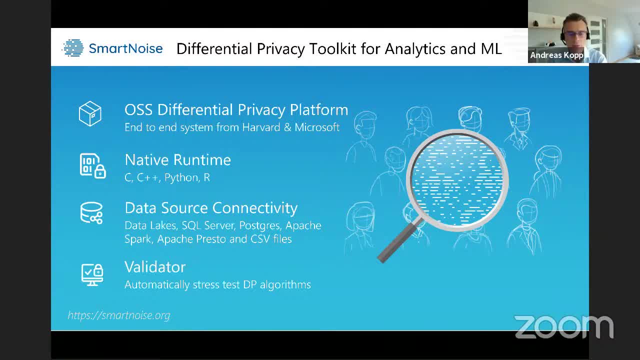 Noise. It had been released in its first version at the Build Conference Last year under the name White Noise, had been renamed to Smart Noise And the idea really is, in this collaboration with the Harvard University, to have an end-to-end. 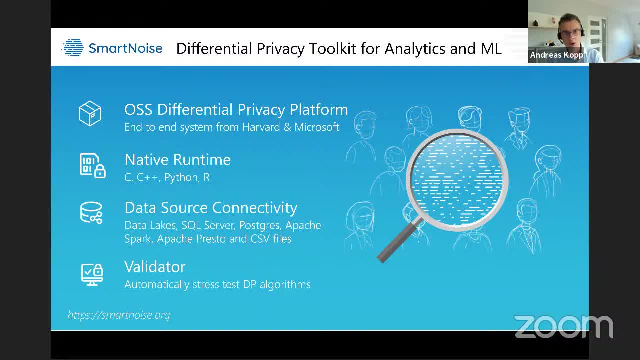 system for practitioners who are not experts in implementing these kind of algorithms, to use differential privacy relatively easily for practitioners. But it is also part of a broader initiative We have launched by Harvard which is called Open Differential Privacy, which is more the community activity to really bring differential privacy forward for the whole community also. 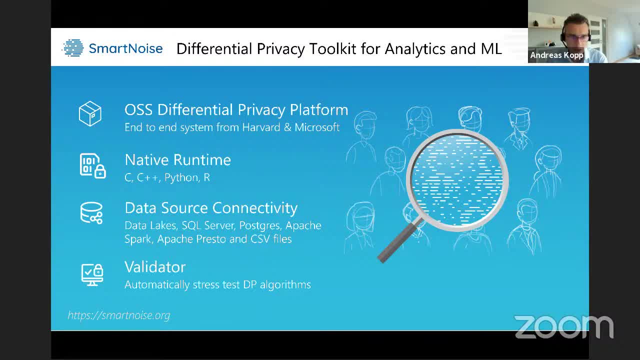 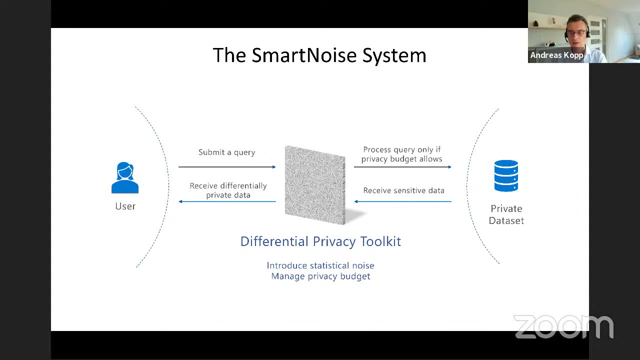 including different research entities, And the concrete product that Harvard and Microsoft are working on is called Smart Noise, And the way it's working is relatively simple. So you have your original data set here on the web. On the right-hand side, this is the, let's say, original unprotected data, which includes a lot of data points about individuals. 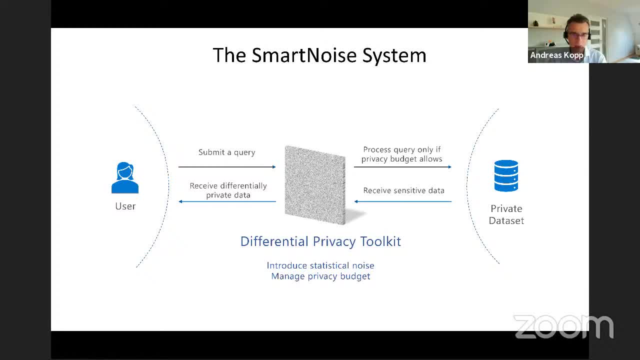 And then you have on the other side you have the user, a kind of analyst who wants to access data, wants to get information about overall patterns within the data set, But we do not want to provide too specific information about individuals, So we provide the user the way to submit a query. 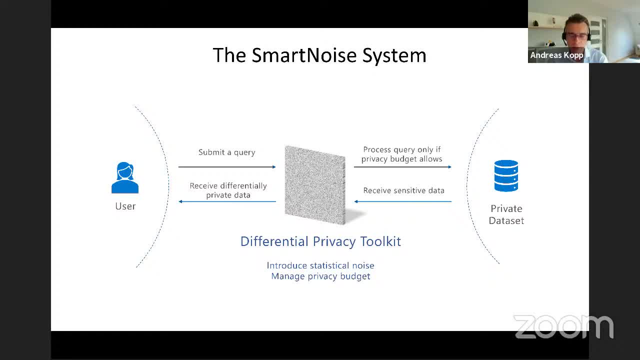 It's executed in the background. Then we add some statistical noise to the data and provide, let's say, statistical aggregate results like counts, averages, histograms or whatever, so that the analyst can get his or her query back or the information that he or she is interested in. 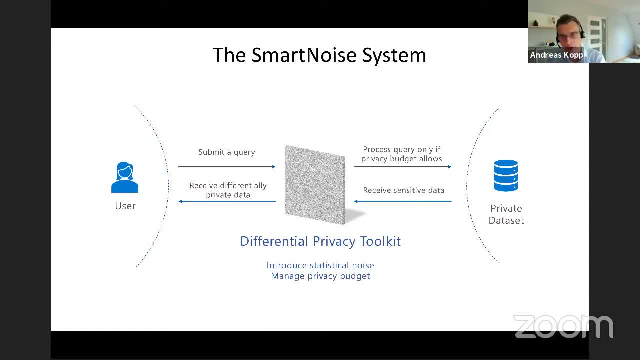 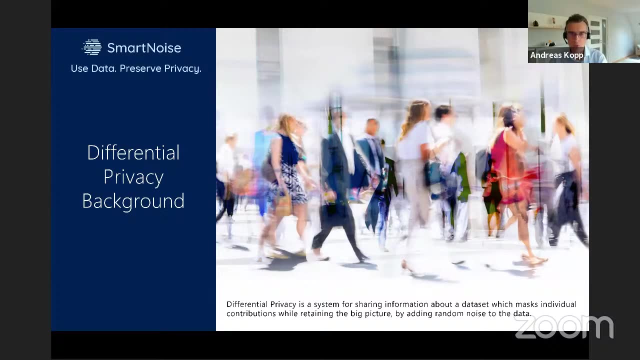 And the way how it works. we will How the data is protected. this is something that we will describe in more detail in this webinar and also show it in action. So really, the main idea- for those of you who have not worked with the term differential privacy before- is that we want to provide information about a big picture, like statistical analysis or machine learning. 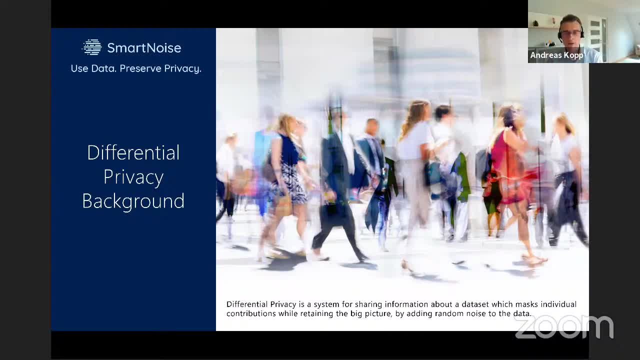 So we want to, for example, learn about the statistical correlation between age and the impact of a COVID infection, But we are not interested in specific data points. For example, we are not interested of the specific medical condition of John Doe, who agreed to participate in our study. 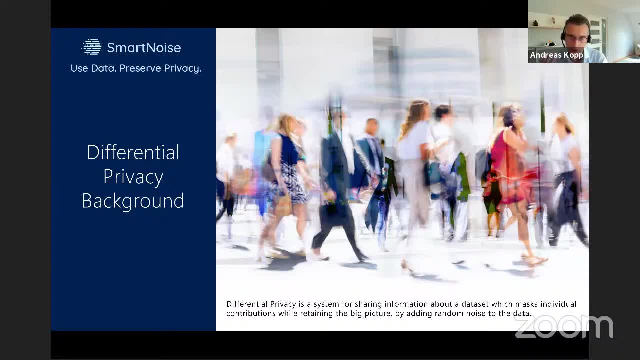 But what we want to do is we want to provide John with a measurable guarantee That his data will not be leaked, so he can, with confidence, participate in our study. That's the main idea of differential privacy. And how are we doing that? 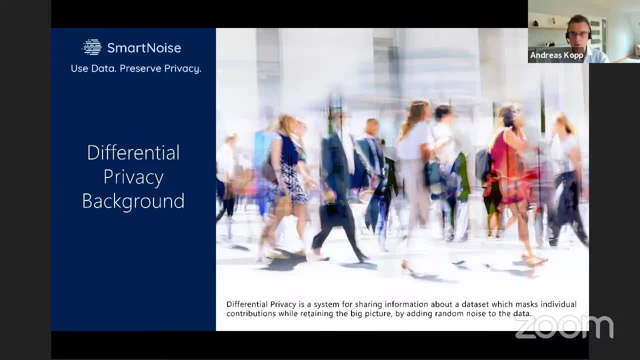 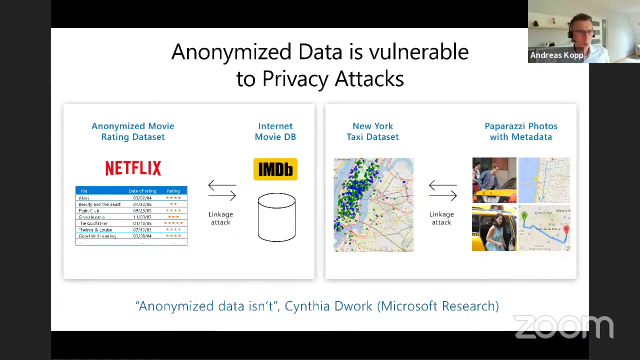 We are adding carefully tuned, random noise to the data and to computations so that the contribution of John, so his individual data point, is masked but the overall big picture is preserved. That's basically the idea of differential privacy. And maybe you would argue: well, what's the problem? 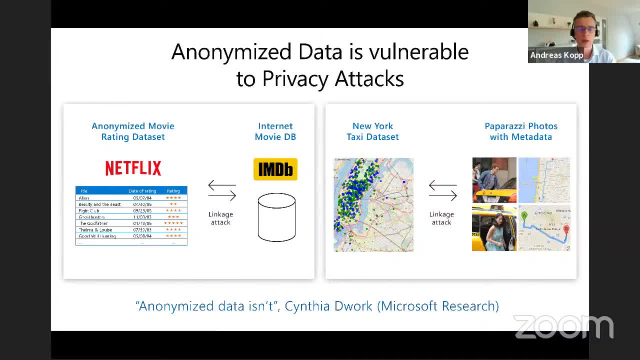 We have this problem today. It's solved. We are working with anonymized data. That's the current practice to protect personal data in many, many cases. And the problem is with anonymized data that it is vulnerable. So you cannot really protect data by anonymization or pseudonymization. 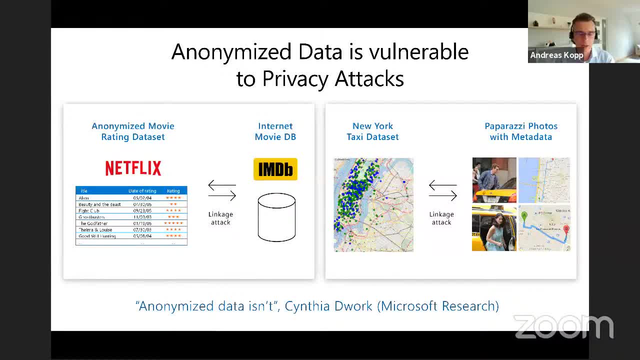 So here are some quite prominent examples to show that anonymized data is really at risk of being reidentified by privacy attacks. For example, Netflix held an open competition a couple of years ago in order to improve their movie ratings, So they provided an anonymized version of their movie rating data set to the public. 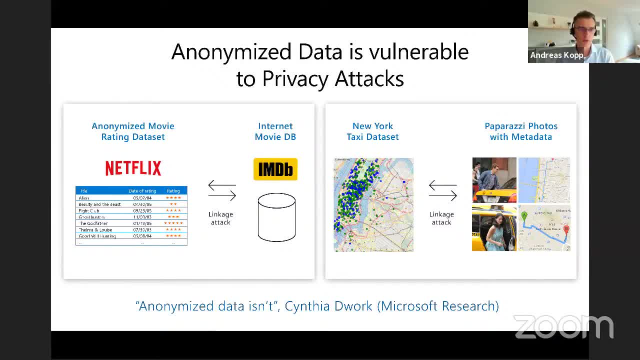 So really no information. what we typically would consider as PII had been included, But it took only, I think, a couple of months until researchers were able to re-identify the people behind the recommendations, behind the ratings by name, by simply linking. 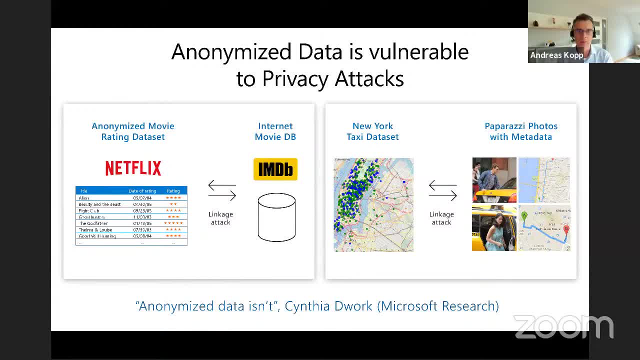 The ratings with the internet movie DB. So this kind of linkage attack was not based on typical PII information like name, gender, age or something like that. The actual key was the ratings themselves, And they were able to re-identify quite a large fraction of the people represented in the data set. 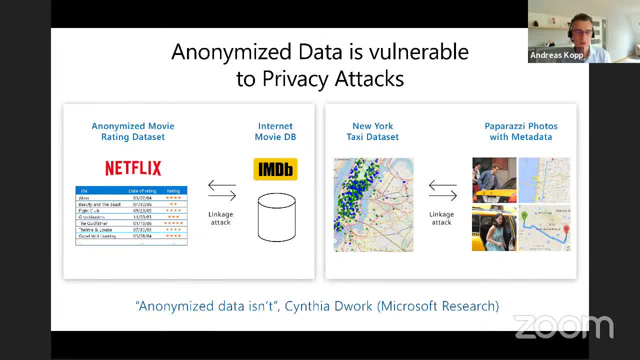 That was a kind of research project. There's also a paper, But the example on the right-hand side is an actual attack. I think many of you probably know the good old New York taxi data set. It also does not include information that we would typically consider as PII. 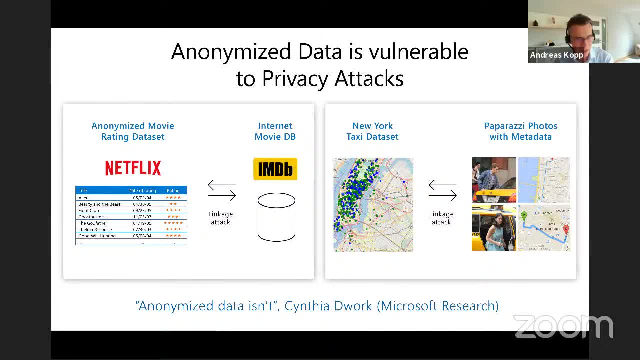 The only information related to the passengers is the number of passengers in the data set, But that's it. And what adversaries were able to leverage was the GPS information. So the start, So the start location. for example, they just linked that with information from gossip websites to identify VIP celebrities, the rights of those people to find out what was the destination address of the celebrity, how much did they pay, how much did they tip, etc. 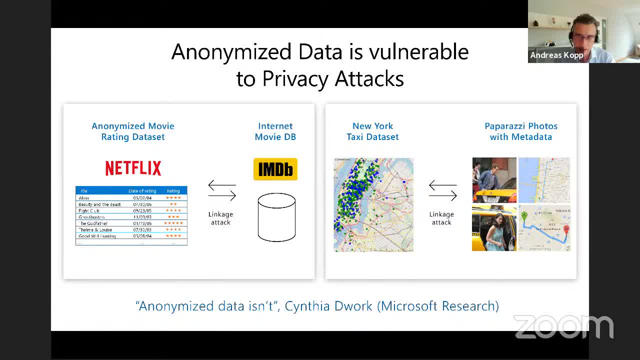 And that is a real-world attack. And the dilemma is summarized By the work by Cynthia Dwork from Microsoft Research, who's one of the inventors of differential privacy that she said anonymized data isn't. So either, the data is not anonymous, because you can still identify people. 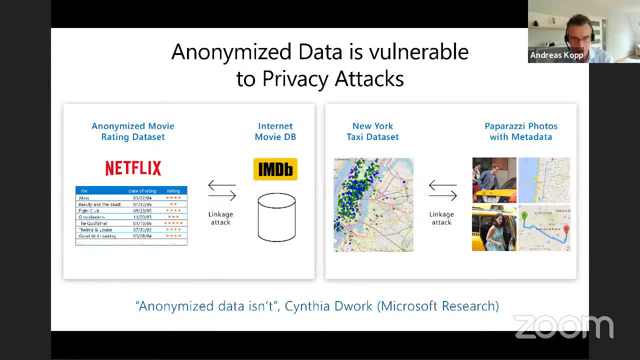 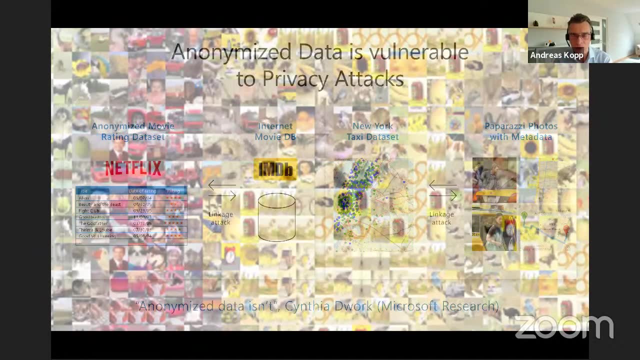 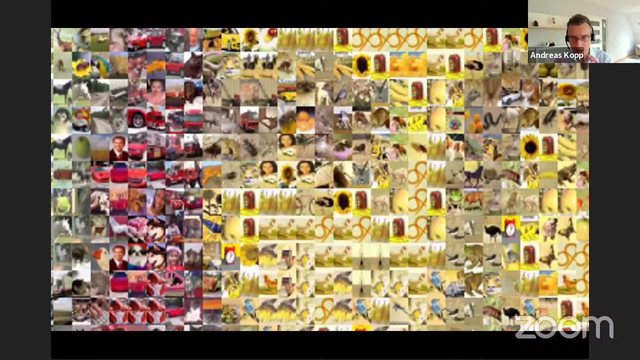 If you really want to ensure that nobody can be identified, you would have to remove so much information from the data that it's not. That's the basic dilemma of data anonymization And the idea of differential privacy. so shout out to the Facebook PyTorch people for providing this example is really to. if you look at all these data points you can see, you can identify. there are faces, there are flowers, for example. 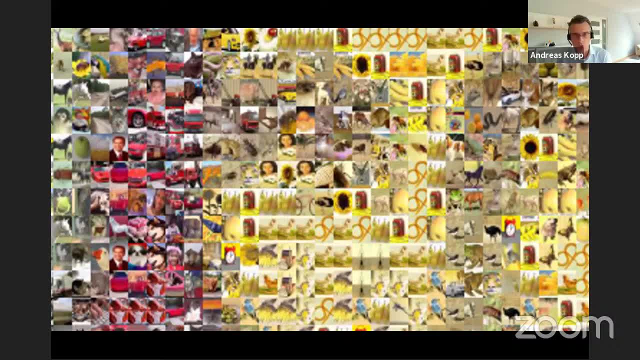 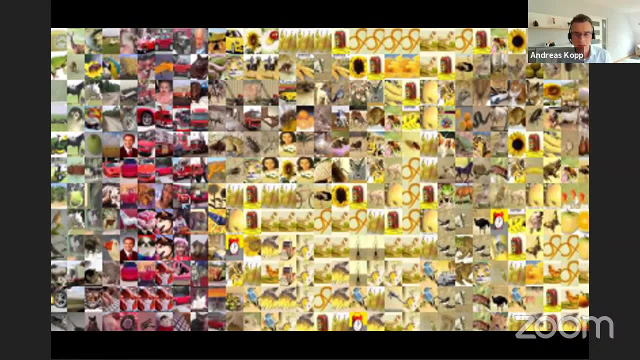 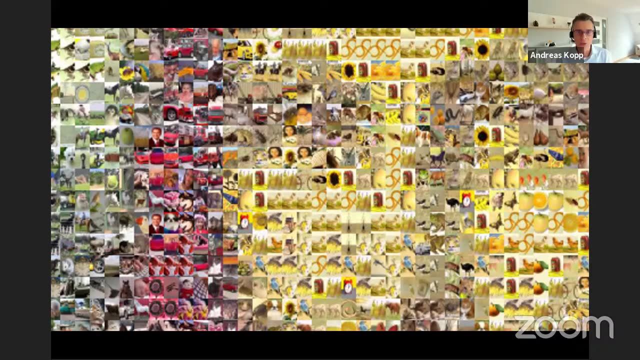 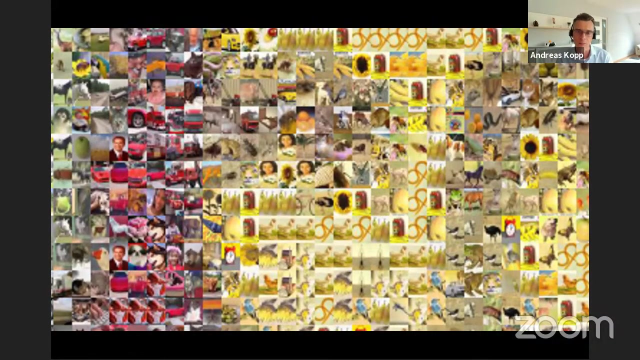 And what we are typically doing when we do machine learning or statistical analysis. we are not interested, as I said, in those data points. We want to see the big picture, which is the painting of Mona Lisa in this case. And the idea is, if we go back to the individual data points, what differential privacy does? it blurs the individual data points. so the individual contribution of the people. 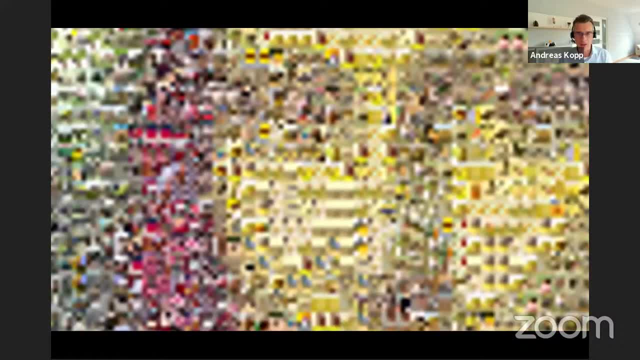 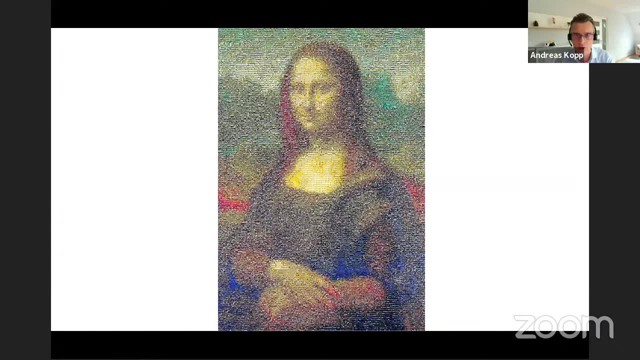 But the big picture, the painting, is essentially the same And this is what we are interested in, And that's basically the idea. I think it's a nice illustration To give an intuition about the idea of differential privacy. Of course, there is also a formal, a strict mathematical definition. 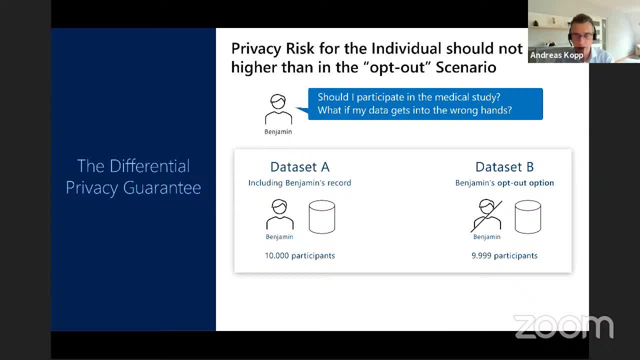 And here's another way to talk about this, For example, if you consider that we have an individual Benjamin, for example. So Benjamin is willing in general, So he wants to support medical progress, So he wants to participate in a medical study. 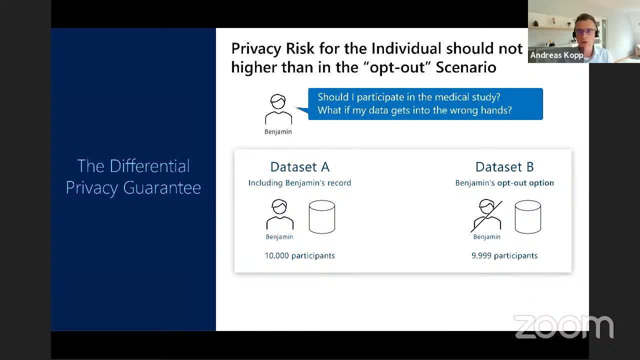 But obviously he doesn't. So on the other hand, he is concerned what could happen if his data point or his data, his record, gets into the wrong hands. And probably the perfect guarantee that we would give Benjamin is that we say we look at it at a risk or from a harms perspective, that we say, well, there are two scenarios. 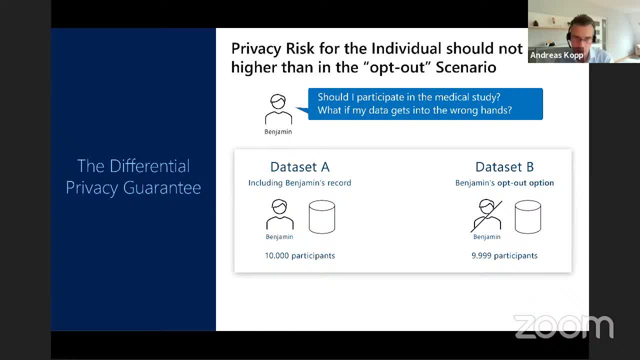 One is the study, including your data point, And then there is the opt-out option. So the same data set. the only difference between data set A and data set B is that Benjamin's record is not included or maybe replaced by another record, And this is the core principle of differential privacy, also where the name differential privacy comes from- that we compare the scenario of the database, including his record, with the scenario of Benjamin's record. 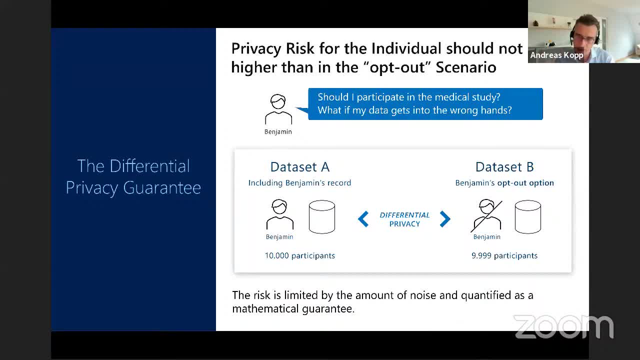 Okay. So what happens when we compare the scenario of the database excluding his record and the promise of differential privacy? is that the risk of data leakage is essentially the same. I'm saying essentially, it's not 100% the same. There is a tuning knob which is called epsilon. 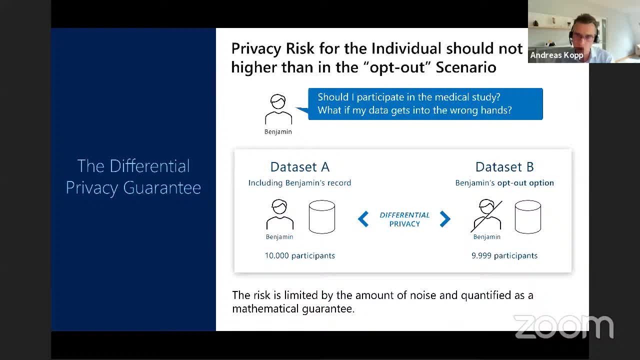 This is the amount of noise which we can use to control the data, the privacy level, and also to control the remaining risk that something could go wrong. But for practical applications, the guarantee to Benjamin is that, even though he participates, if we apply differential privacy, the risk is essentially the same as in the opt-out scenario. 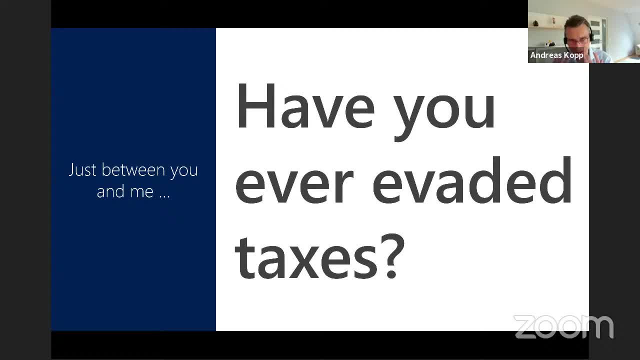 And yeah, maybe to give an idea how it works in practice, so how we can apply random noise, carefully tuned random noise, to the data. here's a practical example which is a little bit older than the differential privacy concept, which is called randomized response. 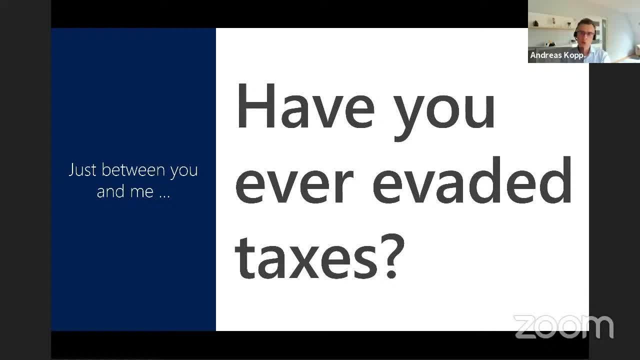 So consider a situation where we want to ask a community or population an extremely sensitive question, like we want to find out about 10%. What happens if we ask that question to the community? So it's clear that you will probably not get honest answers in many, many cases. 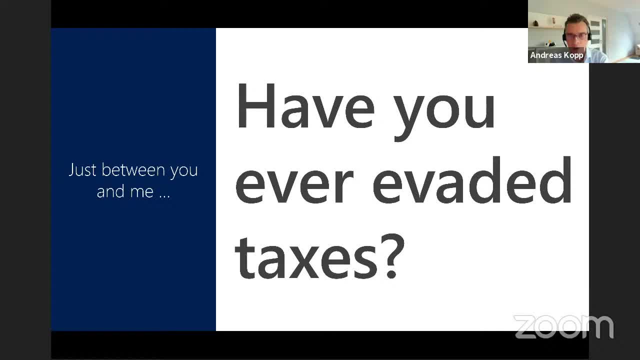 especially not from the tax evaders, in such a setting. So what can we do to ensure that, on the one hand, we get reliable answers, but also that we protect the privacy, even of the tax evaders, even in a situation where the tax investigation? 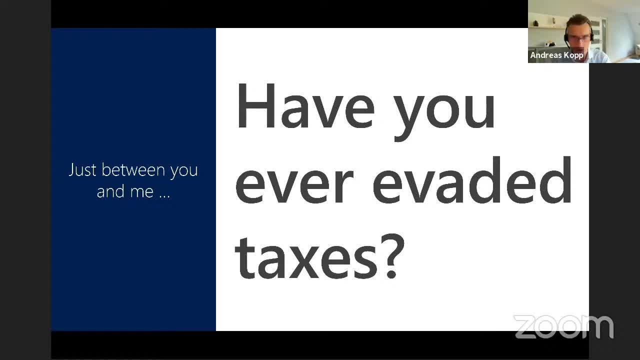 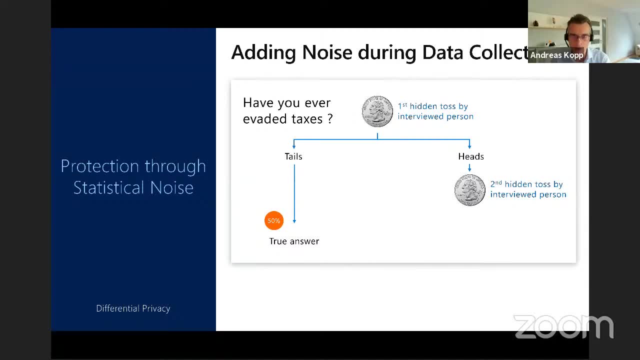 seizes all the records, including the names, And the answer is we leverage randomness. So it's a very simple experiment or a relatively simple setup used in randomized response, I think since the 1960s, and it's relatively straightforward. So we ask the participant to do a hidden coin toss. 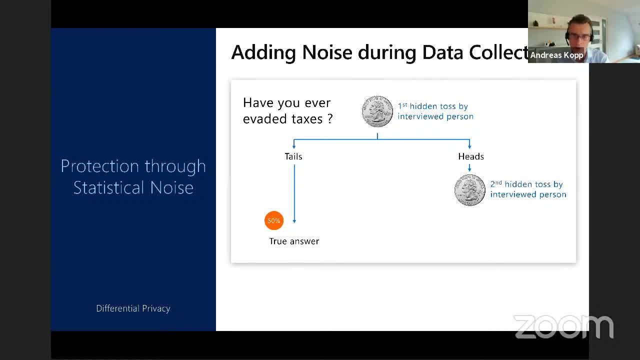 So we do not see what the result of this coin flip is. If the result is tails, the participant is asked to give a true answer. If the result of the coin flip is heads, we ask the participant to flip the coin for a second time. 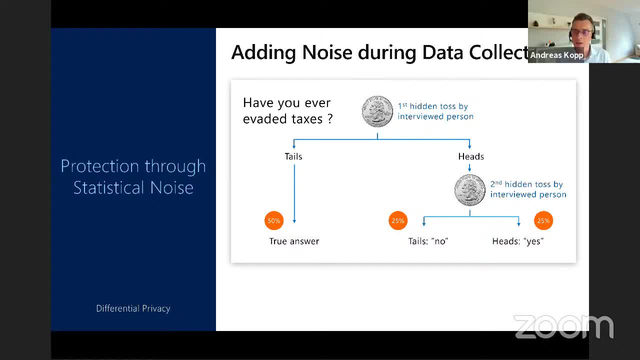 and make his or her answer dependent on the result of the coin flip. So it's a very simple experiment, So it's pure random And everybody is happy with this setup and follows the rules. Then one thing is that we can guarantee to the participants 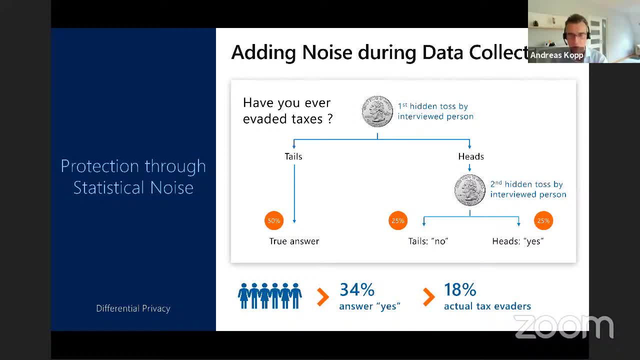 is that they have plausible deniability. So even in the case that all those records, including their names, is seized by the tax investigation, everybody has plausible deniability because they can say: can argue. well, I had to give this answer. 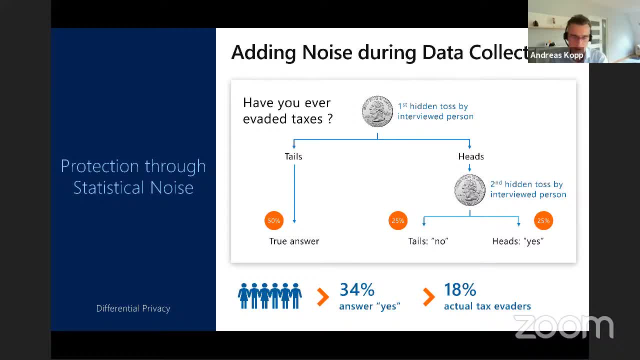 I had to give this answer because of the way the experiment worked, So it is a random answer. But on the other hand we can calculate the actual tax compliance of the population. So if, for example, 34% answer with yes, 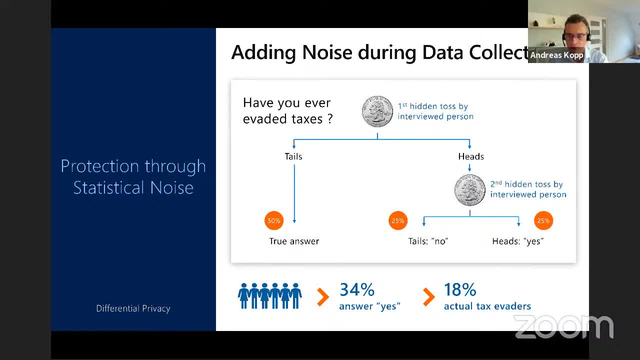 based on the experiment, we can calculate the percentage of actual tax invaders, which is 18% in this case. Of course, in today's differential privacy settings, we are not flipping coins. the noise is added automatically If you consider, for example, Windows 10,. 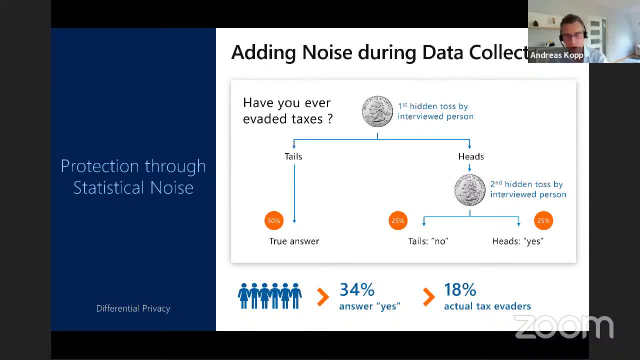 if we collect diagnostic data from the end-user devices, we apply random noise, differentially private noise- before the data is transmitted to Microsoft, then for analysis, And the same thing is true for Google and also for Apple end-user devices. So they are leveraging the same concept. 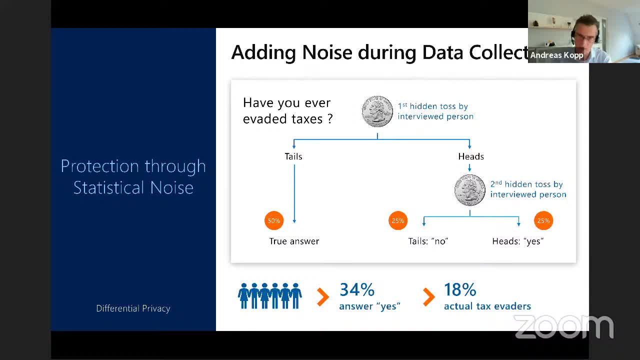 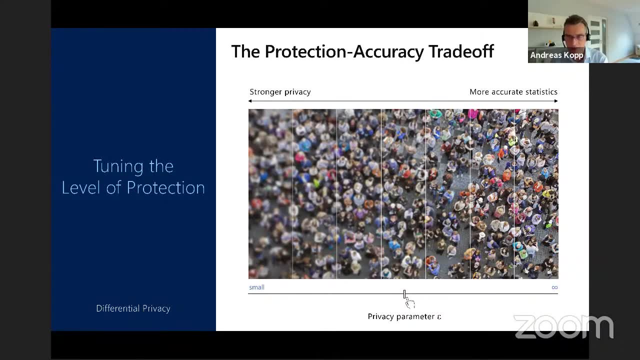 which is the local differential privacy model on the end-user devices. And yeah, as I mentioned, differential privacy is not a binary switch. So there is a very important tuning knob which is called privacy parameter, epsilon or privacy loss parameter, which you can use to work on this trade-off. 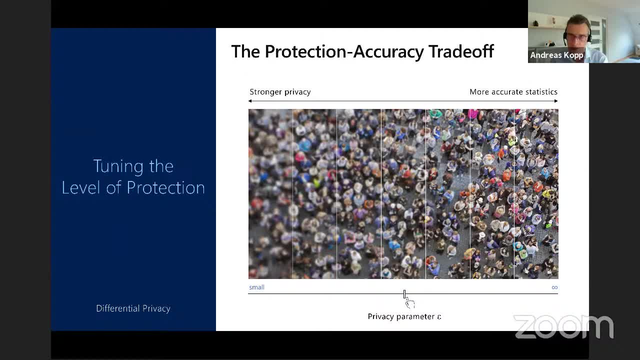 between the end-user devices and the end-user devices, So you can work between privacy protection. you can make it extremely strong and accuracy, And this is shown here in this picture. For example, if the epsilon value is extremely high, which means that the noise is relatively low, 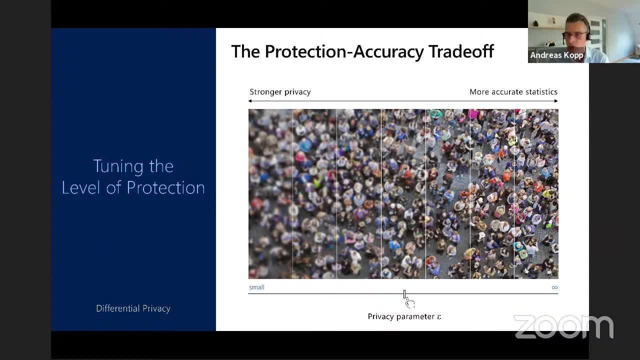 on the right-hand side you have maybe the original picture, So it's very clear. You can still identify people. If I move the privacy parameter to the center, then the picture becomes. it's a little bit blurry, so maybe I can still recognize the gender. 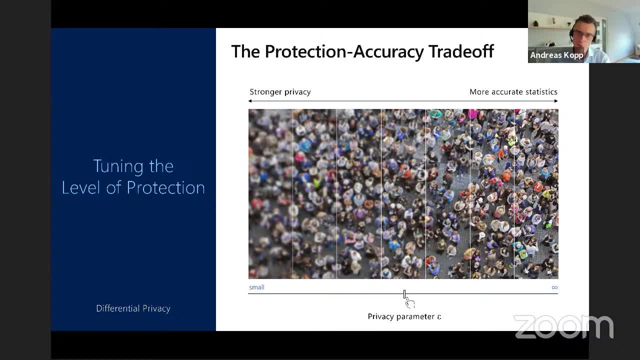 but it's obviously not as clear as the original picture. And I move to the far left. then it maybe becomes hard to even count people. So we are always operating on a trade-off between accuracy and the privacy guarantee. if you are using differential privacy. 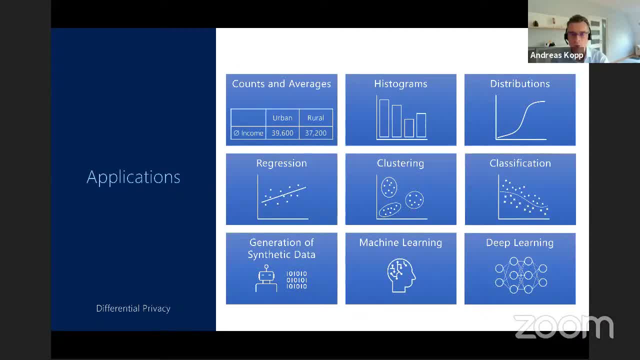 And, yeah, differential privacy supports a broad spectrum and that's why we have this particular example. that's very interesting. So we have a combination of applications which is also included in our talk here. So we show a couple of, let's say, 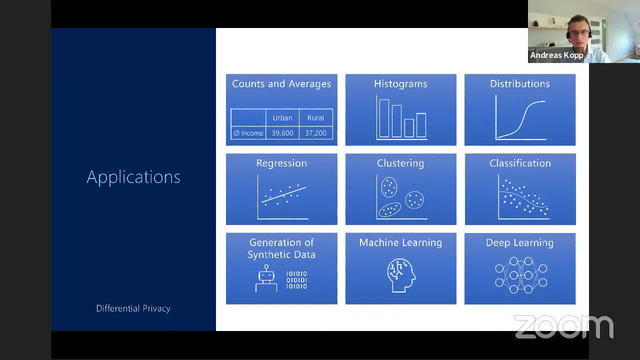 classical statistical examples like simple counts, averages, histograms, looking at distributions. Then you have more complex applications like multivariate analysis, like regression, clustering, classification. Another interesting use case about that is really to generate the generation of synthetic data. 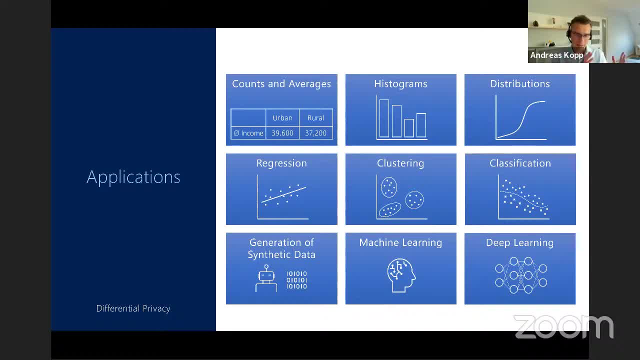 So you can look at an original data set and leverage differential privacy to create a new synthetic version of the data set which satisfied differential privacy, which you then hand out to the community and guarantee that the privacy of the individuals represented in the original data set is preserved. 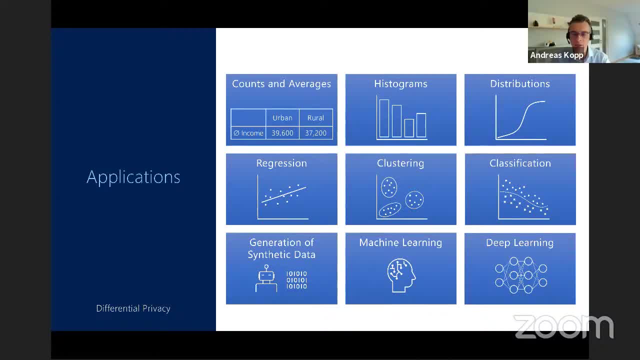 And you can also- and we will show demos on that- leverage differential privacy for machine learning, let's say for classical machine learning use cases like random forest logistic regression and these kinds of things, but you can also apply it to deep learning. 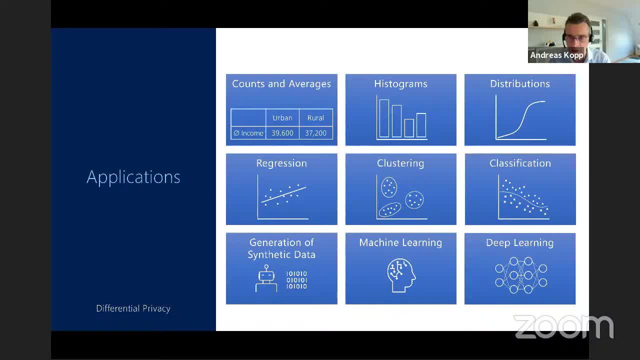 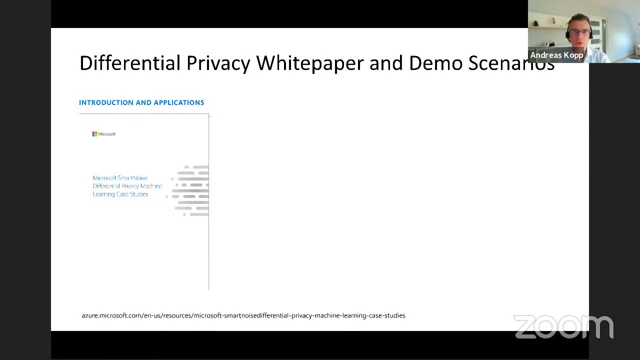 So all major deep learning frameworks like TensorFlow and PyTorch also have additions for differential privacy And we will show examples with PyTorch for medical images in this webinar And the problem with differential privacy, at least from my perspective as not being a scientist. 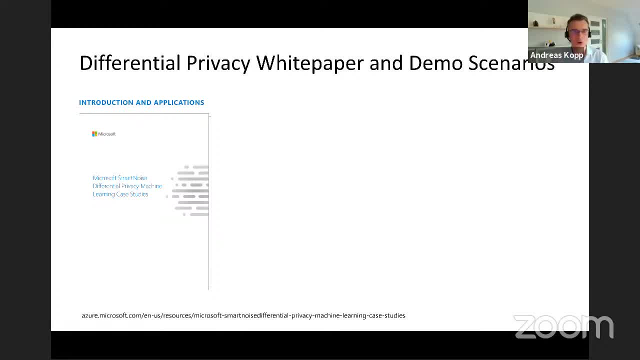 being more a practitioner is that there is a lot of. there's a really strong scientific foundation, a lot of research papers, but for, let's say, data scientists or machine learning practitioners, it's not so easy to understand The concept And what we did, with the help of Lucas and other folks. 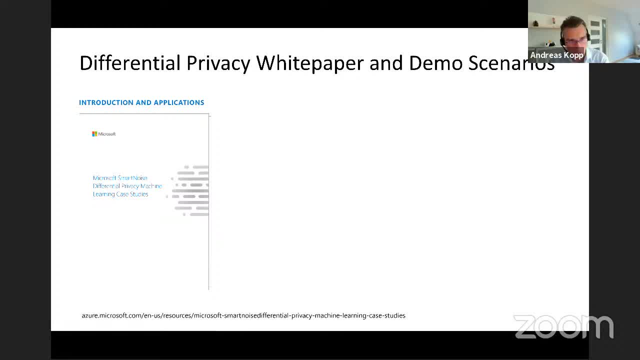 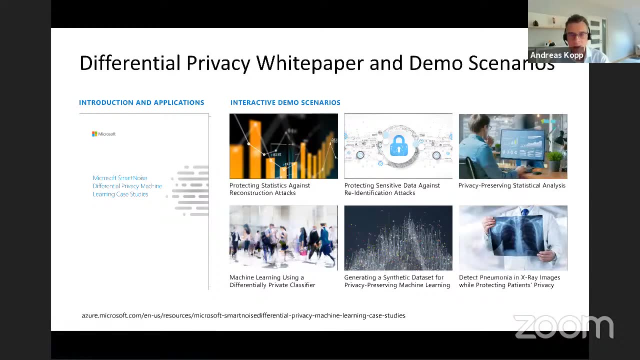 is really to come up with a white paper, quite comprehensive white paper which is focused on for practitioners really to understand the concept, to make it very tangible, very practical, And it also includes six demo notebooks which you can use. They are all public. 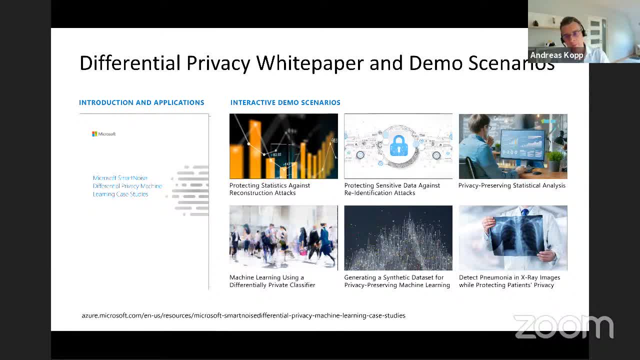 And we will show a couple of them in this webinar really to better understand the concept, to play with the concept and also apply them to your own use cases. And what we are going to show in this webinar is how differential privacy can be used to protect. 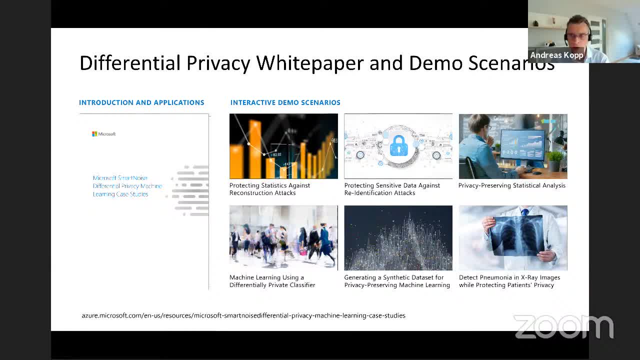 against re-identification attacks. We also look at the impact on various epsilon values and the number of data points. We will also take a look at doing machine learning with a synthetic data set And the final demo will be a deep learning scenario to detecting pneumonia and X-ray images. 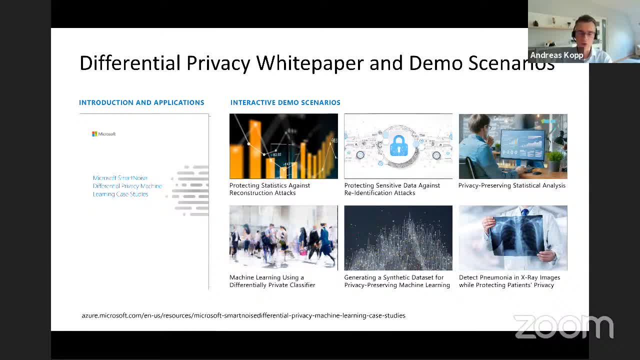 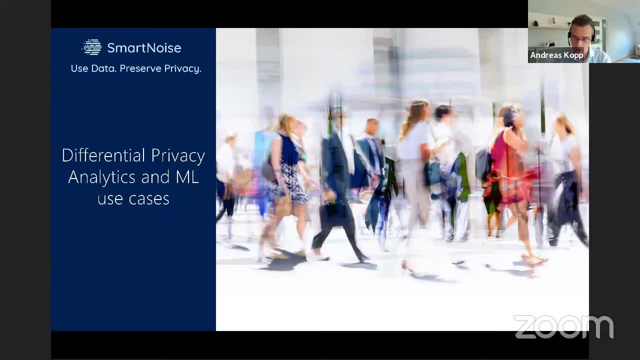 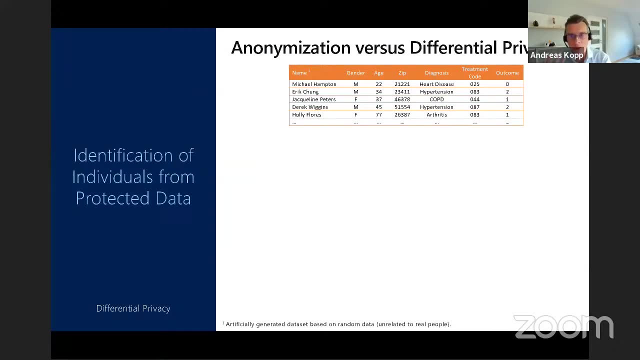 comparing the non-private and the differential private version. And that brings me to my first demo. So now we are moving to the differential privacy. So let's take a look at the differential privacy, analytics and machine learning use cases really to understand. on the one hand, 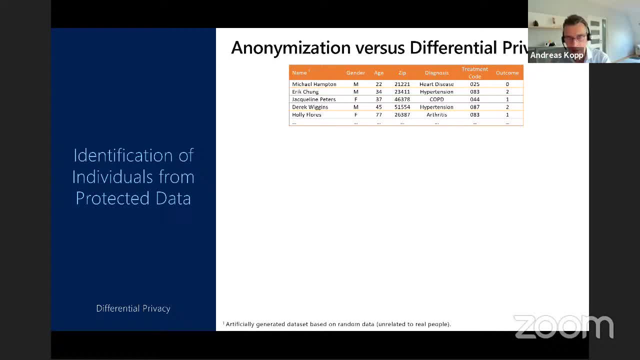 the risk of a classical privacy protection methods like anonymization and to compare that with differential privacy. So let's assume we are hospital representatives, So we have a lot of patient data and we want to provide this data to a research institution to benefit medical research. 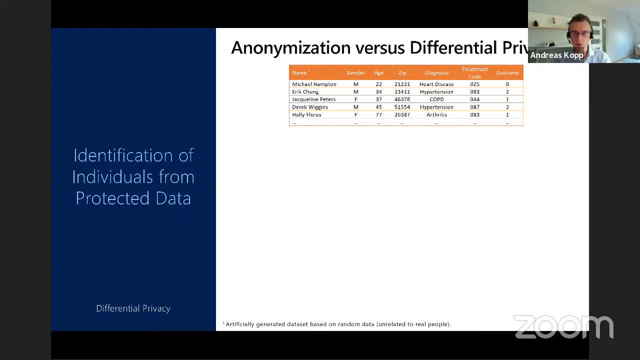 So, and we have information, of course, as the hospital representatives. we have the full data set. We have the names of the patients, We have basic demographic information, but also the extremely sensitive information like diagnosis, the treatments that we did and also the medical outcome. 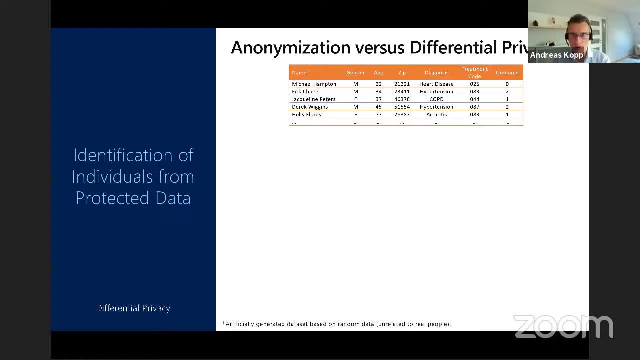 So what we did in this demo? we generated 30,000 records, of course, all synthetic, random data, so no real data about real people, of course, And what we compare in this demo is data anonymization. So we deduct information, we Vault the data. 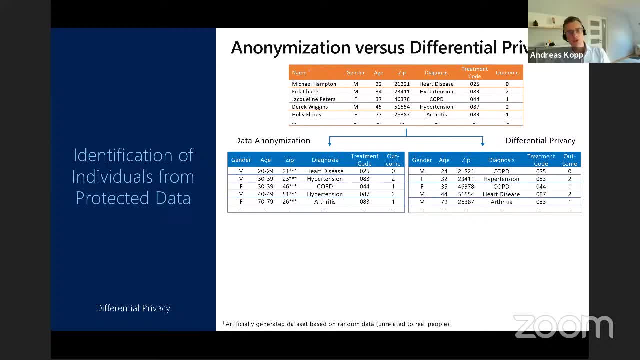 So we remove the names. for example, we draw names, So ages are only shown in decades, and we take away three digits of the zip code. We also ensure that for each demographic combination of attributes at least three records exist. So this data anonymization satisfies. 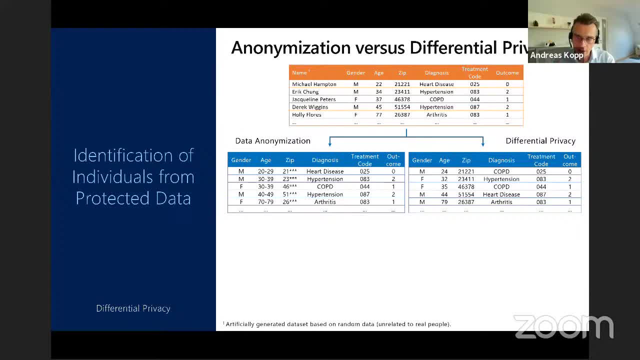 K of 3 anonymization And, on the other hand, we generate a new data set based on the original data set, which satisfies differential privacy using the smart noise product, And Lukas is going to show a little bit more background how this works. 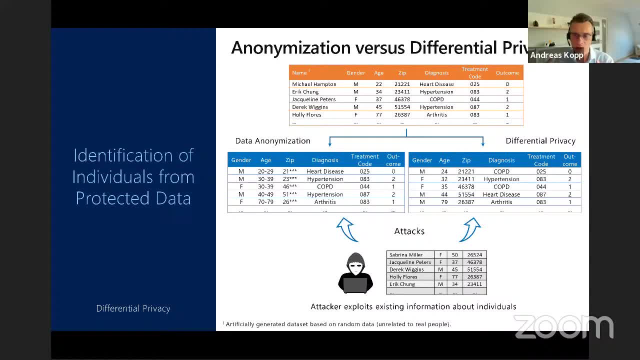 And for comparison, on the other hand, we have an adversary. We have an attacker who has some information, some very basic information like phone book information. So he has a real large data set about names, age, gender and also zip codes. 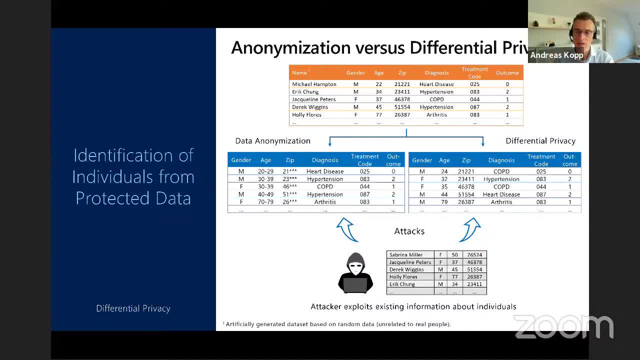 This is really a toy example And in the real world, attackers would be able to leverage much more information, And it becomes really critical if they are able to combine various data sets to do much more sophisticated attacks, based on triangulation, for example. 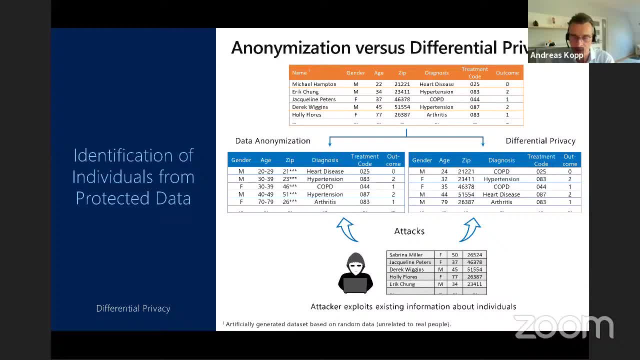 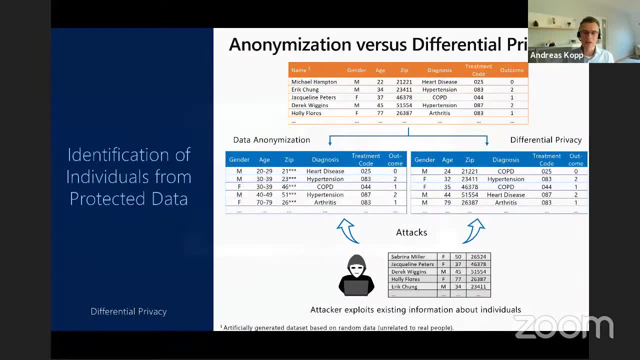 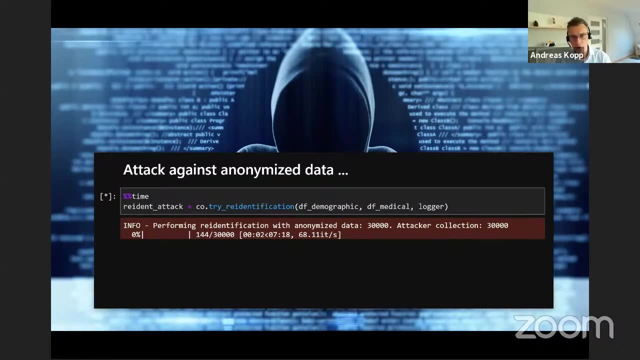 So what you see here is really- it's a toy example, but already disturbing. So maybe a small spoiler. And what we are doing in the notebook- I'm showing it here because it takes roughly 10 minutes in the notebook- is we try to combine the attacker's data. 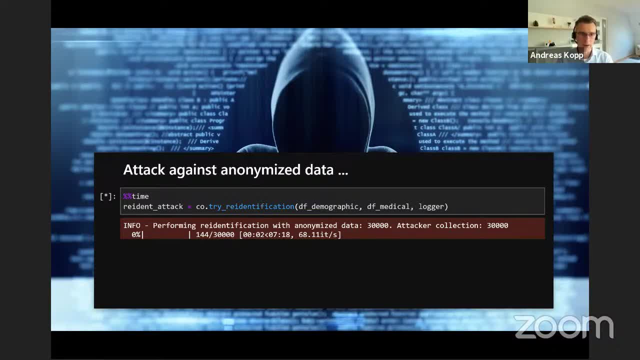 set with the data set which is protected by anonymization. So it's two phases. One is simply to match the information And then we do a second pass. We have included a specific UID to be able to really find out how many, how many records could really be identified. 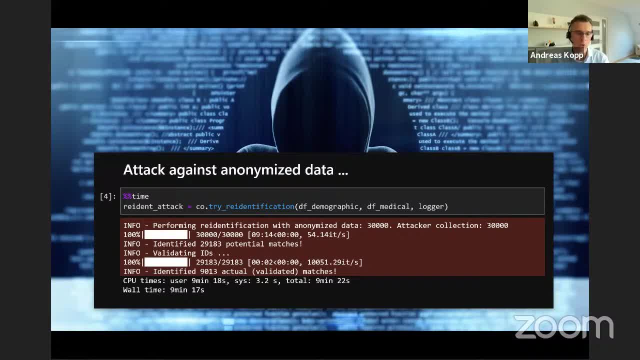 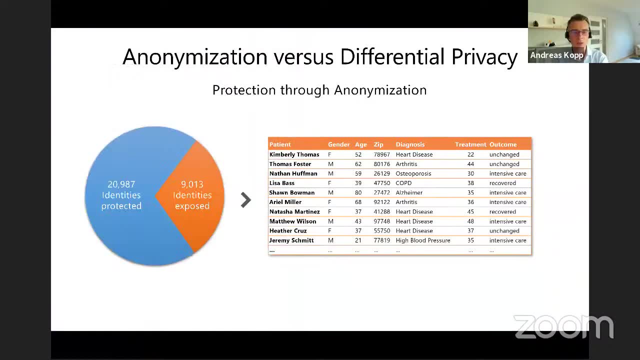 So to be able to exclude false positives in this example, And what we can see here is that that's the result. So we were able to re-identify almost a third of all identities based on anonymization, And that's kind of to expect based on this K of 3. 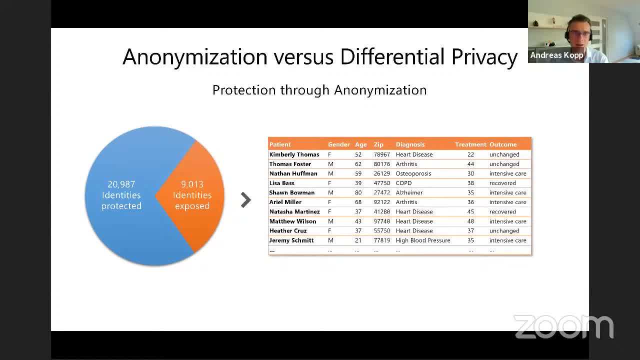 anonymization that we have used And you can see here What we were able to re-identify. Just a couple of examples. as I mentioned, all random data, So no real people represented here, of course, But I think this really shows the problem of current data. 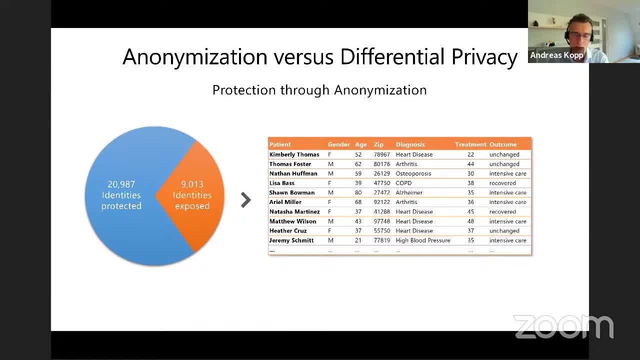 anonymization strategies. You can argue: yeah, in a real case we would not use three anonymization, We would maybe use 10 anonymization. That's all fine. But on the other hand, real world attackers would be also able to leverage much more sophisticated 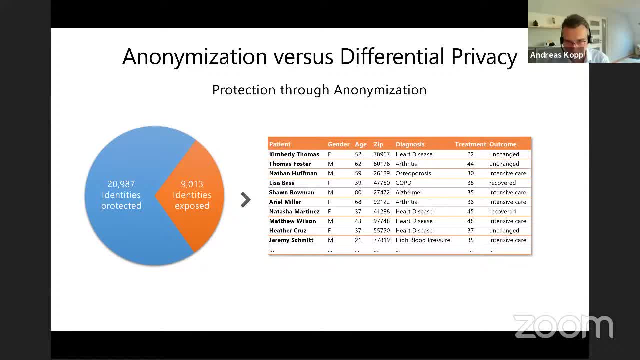 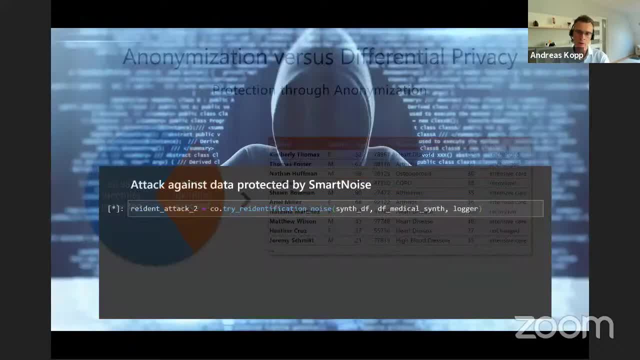 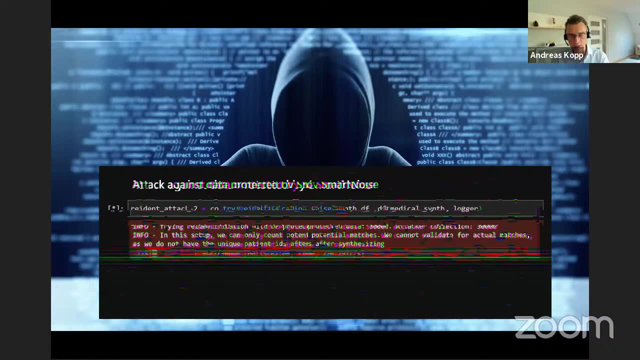 sophisticated algorithms and much more additional data which they can link. So this is a real problem, which is shown only already by this toy example. And what we are doing, on the other hand, for comparison, is we leverage smart noise to generate a new data. 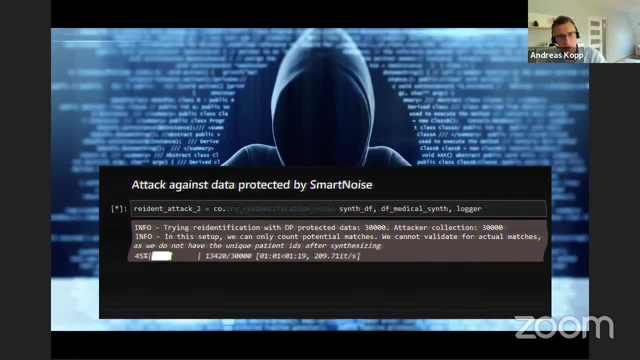 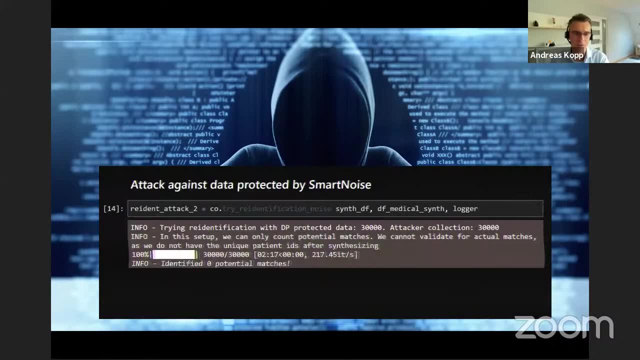 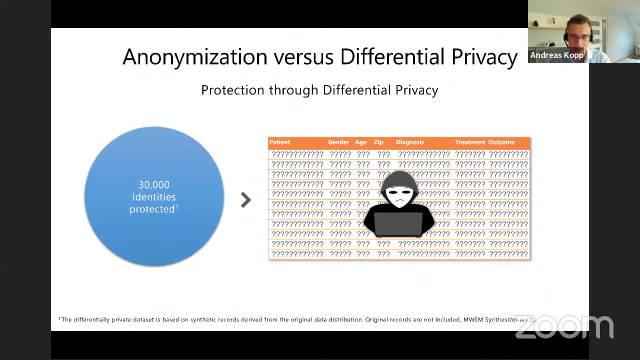 set based on the original data set, which has the same statistical properties as the original data set, And since there is not much to see here, we spiced up the animation a little bit And the result is then here. So in this particular example, we 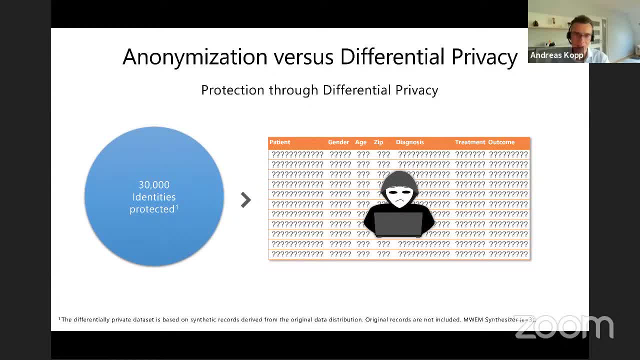 were able to protect all identities, So not a single identity could be re-identified by this attack, which shows the differential privacy provides a strong protection mechanism here for those who are interested, But we are using a specific synthesizer, the MBM synthesizer. 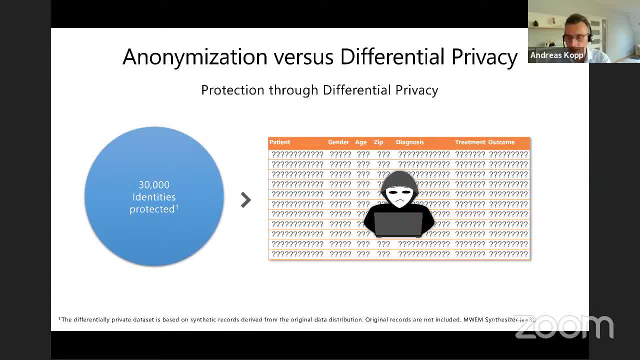 Maybe Lukas has some time to discuss it. in his part about the synthesizers, We used an epsilon of three, which is a common starting point for practical use cases. Of course, the question you might ask is: well, that's nice. 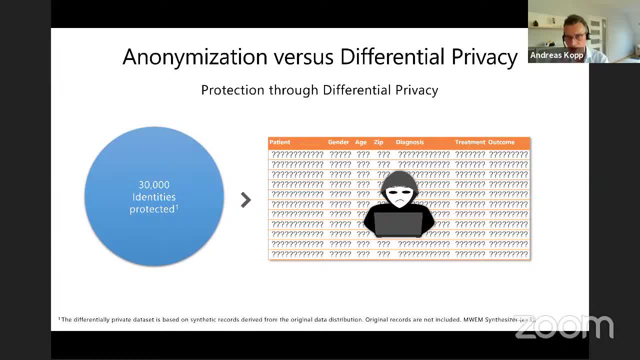 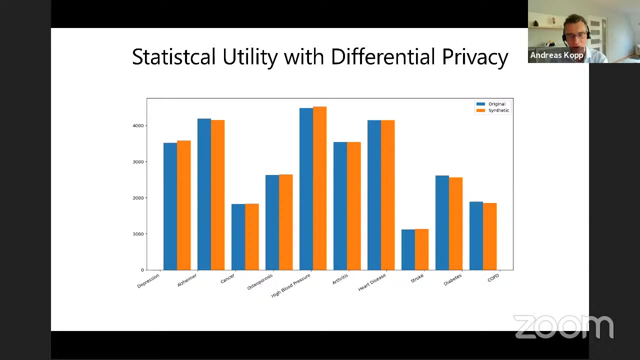 We've masked the contribution of the individual, So we added noise to the data. Fine, But has the data still utility for statistical analysis? At the end of the day, we want to see the big picture, We want to do analysis, And what we are seeing here is a very simple univariate use case. 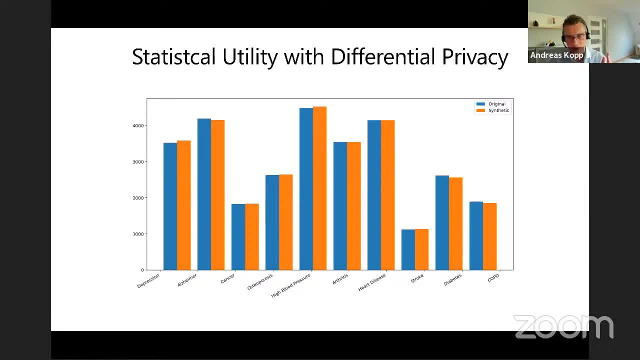 So what we compare is the distribution of the diagnostic code, So the left one, the blue one is the original And the orange one is the same distribution, So the same feature based on the synthetic data set And what you can see here. there are some differences. 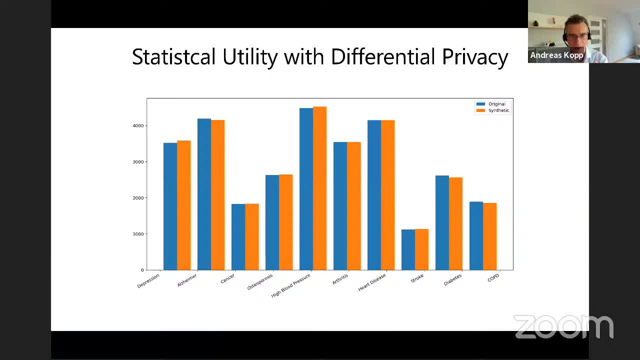 in the histogram, But it's quite consistent. So there is still utility in the data. You can still use it for statistical analysis. But the question is well, what is the use case And what is the use case And what is the use case? 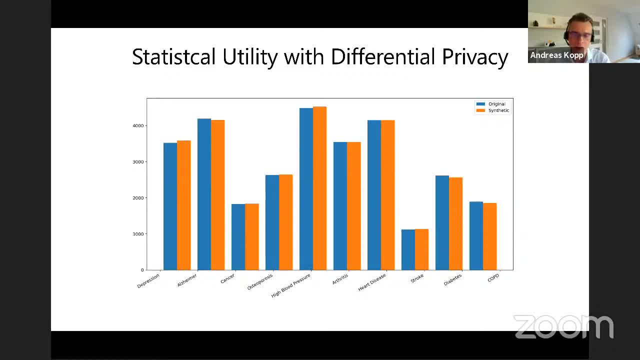 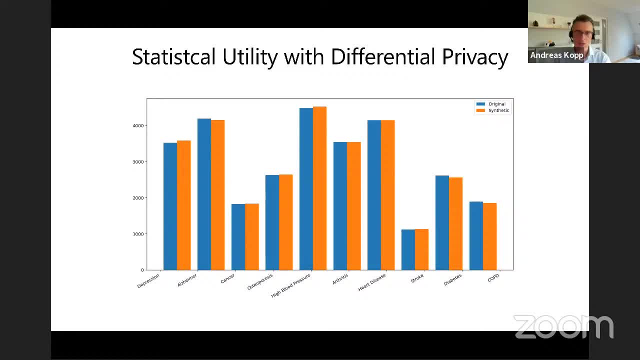 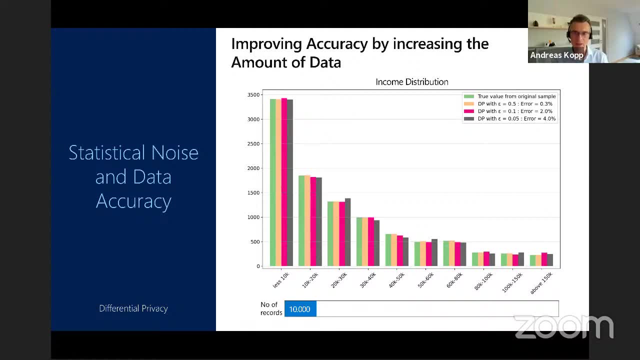 introduced by the noise. we have a separate notebook. So what we are doing here is we also compare distributions at various data set sizes based on the California income distribution data set, And we compare the original value from the original sample with differential private histograms at three different 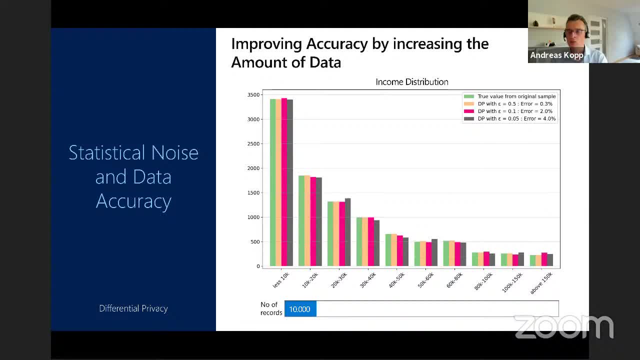 protection levels. So the yellow one uses an epsilon of 0.5,, the reddish one uses 0.1, and the dark one uses 0.05, which is an extremely high level of protection for practical use cases. And here what you can see is based on an overall data set of 10,000 records. so the error 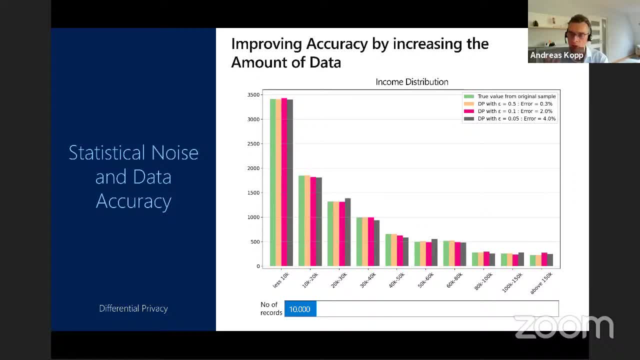 the percentage deviation goes, depending on the level of protection, from 0.3 up to 4.. And you can also spot, especially for the dark bars, that there are some deviations which you can see, And then if we go to 50k records, things look a little bit different. 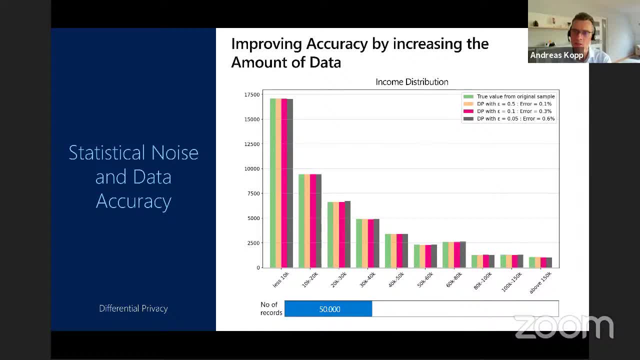 So even in the case of the strongest protection, the deviation is below 1%, And if we increase the data even further, then it's hard to spot differences between the bars, And the error, even in the most aggressive scenario, is 0.3%. 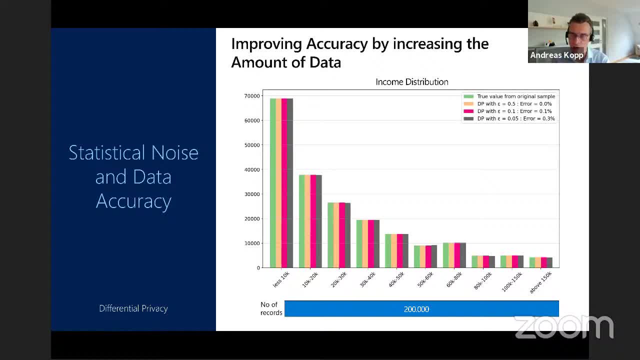 So that's a general observation for all use cases. You can compensate for the loss and utility that you get by the introduction of noise by adding more data. That's a common observation also for other use cases, also for machine learning and also for deep learning. 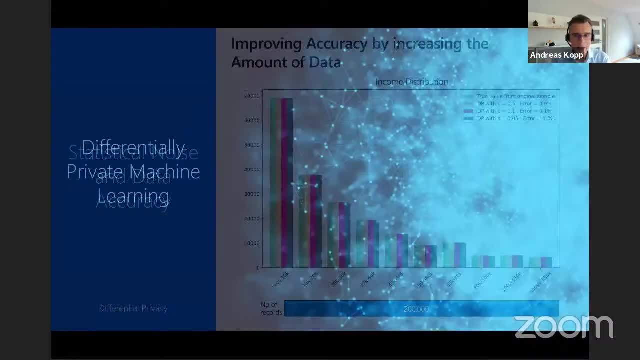 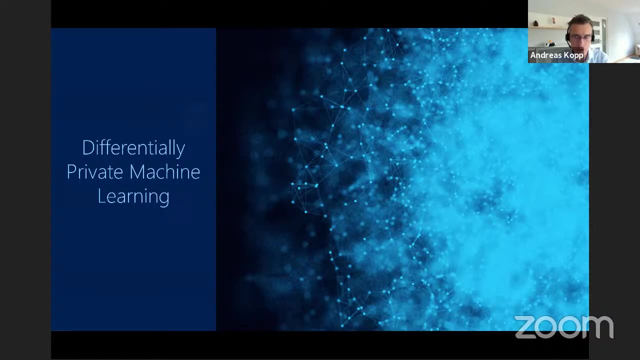 which is an important property. So maybe now moving to machine learning use cases, differentially private machine learning use cases. So we are always interested if we are doing machine learning, also besides the privacy discussion. we do not want to that our machine learning models memorize data points. 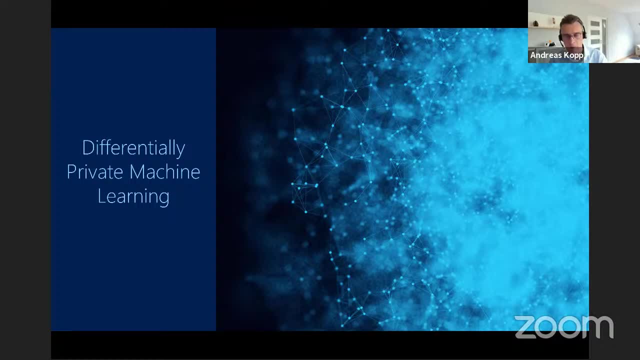 So we want to learn the general thing, the general pattern. But, as you all know, all or many machine learning models have a tendency to overfit, to memorize specific data points, In particular deep learning. that also happens if you are controlling for overfitting. 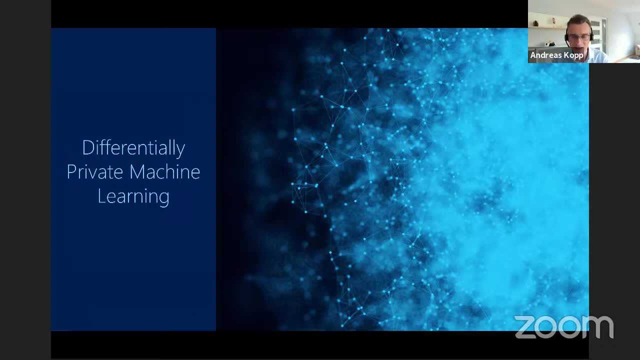 So there's always the tendency to memorize data points, especially very specific data points, And the risk, of course, is that this enables a set of attacks. One is called membership inference attack, so that you're able to find out if a specific individual is represented in the data set. 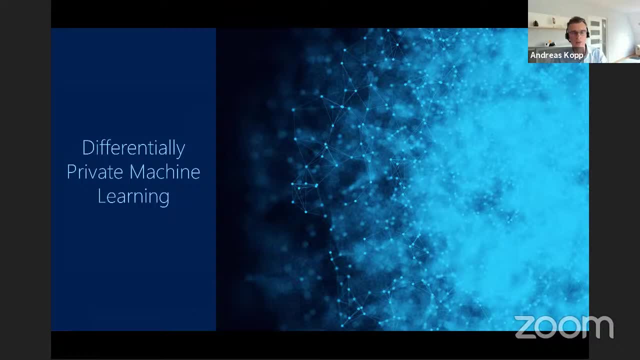 or not, And this alone could be a privacy issue. For example, let's assume we have a medical study about Alzheimer's disease. If you can find out that the specific person is part of the data set, you can with certainty conclude that this person suffers from Alzheimer's. 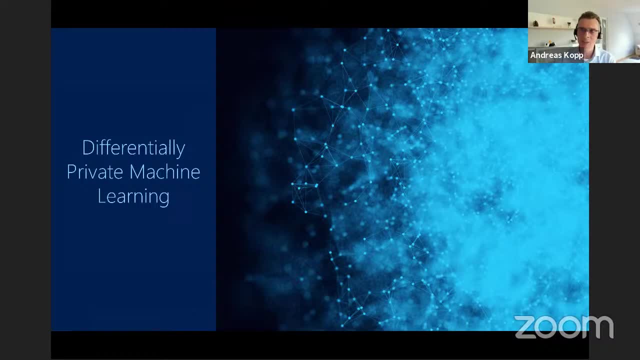 So this is called membership inference attack And given this large neural networks that we are using- think about GPT-3, with this 175 billion parameters- that's a real problem. And that happens also if you are able to control for overfitting, because this tendency to memorize data points always exists. 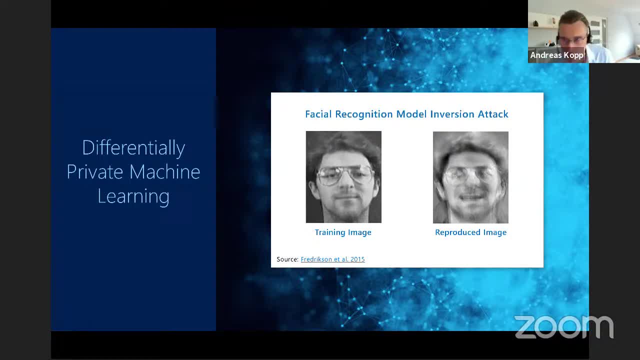 And there's another risk which is called model inversion attack. So it's actually possible- that's also the result of research, of a research study- to reproduce a recognisable image of an classifier. So that's a facial recognition model. so that's not any kind of generative model, it's really, it's a classifier. 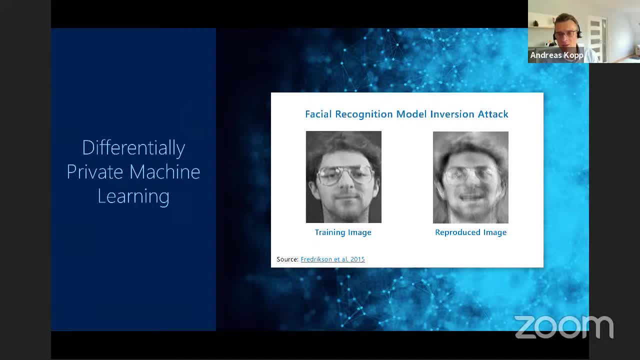 And researchers were able to reproduce, let's say, at least recognisable image of the training data based on this classifier, on this facial recognition model. So this is why differential privacy in, let's say, classical machine learning, but also, in particular, in the behavioral is the most important part of the data set. So there's a lot of Mexico. So this is the question that we have to answer. So this is why differential privacy in, let's say, classical machine learning, but also, in particular, in the behavioral 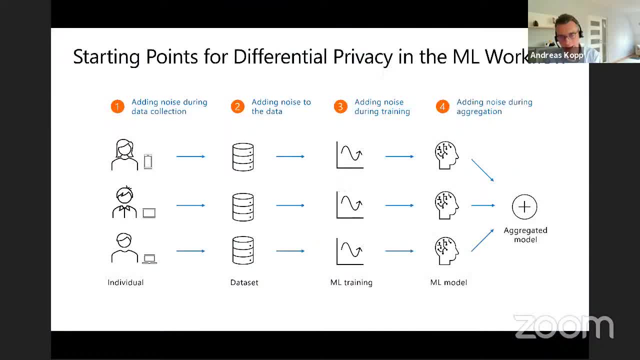 particular in deep learning, makes a lot of sense, And the question, then, is: how can we apply differential privacy with machine learning, And there are various steps within the machine learning workflow that we can use, And these are four options. Of course, these are alternative. 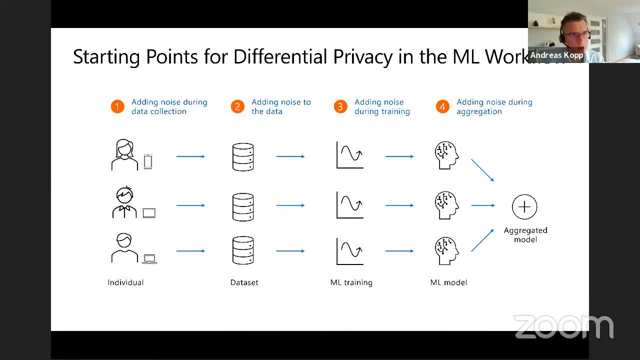 options. So one would be, which is called the local differential privacy model, is to add noise during data collection. This is the Windows 10 example of local differential privacy that I gave. So the local device acquires data about you or about your behavior, or about the device itself. 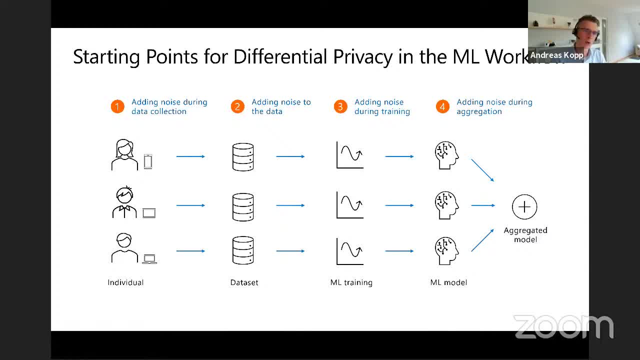 like in the Windows 10 diagnostic data, Locally adds noise to the data and then transmits the noisy data to Microsoft or to Google or to Apple for further analysis. So that's one option. Of course, from a privacy point of view that's. 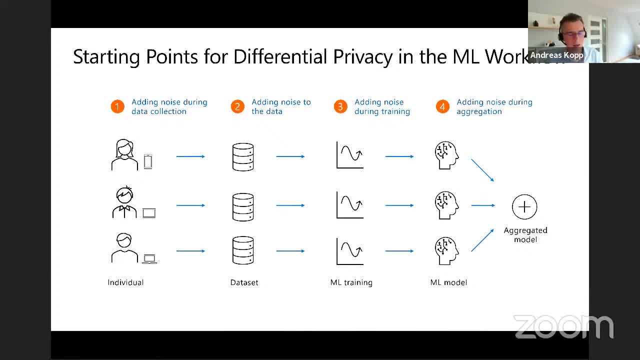 the preferred option, because nobody but the affected individual ever sees the unprotected data. Then there is a second option, which Lucas is going to talk about, Which is that you basically you have a data set and you reproduce a differential private version of this data set And then you are feeding this into your machine learning workflow as training and test data, for example. 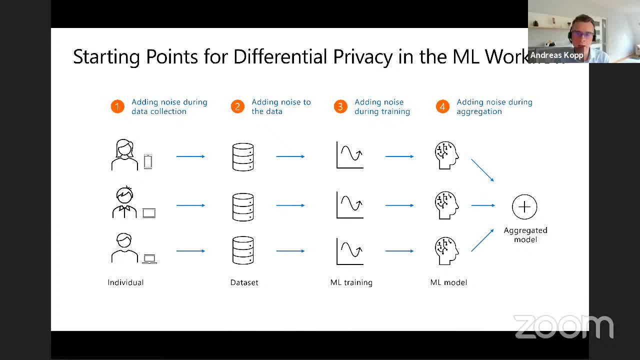 The third option would be to leverage a differential privacy enabled algorithm. So, for example, there are are for the classic machine learning algorithms like logistic regression or Naive Bayes. There are differential private versions from IBM. so from the IBM DiffPRIP library. 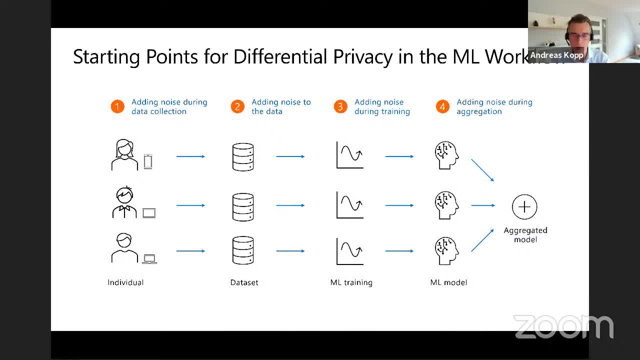 And also for deep learning use cases. both TensorFlow and also PyTorch have differential privacy enabled. with stochastic gradient descent algorithms, learning algorithms, That's also possible. And then another option would be to combine differential privacy with federated learning, So you do your differential privacy locally. 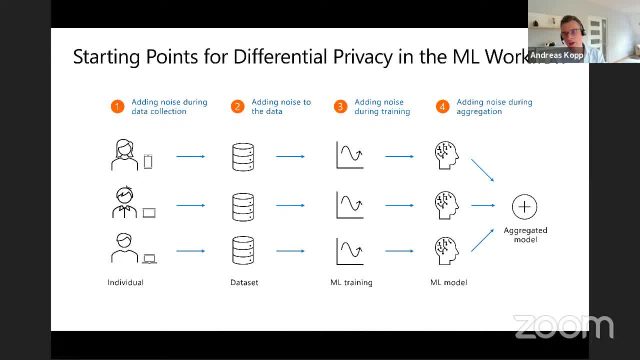 do your training locally and then you just use the aggregated parameters or the local parameters to aggregate it to your machine learning model, And the basic could also be differential privacy way of data collection. So there are a couple of options. In particular, federated learning is typically. 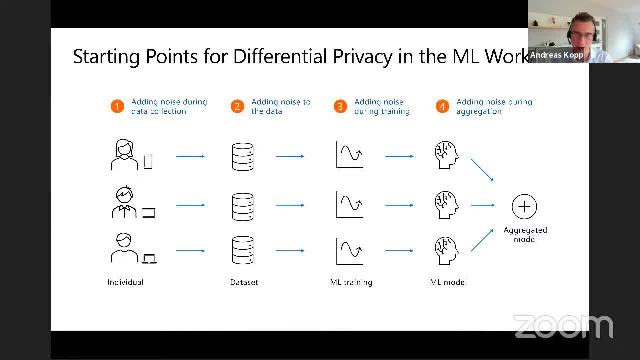 or often combined with differential privacy, So they address different concerns or different use cases. So it's quite common in medical use cases, or quite a trend, to combine these technologies. So a couple of options and Lukas is going to show a demo and also comparing a particular option two. 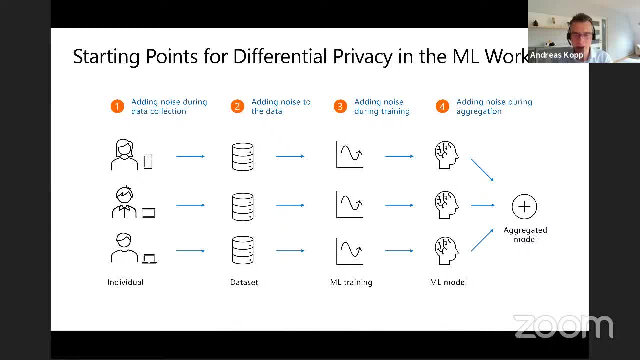 with option number three, And with that I would like to hand it over to Lukas to explain the background of synthetic data sets, sorry, and also to show the demo. Thank you so much, Andreas. Quick question. Do you think we should answer some of the questions? 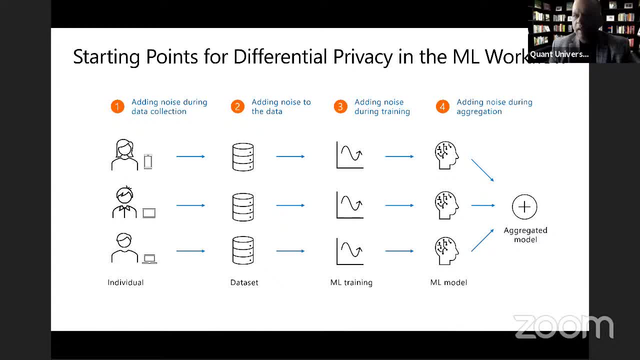 we've been seeing in the chat window before Lukas starts his demo. I think we had a couple of questions, but I actually had a question For all the four steps. do we have sample templates or anything? Andreas, I know Lukas is going to share two of them. 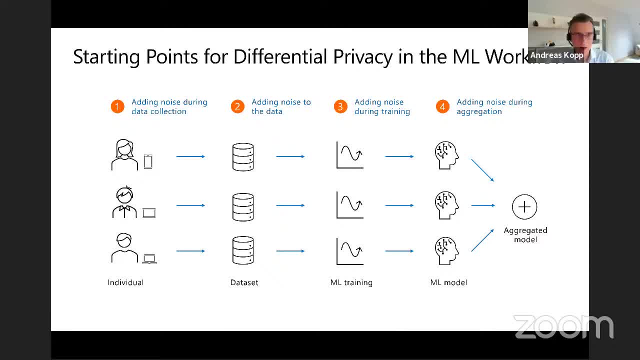 but the other two. do you have templates? We have templates for two and three. Two and three, okay, So not one and four, Okay, okay, good, And I think, Lukas, you were able to answer some of the questions. 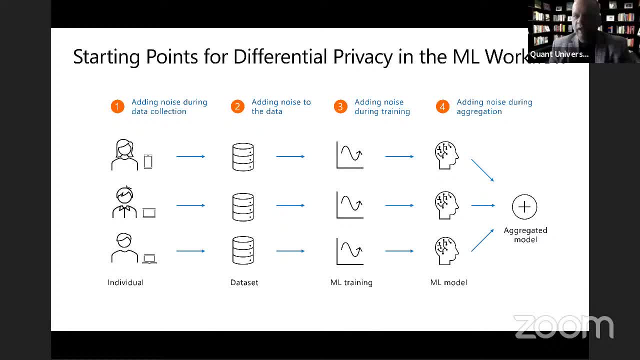 Yeah, I think I got through a couple of them. Do you want to go through them? or I mean, like I don't know how many people were watching the chat window. Are there any questions we can answer? Yeah, let me just briefly touch on. 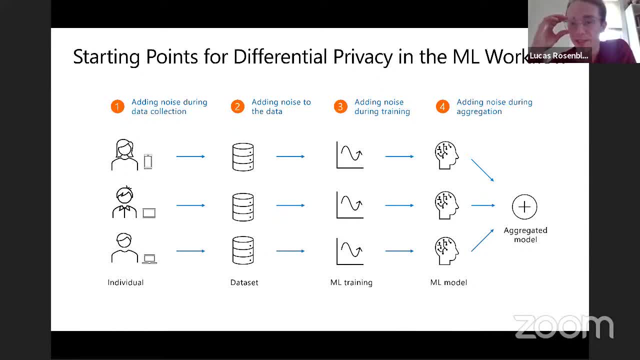 so one of the questions is related to how do you decide on the appropriate value of epsilon. That's a great question. It's almost an open research question. essentially, There are certainly scenarios where you need to ensure a specific level of privacy based on a specific attack you're defending against. 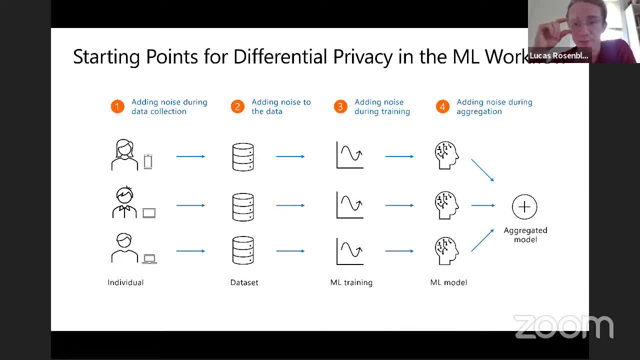 And so you can simply tune your epsilon based on the attack, But generally there is not an agreed upon way for deciding on the appropriate value, So obviously this is not an appropriate level of epsilon. However, there are some values, like Andres was saying, like three: one 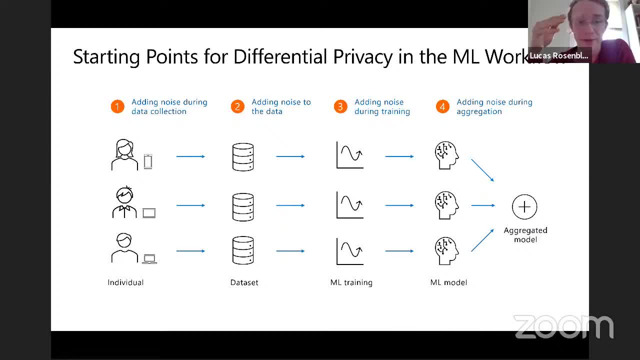 or values below one that are agreed upon in literature. Certainly values above that start to get a little dicey. So you don't usually see values more than 50 or 100 in literature in their tests and from there you start to lose. 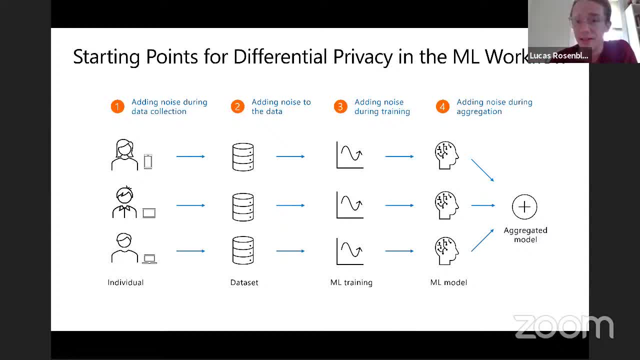 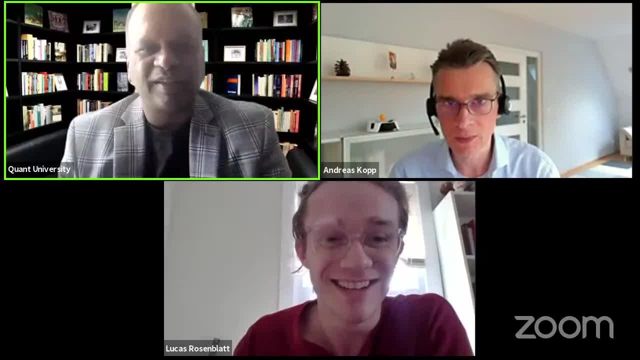 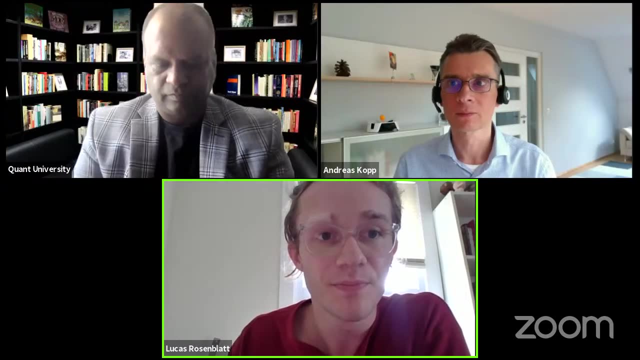 any of the privacy benefits? Yeah, And then maybe I can just start on my part of the presentation and we can get to some of these other questions a little later. Yeah, this is very engaging, Thank you. Yeah, So I'm just going to go ahead and share my screen. 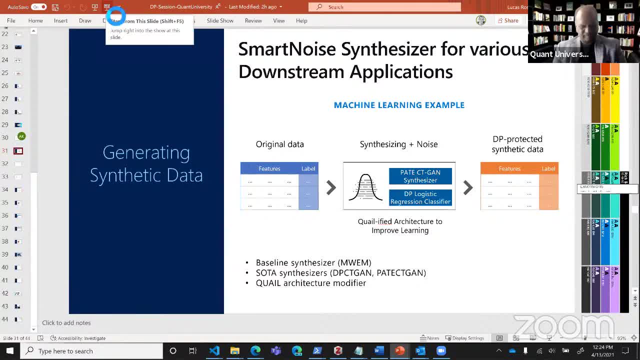 Thanks again, Andreas. That was a very excellent overview. Thank you, I'll just present with the presentation mode off. Okay, so thanks again, Andreas, for all that information. I'm just going to examine one of the downstream applications for Differentially Private. 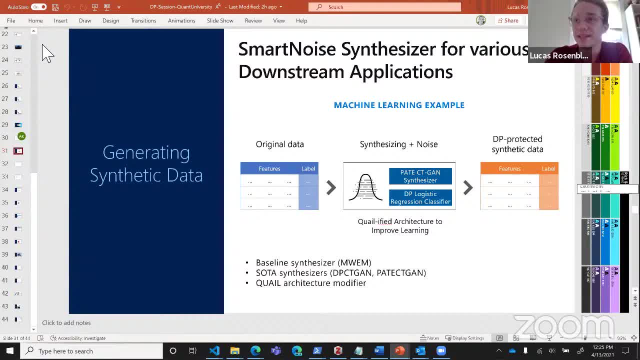 Synthesizers, specifically, That is, to generate a synthetic data set For model training. So synthetic data generation, as a broad overview, involves taking the original data set and training a synthesizer and using the synthesizer to produce sort of as much synthetic data. 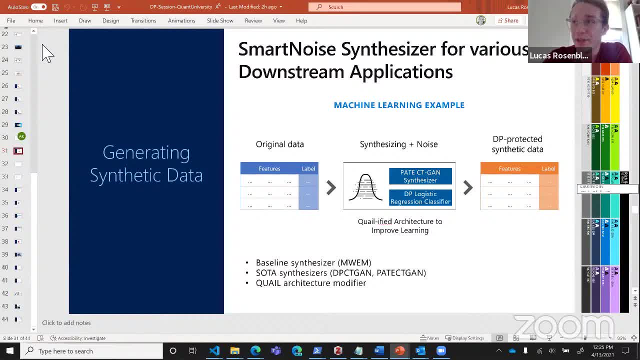 as is required to train the model. And these synthesizers can take many forms. So there's like histogram-based methods like MWEM, which Andreas mentioned before, And there are also generative adversarial network methods like DPCM, Like DPCTGAN. 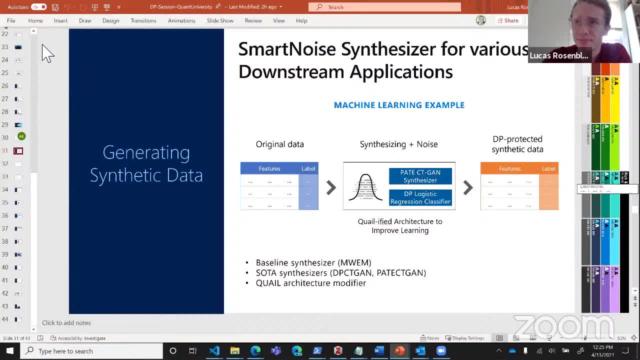 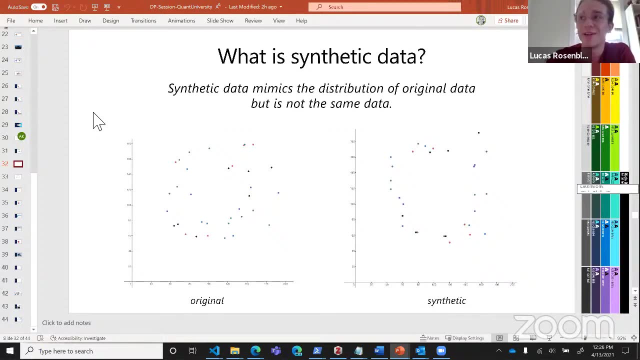 Or Paid CTGAN, which we have up on Smart Noise, And I'll just refer to these as GANs. So that's sort of a broad overview, And now that I've brought up synthetic data, just make sure everybody's on the same page. 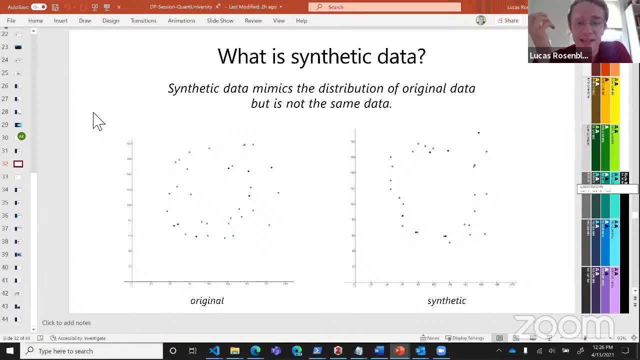 But simply it's, you know, taking some original data set and creating a new data set that mimics the distribution of the original data set. So you can see an example of that here. If our original data set on the left synthetic data set on the right, you can see that the 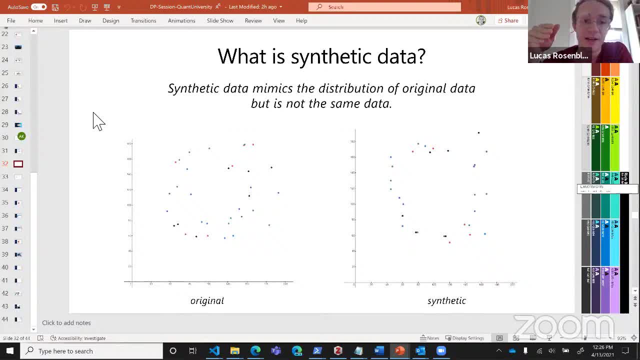 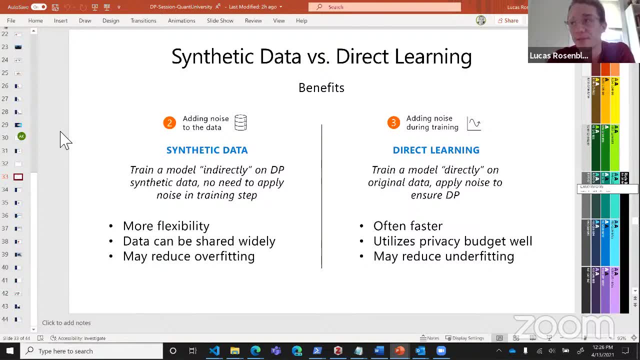 general distribution with some variation is mimicked. Okay, So using differentially private synthetic data when training models has some added benefits when compared to what I'll call direct learning, where that's just training a differentially private model on the original data. So when you use a synthetic data set that is differentially private, you can sort of 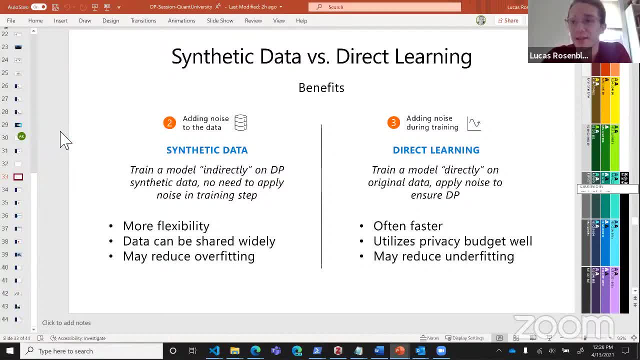 train whatever model you want on the data. perform your hypergrammer tuning safely, share the model and the data widely. There's even some evidence that this process can create a more robust model, so it could reduce overfitting, Whereas direct learning, where you actually apply the noise directly during model training. 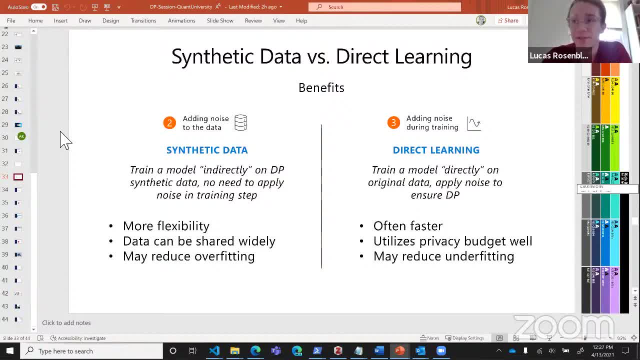 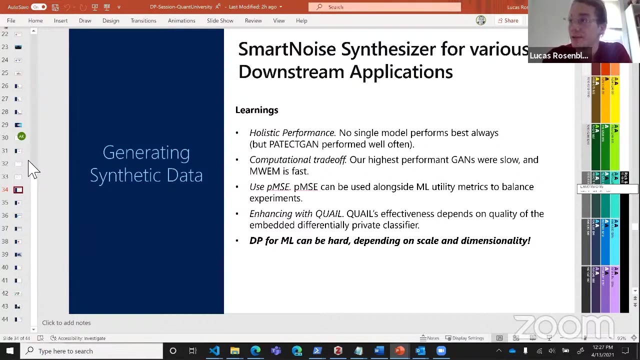 is often faster and utilizes the privacy budget well. However, once you've sort of trained your model, it's one shot, And so you can't really do hypergrammer tuning without reducing your privacy guarantees. Yeah, So I'm going to bring up this paper that I wrote with some collaborators here at Microsoft. 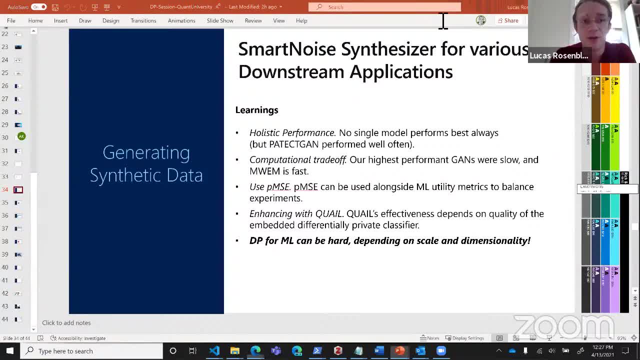 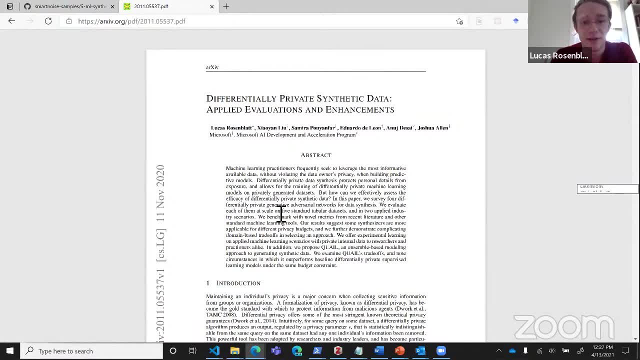 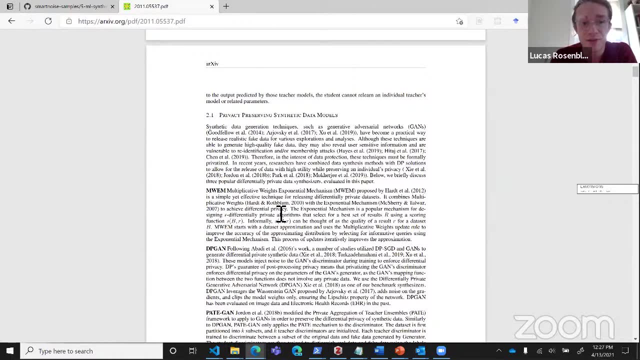 Let me bring it across here. So we took a look at differentially private synthetic data, state-of-the-art methods. We did some evaluations so you can totally check this out if you're interested. It's a broad overview on the mechanisms that actually ensure differential privacy as well. 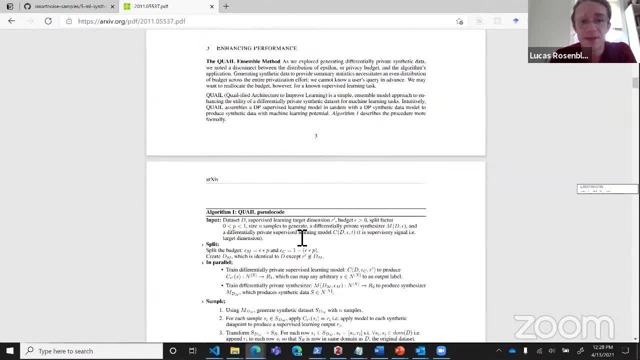 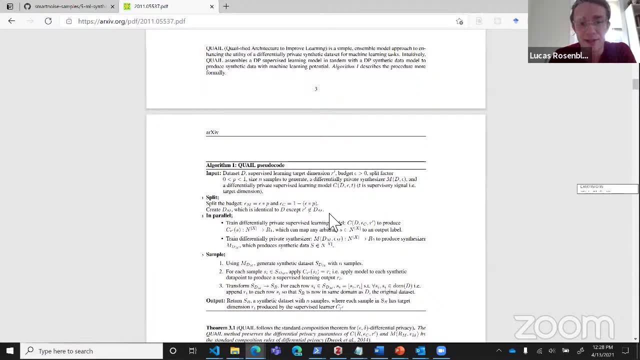 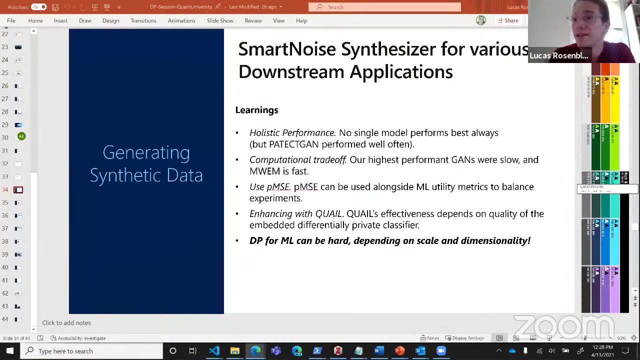 as the way you integrate them with synthetic data methods. We also presented our own method called QUAIL, which helps with generating synthetic data that is specifically for model training. So yeah, if you're interested, check that out. We'll share the link. 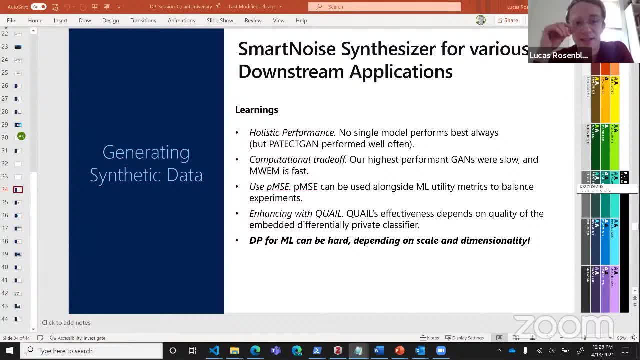 And I've abbreviated some of the learnings from the paper on this slide. So some of the things we learned is that, as is often the case, there was no single data synthesizer that always performed best, although some outperformed others in aggregate. 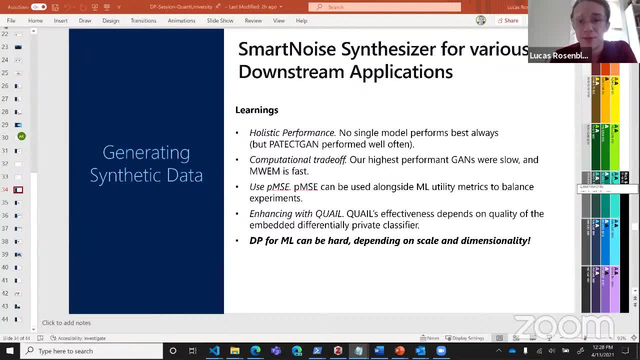 And the GANs were pretty slow to train, While some of the histogram-based methods, like MWAM, were pretty fast. We also discussed some metrics that you can use to assess the quality of your differentially private synthetic data, because it can be quite tricky to do so. 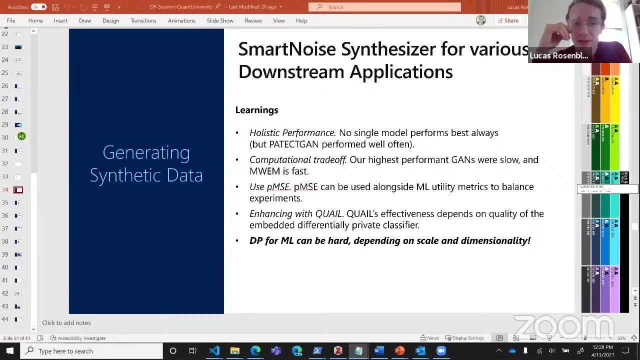 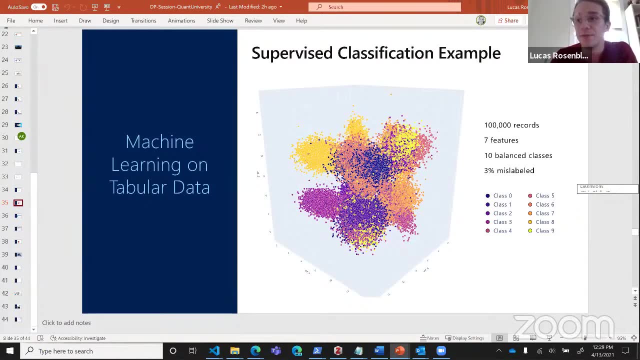 And we present on some of the learnings with QUAIL which can really help with the specific scenario that I'm describing here. So let me briefly touch on this example That I'll show with part of my demo. So here's the original data set, which is sort of a fake data set. 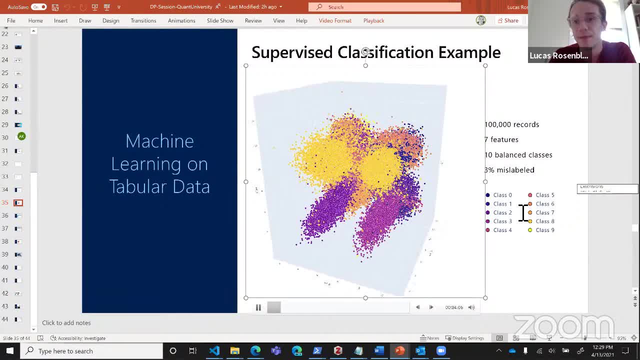 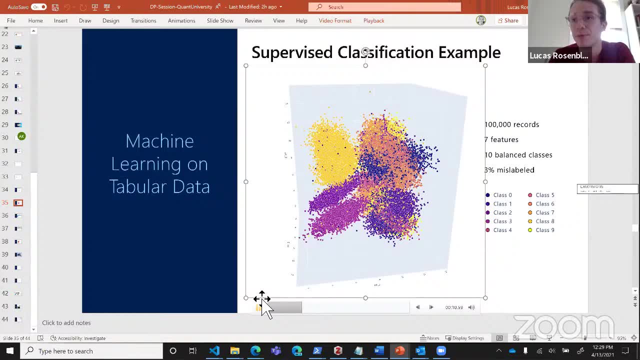 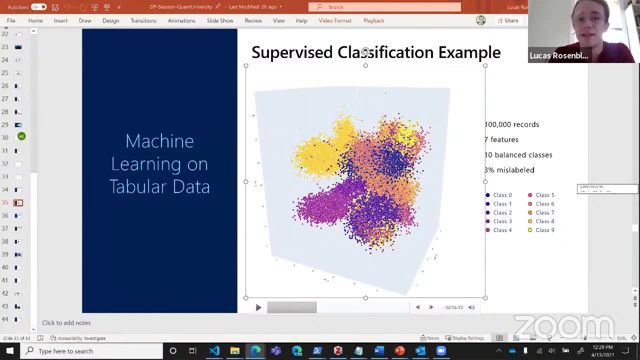 You can see it's actually quite a challenging classification. example: 100,000 records, 7 features, 10 balanced classification, and then there's some noise in there. So 3% of it is mislabeled. Great, And you can actually go online and take a look at the notebook yourself. 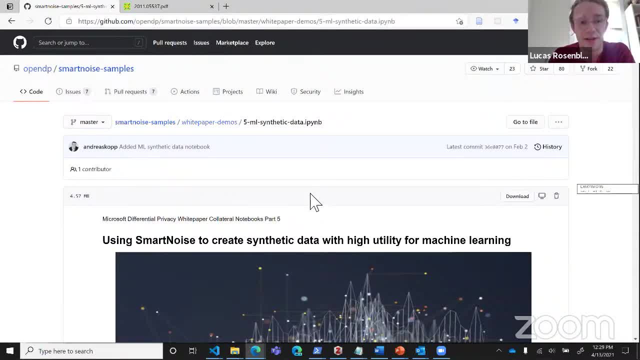 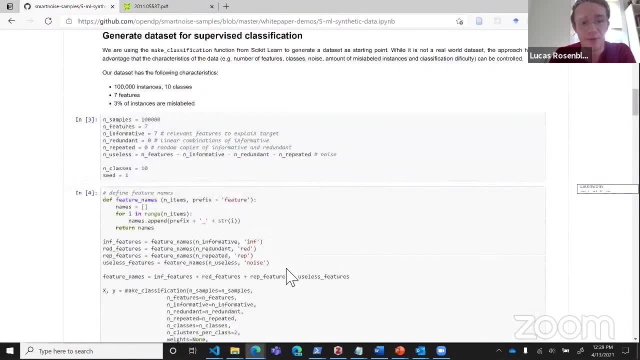 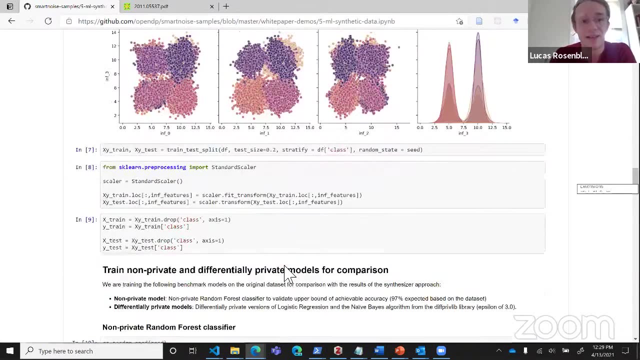 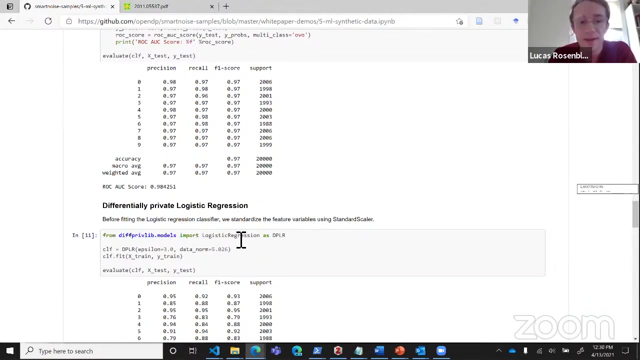 So Smart Noise GitHub, which we'll share out as a link. Here is the notebook where we actually do training and we show a few examples. We train on the original data set and show what just sort of no differential privacy does. So we get a score of 97,, you know, 97% accuracy. 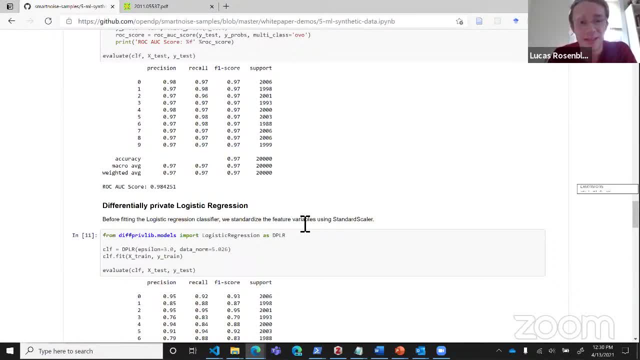 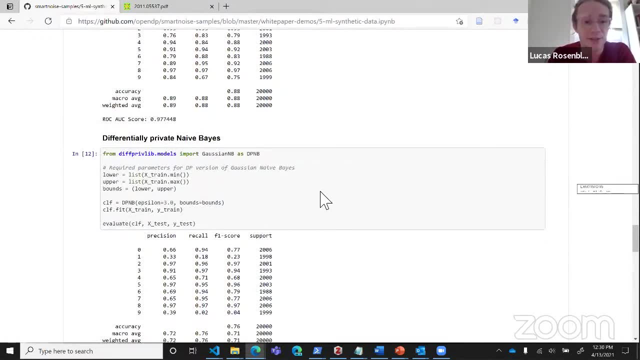 And that makes sense because 3% of the data points are mislabeled. And then we do differential private training using an IBM library actually, And we present the results there. So we see 89% accuracy and 72% accuracy. 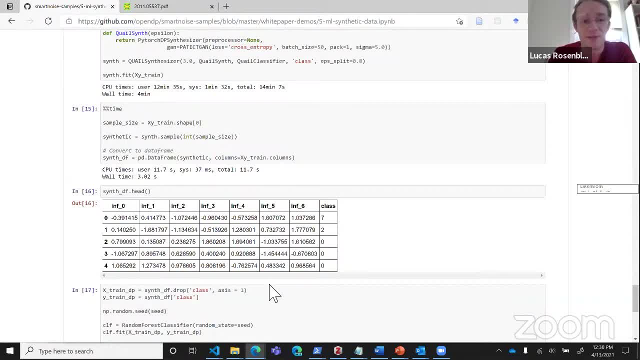 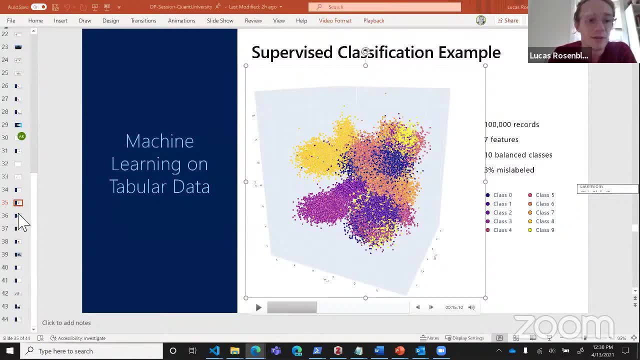 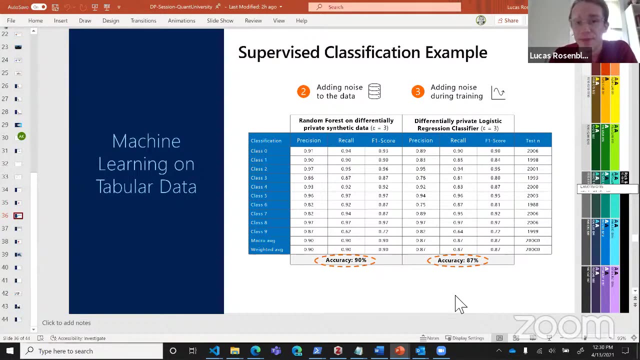 And then we generate a synthetic data set using some Smart Noise tools And we get an accuracy of 90%. Yeah, So just to put those numbers up on the slide So you can see, in this specific scenario, The synthetic data set with a random forest model trained on it, actually outperformed the direct learning. 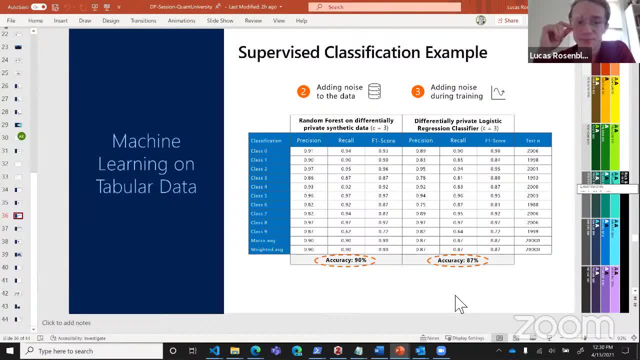 Differentially Private Logistic Progression classifier. So this is a scenario where you actually get a bit of a boost, where you may reduce overfitting by generating that Differentially Private Synthetic Set And then just taking whatever model you want- in this case random forest model and training on top of that. 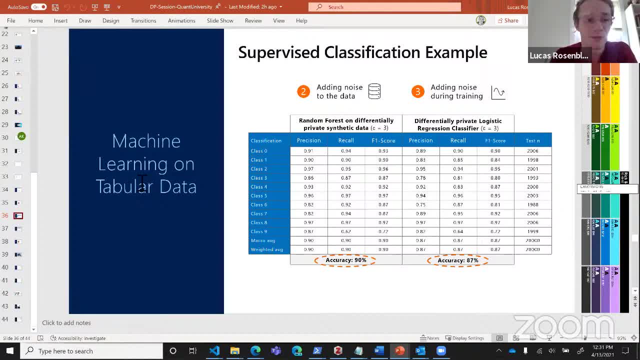 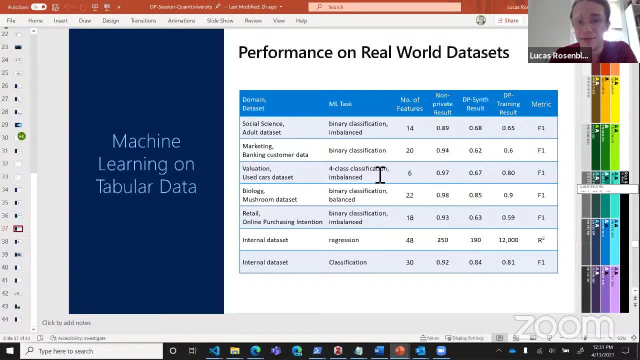 And you still have that differential privacy guarantee, Which is pretty cool. I also have in the paper a bunch of different benchmark results on, you know, your world data set, as well as a few internal Microsoft data sets that I can't say too much about. 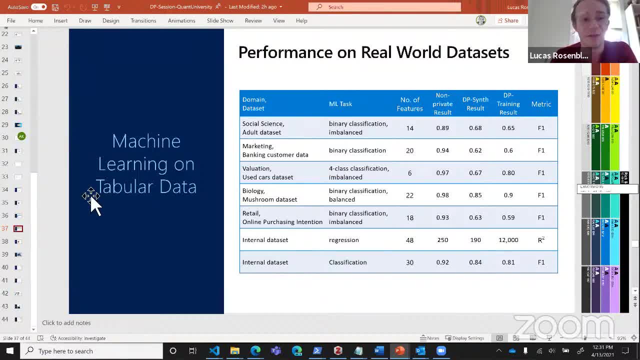 But we present the results there. So if you're interested in this, you can go look at the paper some more And with that I'll hand back to Andreas and see if I can answer some more of your questions, More of your questions in the chat. 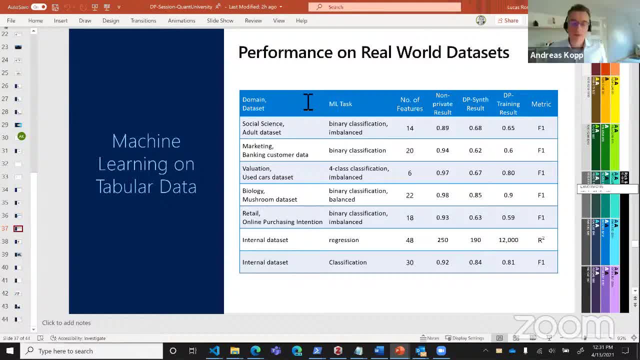 Andreas, do you want to take over again? Yeah, thank you so much, Lukas. there was one question: If we can share a little bit more about the math behind the research. I guess there is some level of detail already in the paper. 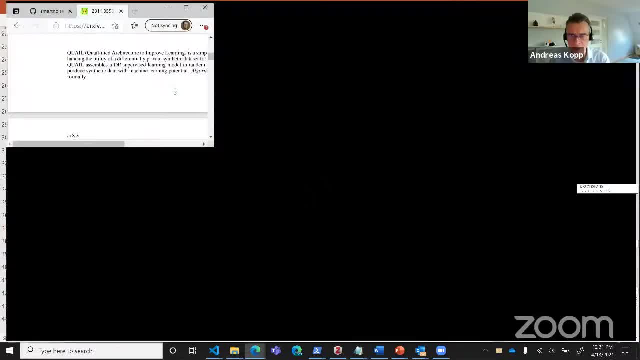 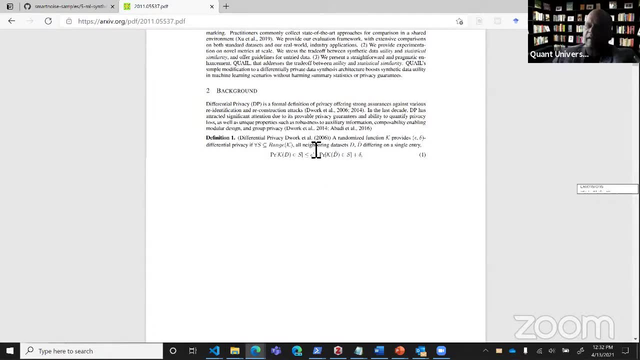 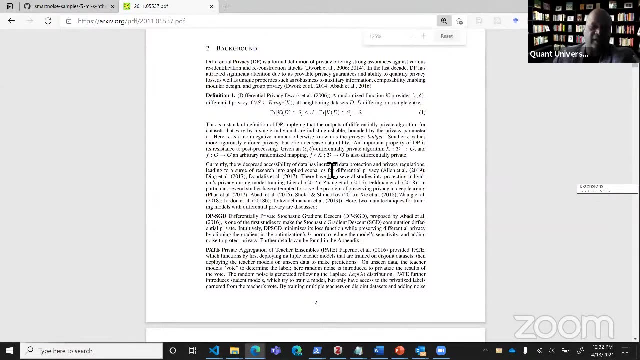 I'm not sure if you can. if there's any way to share more about the mathematical background, Yeah, let me just. I'll just pull up. I'm also interested to you know we have a fairly technical audience here. So if you want to go over your paper and maybe even talk about the other GAN techniques you reviewed, 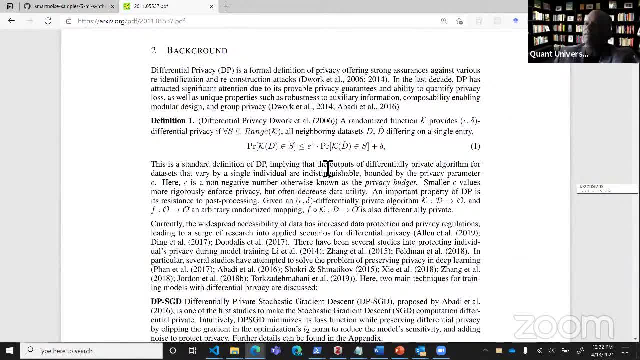 And also talk about QL. I would really appreciate that one too. Yeah, so I'll just do that. Yeah, please, Yeah, I'll do that, And then if people have questions after Andreas finishes up, we can dive more into it. 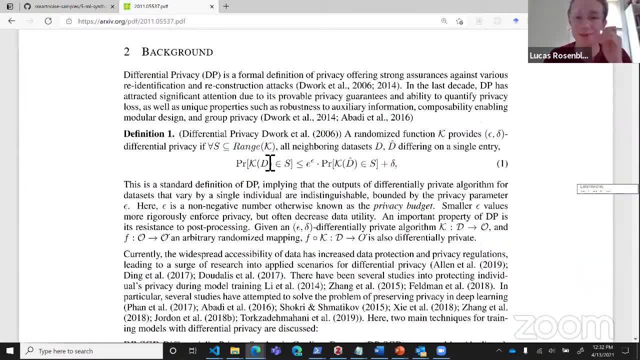 I figured you know it would be remiss if we didn't put up the definition of differential privacy at some point in the presentation. Here it is. Here's the formal definition, And whenever we're designing a differential private mechanism, right, we want for the mechanism itself to satisfy this inequality. 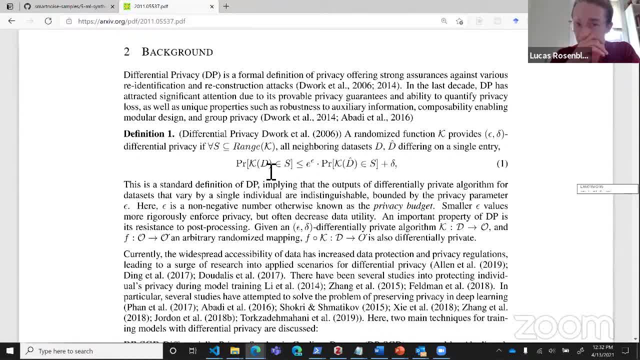 And so I won't go through. I'll answer questions on this equation. I'm not going to try and go through that because that would require, I think, a little more time than we have. But you can see here, this is our epsilon parameter that we tune. 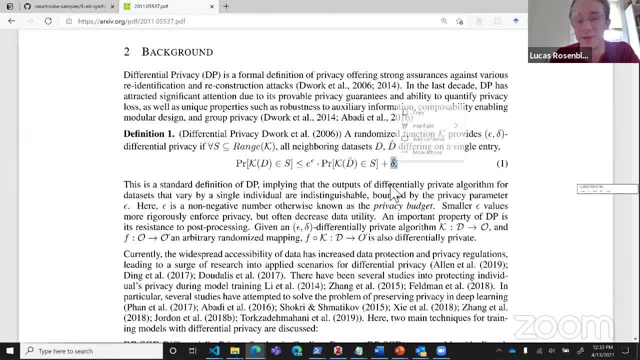 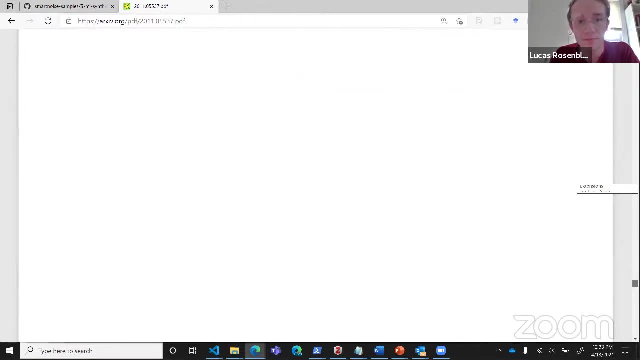 And this is actually what is known as the delta, That is, the delta parameter which provides a little bit of fudge factor, depending on your mechanism, where you can adjust the bounds for such that your proof satisfies this equation. And then let me just scroll through to some of the GAN architectures in the appendix. 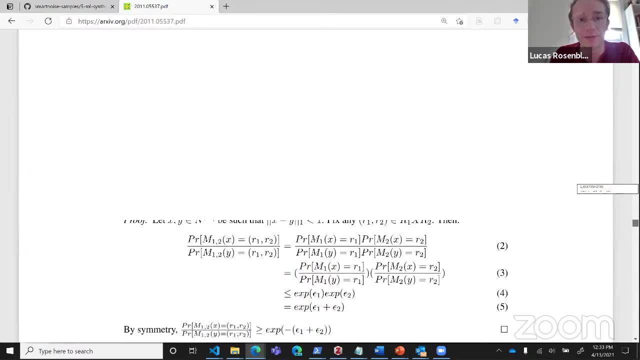 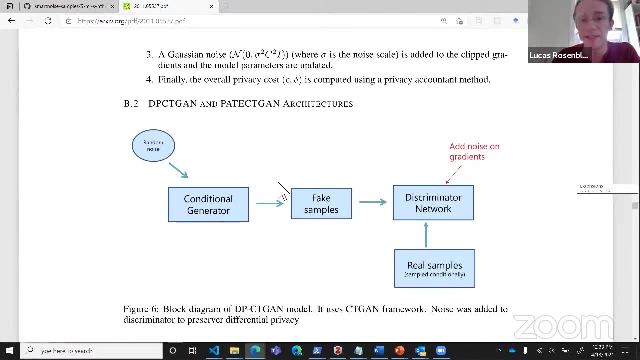 So here's a proof of Quayle's differential private guarantees. And then here's some of the GAN architectures. So the DPCT GAN model- that is on smart noise, actually adds the noise to ensure differential privacy in the discriminator network, And so it's, you know, a pretty traditional. it's actually the CT GAN architecture, if you're familiar with that. 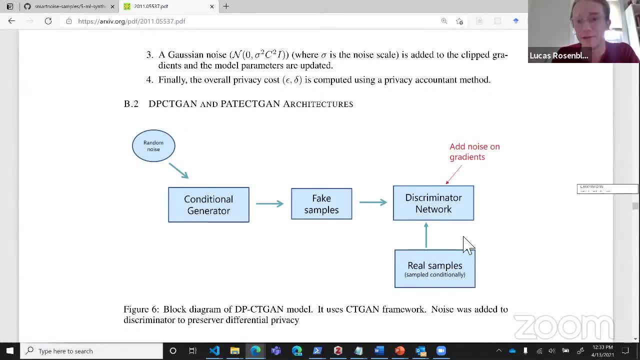 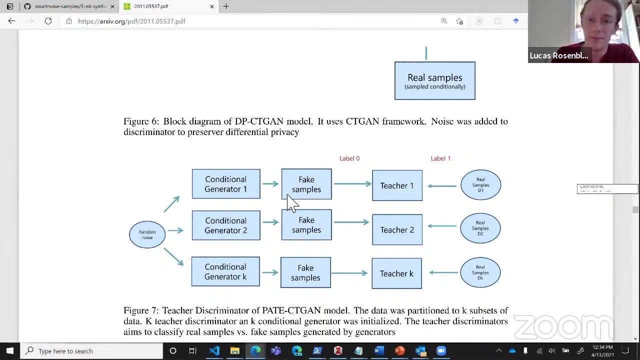 So pretty traditional GAN architecture but modified in the discriminator network, Using the Opacus language, Using the Opacus library to create differential private synthetic data, And then PATE GAN or the PATE CT GAN model relies on the teacher-student model, which is PATE. 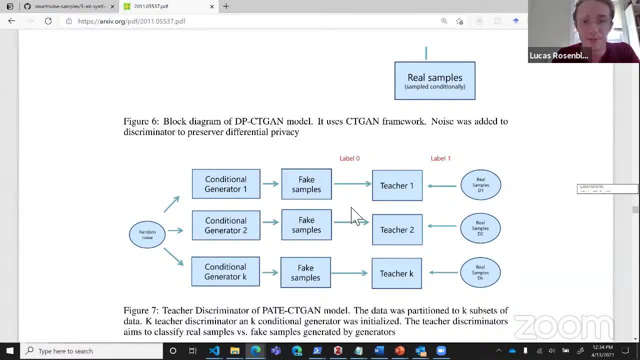 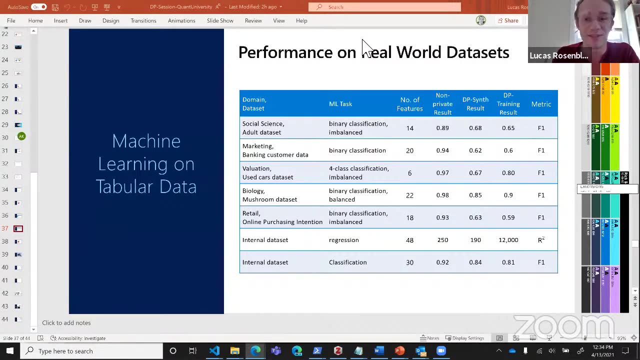 And I can talk a little bit more of that, although that might be outside of the scope of this presentation as well. So it's just a different mechanism, essentially for ensuring differential privacy in the synthetic data scenario. Okay, I am going to hand it back to Andreas so that we can finish up the presentation. 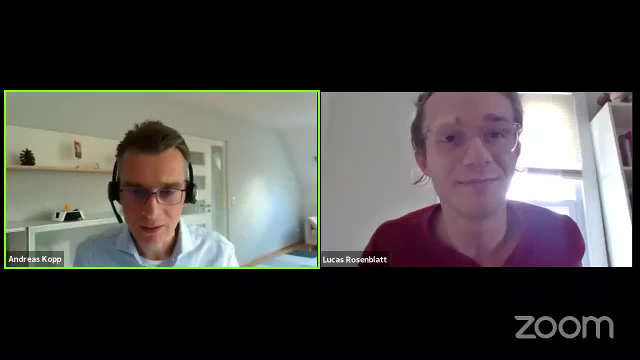 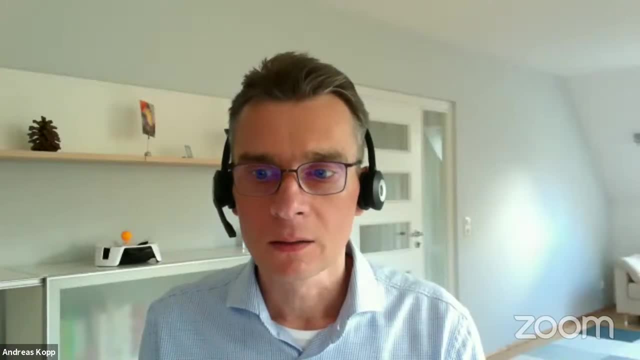 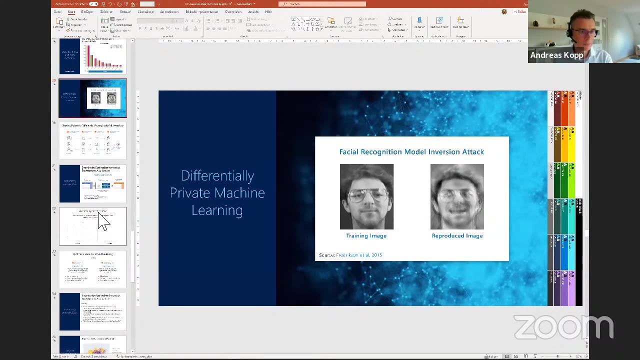 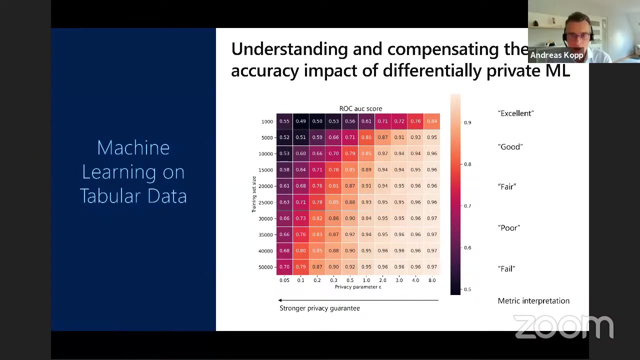 So, Andreas, do you want to take over again? Yeah, So I guess you can see my screen again. We can see it, Andreas. Okay, I can see it, Andreas. Yeah, Perfect. So one of the questions that you find in the white paper again and again is: what's the impact? 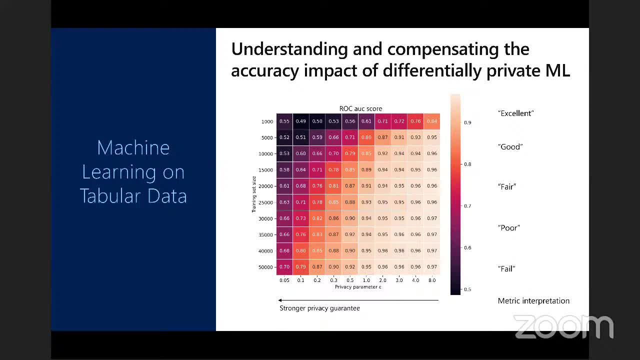 And maybe this also helps a little bit in getting an impression about- well, let's say, guidance- how to choose the epsilon parameter. What's the impact of accuracy of differential privacy? Yeah, So the impact of accuracy of differential privacy at various epsilon levels. so what we are seeing here is a set of experiments that we have done with the same data set Lucas has used in the context of the synthetic example. 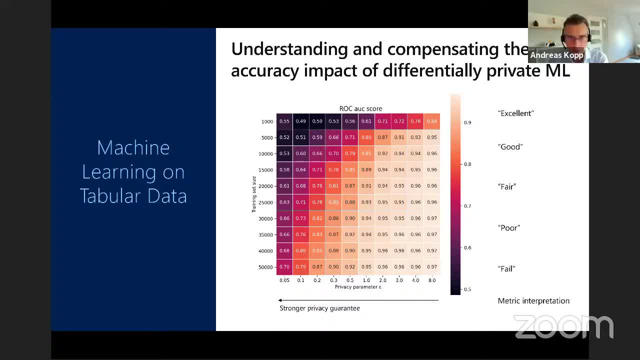 Here we are using actually the IBM differential privacy library, So this is a differential privacy-enabled algorithm which is a Naive Bayes in this context, And what we can see here is at various levels of epsilon and also at various levels of the training size, is the impact on accuracy. 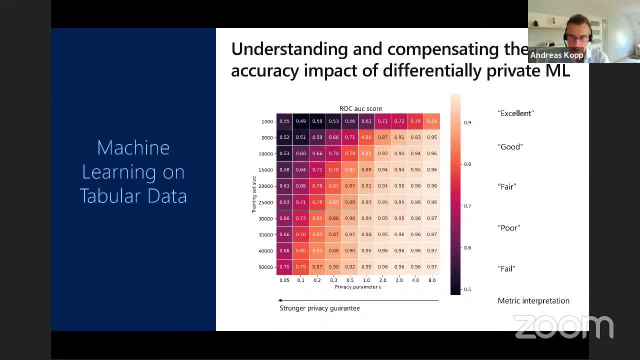 And if you look at the results in a setting without differential privacy, it is quite consistent with the level of an epsilon of eight. The only exception is this one. So if you don't use differential privacy, then this one is Okay. So if you don't use differential privacy, then this accuracy level is higher. 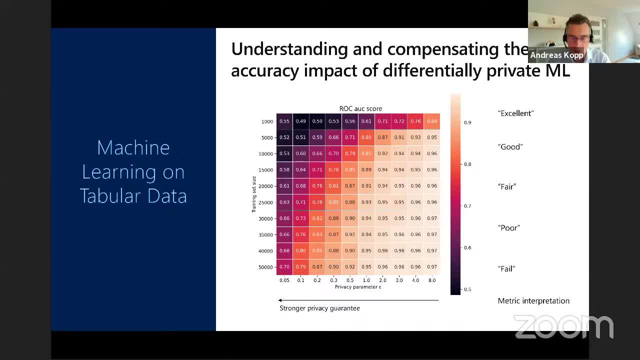 So the main takeaway is really that you can control the amount of accuracy that you lose by differential privacy by carefully looking at the choosing the epsilon parameters, What we, as Lucas, mentioned, so practical examples you can find here. So between 0.1.. 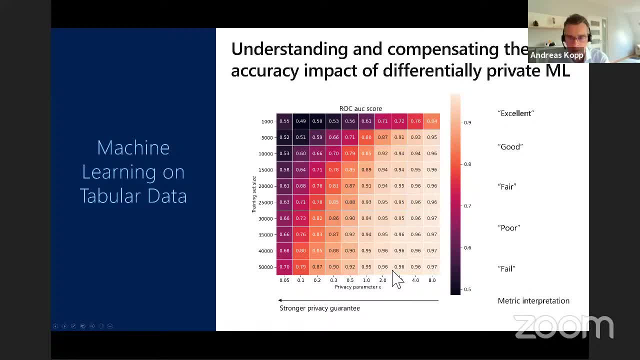 Also, 3.1 or 3 is a commonly used parameter, but that depends on the use case. There are also some economic approaches If you, for example, if you can relate the use case to a risk. So there is a nice Harvard paper, for example, with an insurance use case or a medical use case, where they calculate based on the epsilon value. 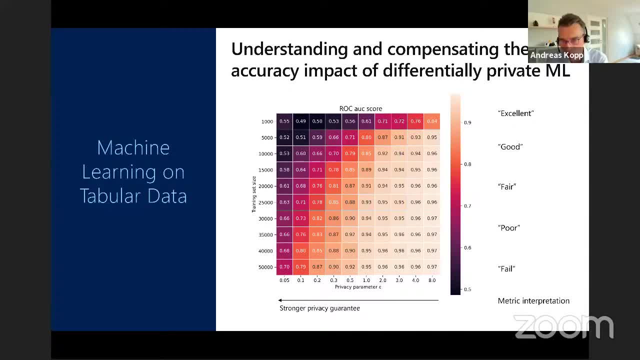 What would be the risk of an increase in the insurance premium based on various epsilon parameters. So there are also. there is a way to even get an economic interpretation of the epsilon parameter, or at least of its impact on expected increase of an insurance premium, in this case. 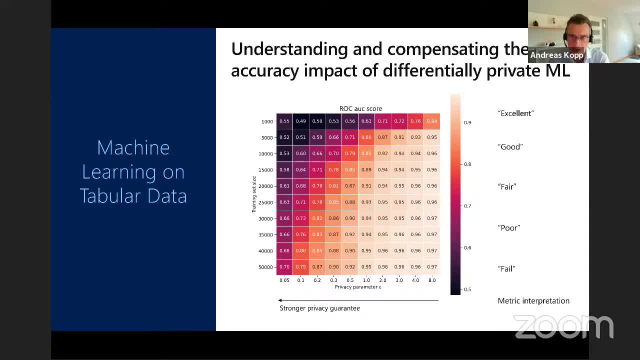 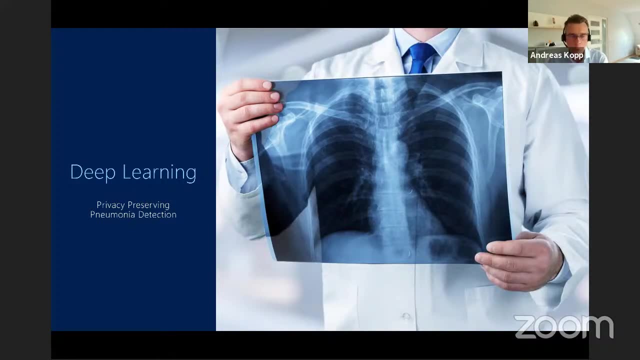 So I think that this gives a nice overview that you can compensate for the privacy Loss if you have a chance to add more training data. And that brings me to the final part. The open question, of course, is what about deep learning? 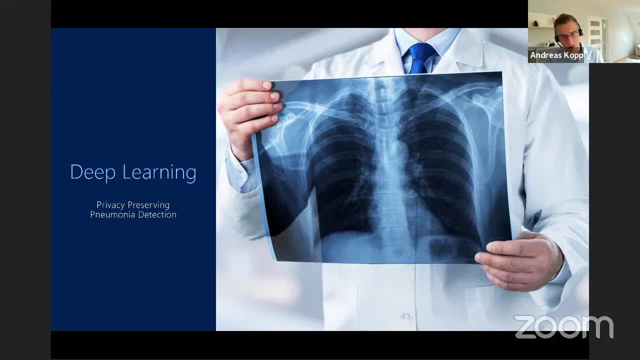 What we've seen so far had been classical analytic use cases, a univariate use cases and also multivariate use cases with classical machine learning. question is about deep learning And this is where obviously there is The biggest risk of memorizing data points, as we have discussed. 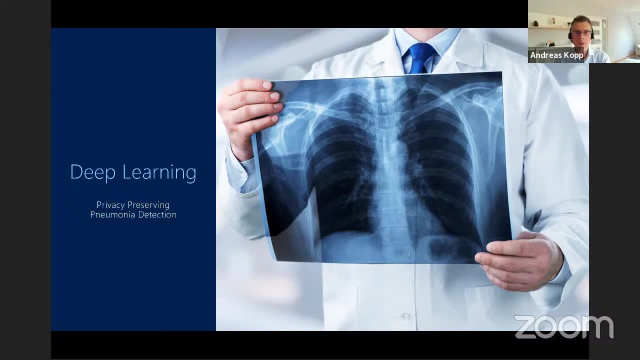 And in the final demo and the final notebook we leverage relatively small medical data set of only 5000 images, So relatively small for deep learning standards. So you can also reproduce the demo with the local equipment. We have Trained it here in the Azure cloud to leverage GPU instances. larger GPU instances. 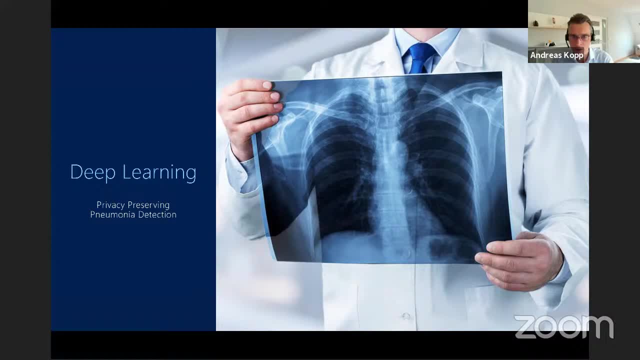 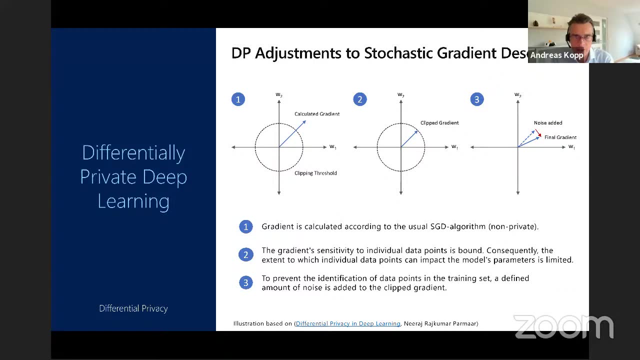 But you should be able to reproduce the demo also based on a smaller equipment, And the way differential privacy works with deep learning is it's relatively straightforward to include it in your existing workflow. If you consider Stockholm Stochastic gradient descent, There are conceptually 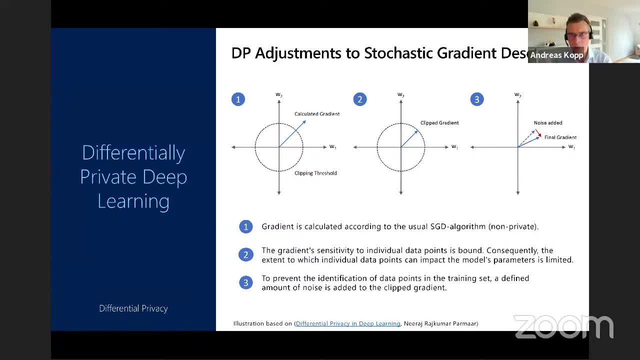 Only a few adjustments To make stochastic gradient descent, which leverages randomness by default. Hence the name stochastic To to add differential privacy To the to. the mechanism One is to clip The gradient, So gradients Can become an absolute terms. 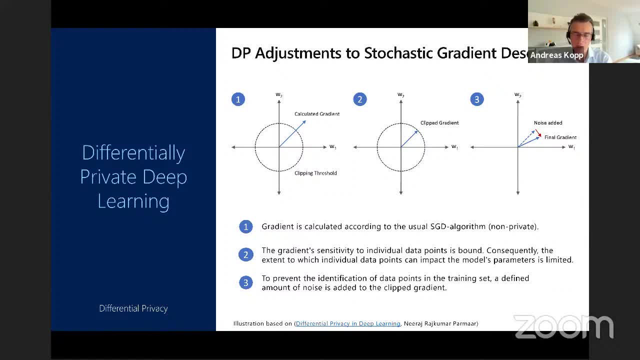 Very large And in order to To reduce or to mask the sensitivity to specific data points, The gradients are clipped. This is Change number one, And the change number two, compared to, let's say, classic stochastic gradient descent, Is that we then add: 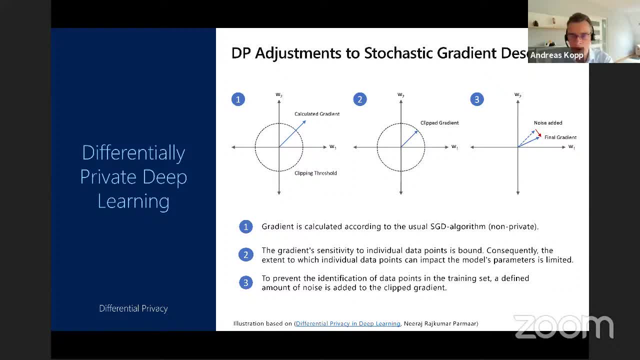 Noise To the clipped gradients And the. the amount of clipping And also the amount of noise Become additional Hyper parameters Which you use in the context of differential privacy, and both The extension for TensorFlow But also the extension for PyTorch, which is called upper cost, which we are using in our demo. 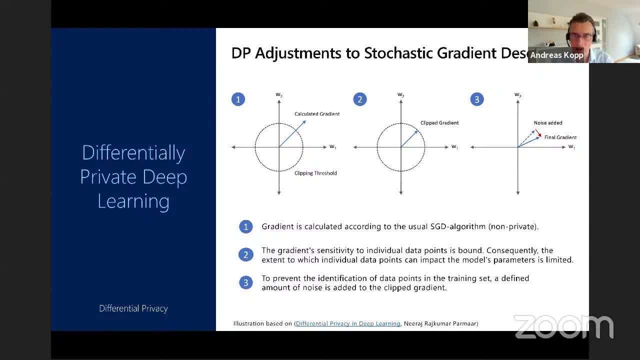 Leverage this concept And in particular for for PyTorch is. it's relatively straightforward to Include that, And what I would like to do is to actually Go through the The notebook And show you how we are doing it. 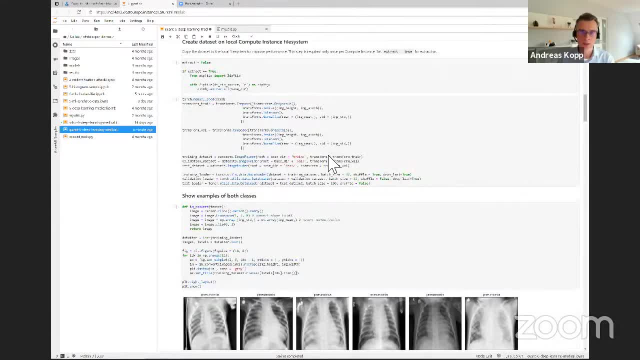 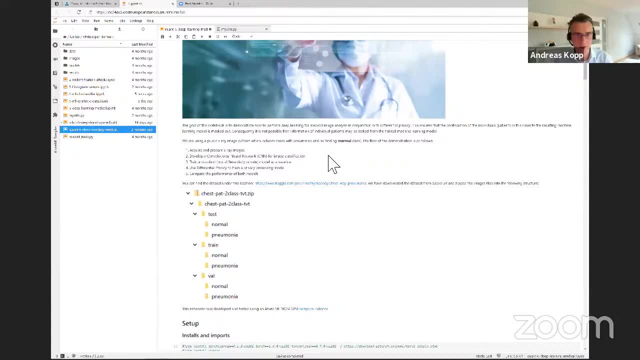 And this Relatively simple Example. So we are leveraging a public data set. It's a binary classification of X-ray images, So Detecting pneumonia versus Normal Wish. Where's this X-rays In the Data set? 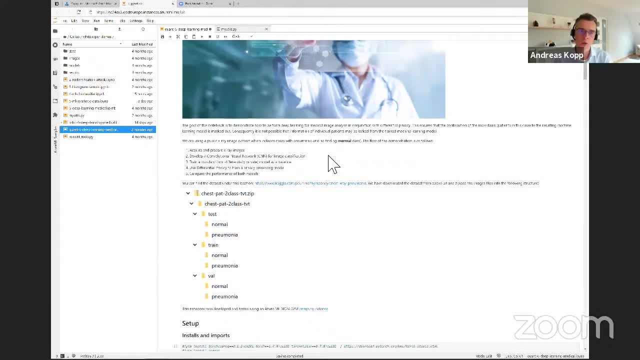 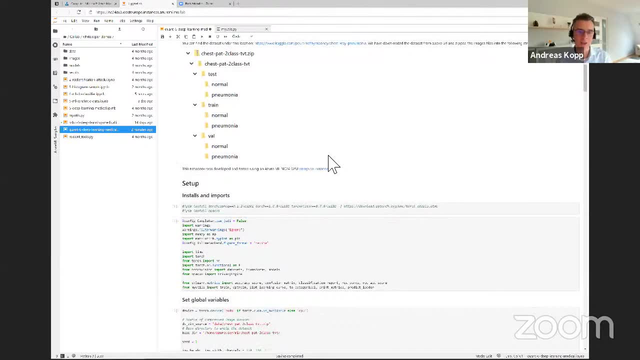 It's a binary classification of X-ray images. So It's a binary classification of X-rays Which show normal condition. It's a, as I said, it's a public data set Which you can use. The advantage is it's relatively small, but 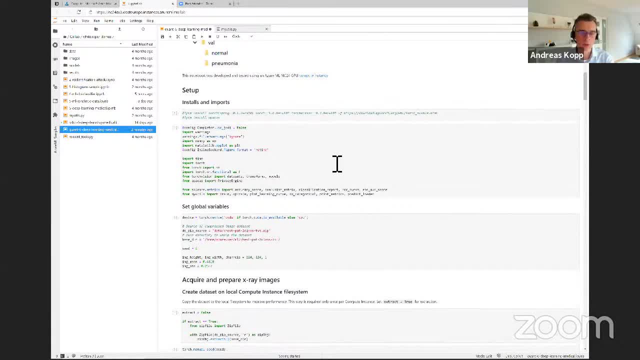 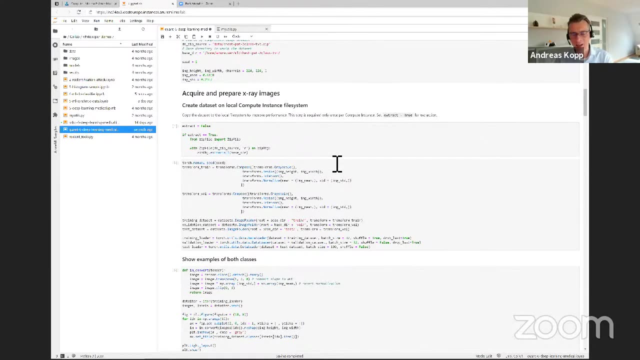 Convergence behavior. It's quite good. So when we are Doing the usual stuff- Importing PyTorch, importing So the differential privacy extension For PyTorch- Then we acquire our Dataset. So We We do not. 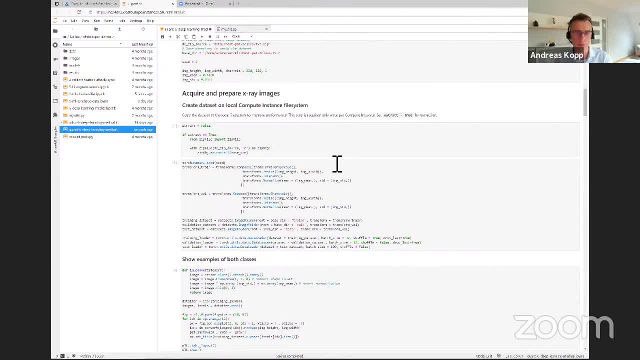 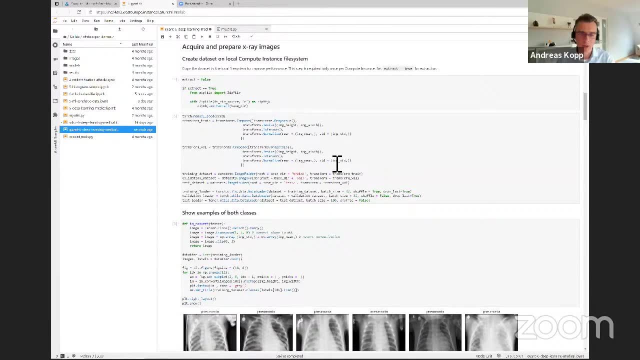 Any. We do not leverage Any kind of data augmentation, We just Use the raw images. Do some normalization, Of course, but no augmentation. No, no, no, No fancy stuff. Here You can see the the images. 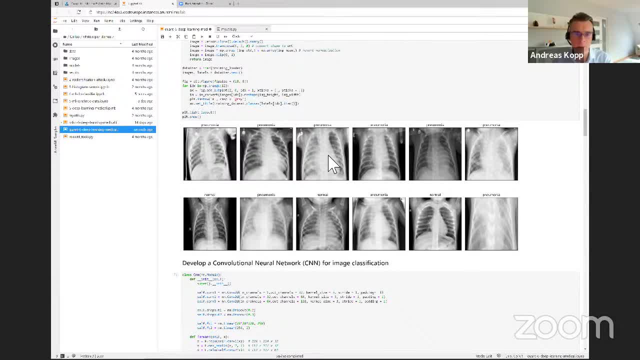 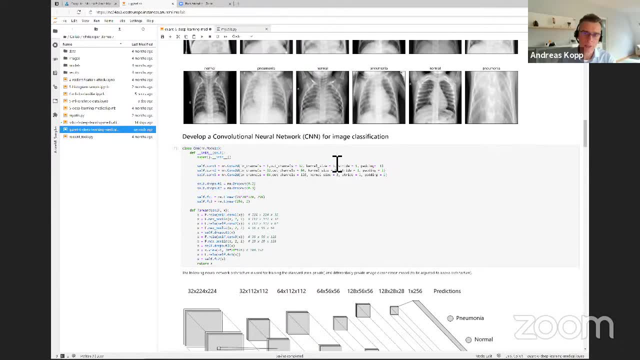 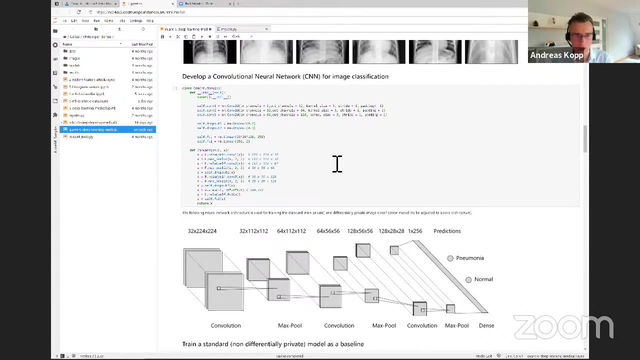 So A couple of random examples, Including normal condition And also Including Pneumonia. Then we Design, Relatively Straight For What See In The Standard Standard, The model of Penetration. 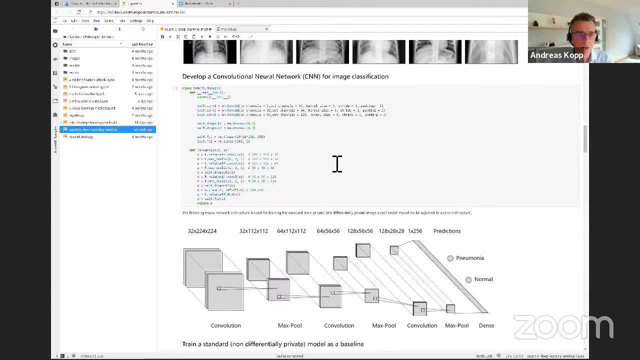 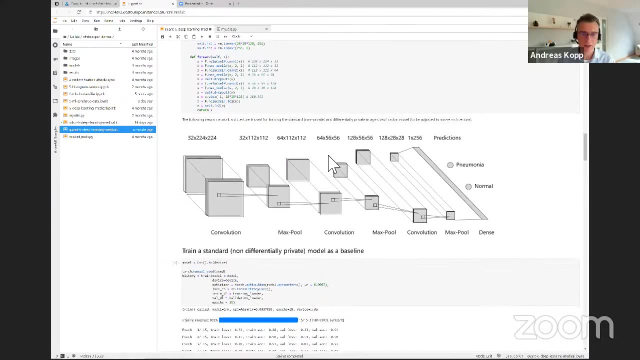 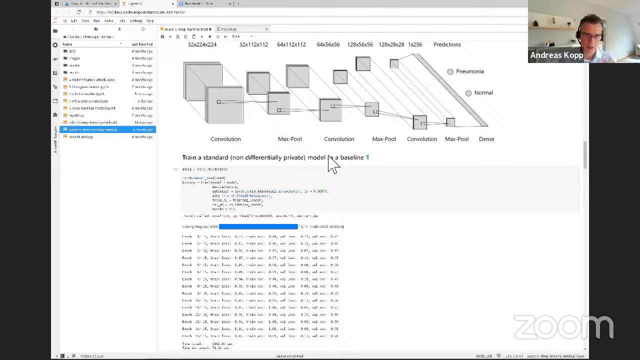 For the Data block And These Materials That We, We Use The Data. Therefore, When We Do Any What Problems, Then We Do Any Thing That Warners. 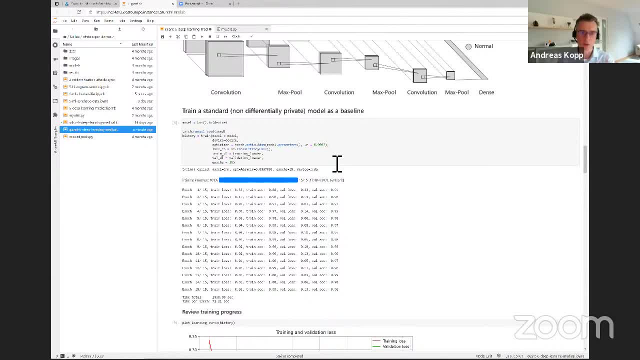 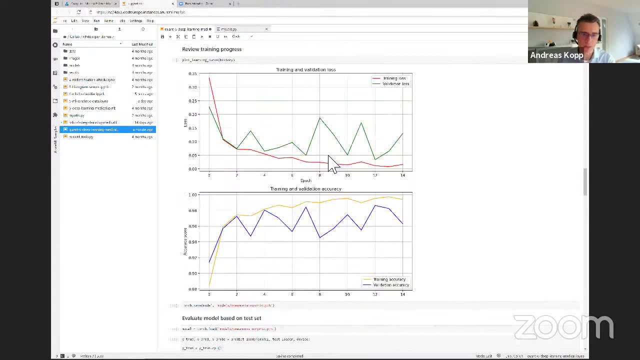 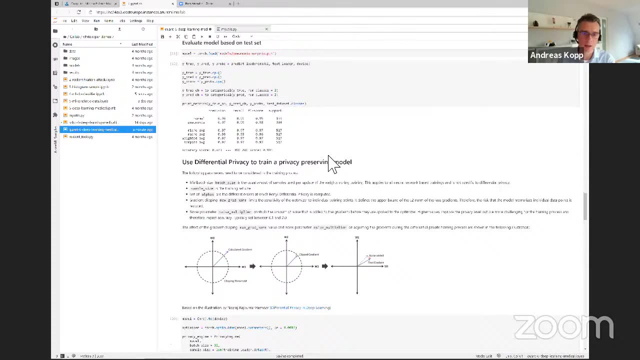 particularly for the performance metrics. This achieves after a couple of epochs, quite a good accuracy, quite a good validation accuracy. And then we are testing based on the test set. So we achieve 97% here. So it's a quite good model. 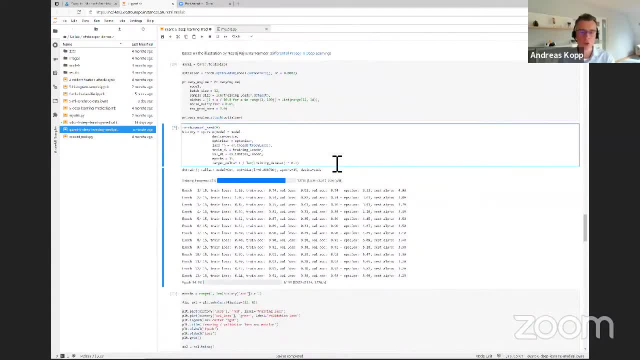 And then here you can see the differential private version. It's not a big change. The only thing is we have to import the privacy engine of Opacus. so the extension for PyTorch, We attach it to the optimizer and we add those hyperparameters which are: 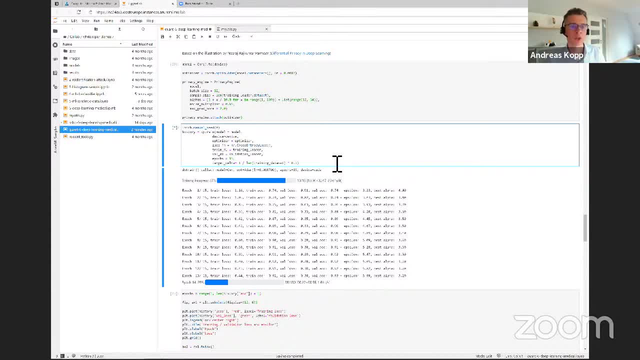 specific to differential privacy for deep learning, which I mentioned. So the amount of gradient clipping and the noise multiplayer, and then there are a couple of other hyperparameters, But these are the important ones. What you can see here is the training process. 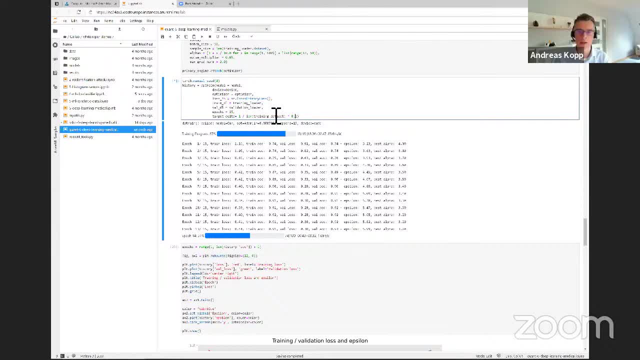 We adjusted the training loop to get Epsilon back per epoch, So we can decide after the training which model, after which epoch we are using, Because now not only we are looking at training loss and validation loss, we are also looking at the Epsilon consumption per epoch. 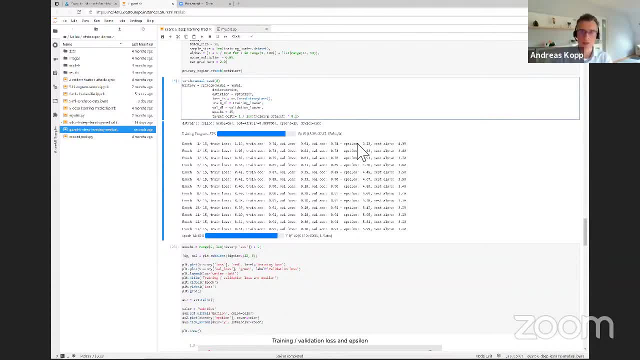 The more often you go through the data set, the more privacy budget you are spending, And so this becomes also an aspect in deciding on the number of epochs is how much Epsilon you want to spend. So that's an additional consideration for the deep learning process. 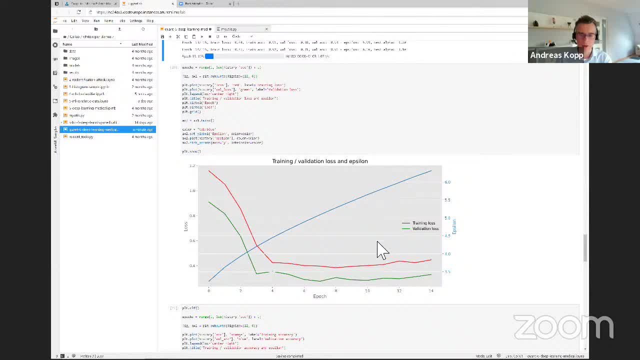 And then we can see the results of the training, so classical parameters Like training loss, validation loss, But also we can see here, in addition to that, the Epsilon consumption, the privacy consumption, And if overall we have an Epsilon budget of, let's say, 10,. 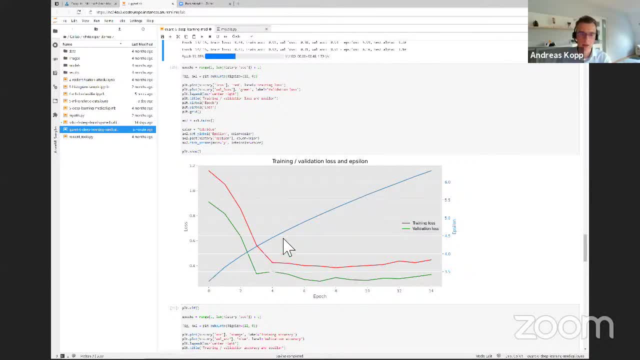 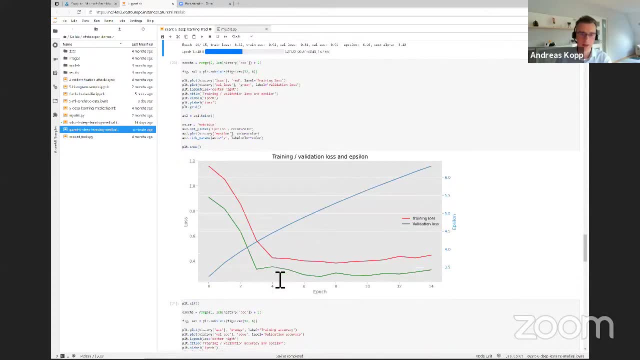 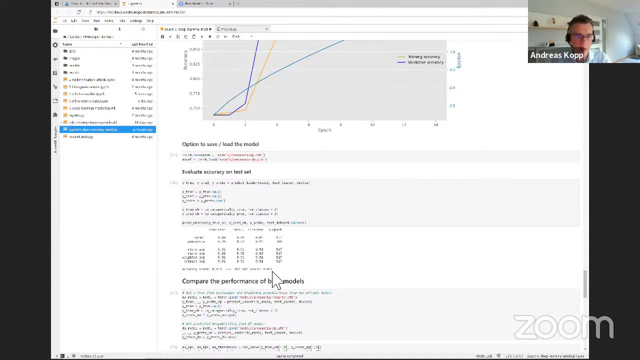 then we would stop here. But we can see that also, considering the loss values, the training and validation loss, it makes sense to do early, stopping earlier, And then we can see. We can see the results here. So we are losing a couple of percentage points. 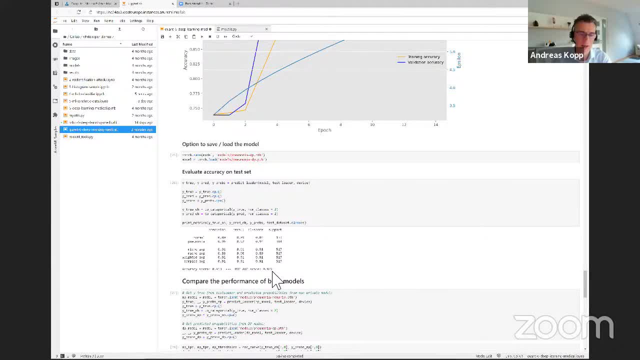 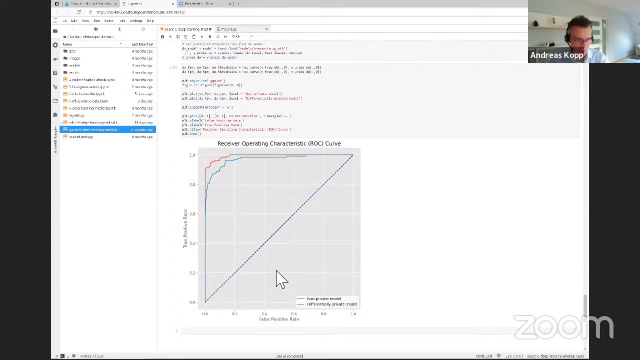 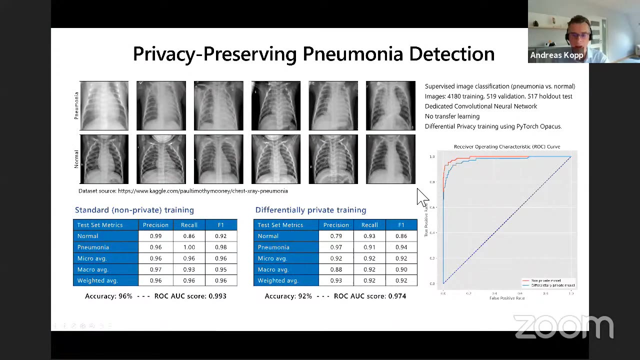 in terms of accuracy. We will compare that on the slide again And you can also see the comparison in terms of receiver operating characteristics. But I think it's probably easier to compare that here in this slide. So, as I said, we are losing a couple of percentage points. 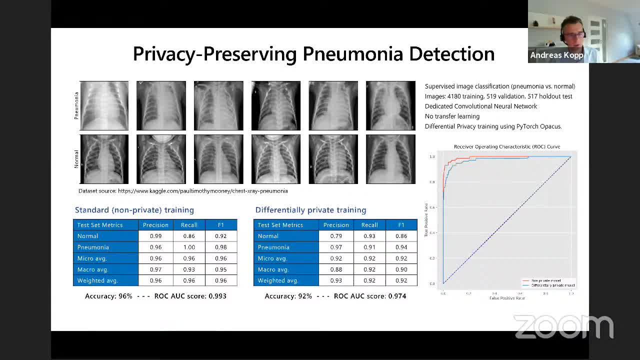 Compared to the standard, to the non-private training it's. in this example, it's four percentage points that we are losing, but still getting quite good results. Of course, this depends on the use case, So if it's a very unbalanced data set. 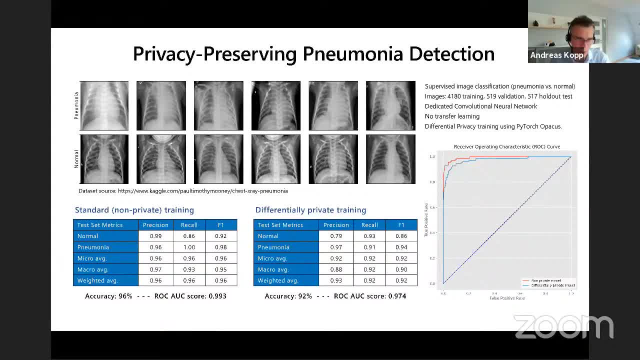 the results will not be as good at what we've achieved here. If you have more classes, of course the world will be will also look a little bit different, But I think it's a general good way to start with differential privacy. if you look at the example, 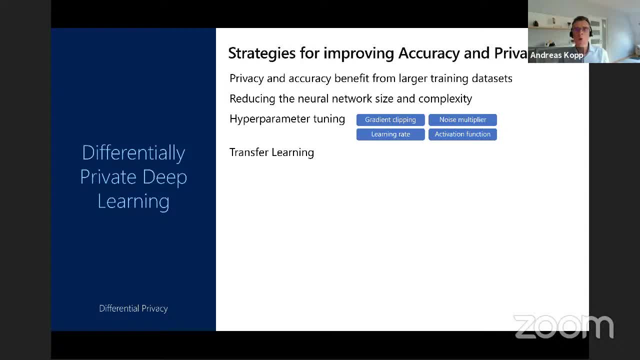 And then there is of course always the question: what can we do to improve accuracy and privacy even further? So the same observation that we had for the univariate analysis and also for the machine learning- the classic machine learning examples- apply. 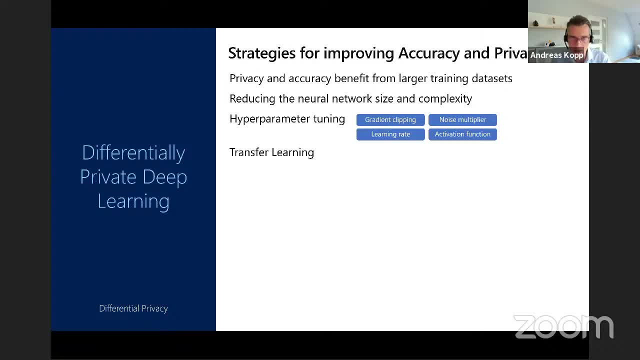 Here. So more training data makes sense, Of course, reducing the network size and the complexity, which is generally a best practice to avoid overfitting in particular also applies to differential privacy Hyperparameter tuning: you get two additional hyperparameters. 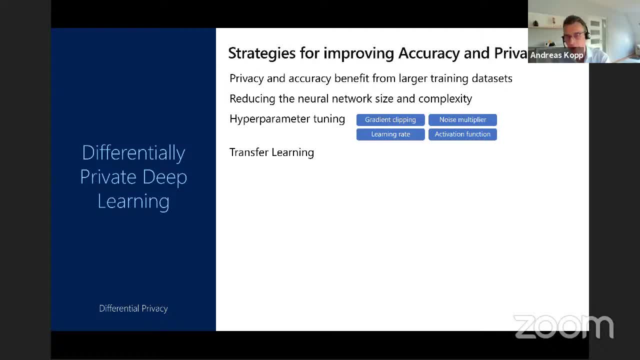 Now we have in addition to the usual set of hyperparameters. you get gradient clipping and also the noise multiplier as additional hyperparameters. But also the classic hyperparameters like learning rate and also activation function have a specific impact on differential privacy. For example, there is some research that bounded activation functions like sigmoid may make more sense than the classic ReLU activation function. 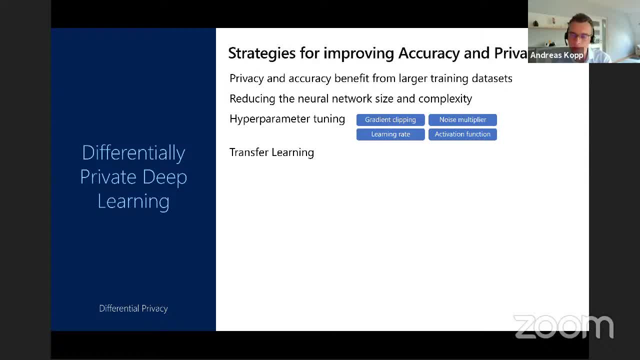 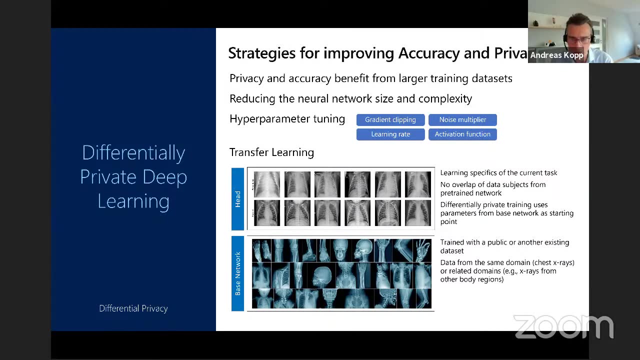 So it has some impact on classic hyperparameters as well, or architectural considerations, even though that we used ReLU activation functions in this example. And then, of course, you can also combine differential privacy with transfer learning. So, for example, if you have a public data set, like in this case, a medical data set which has been trained without differential privacy, 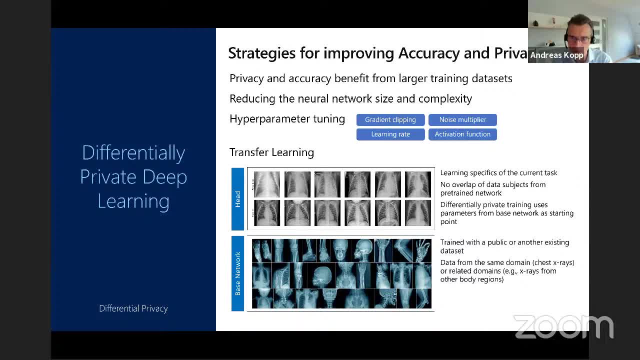 you can train on top of it. And you can train on top of that with differential privacy based for your specific use cases. So there are all kinds of options and variations which help to improve the accuracy and the privacy even further. And the less epochs you need, the better it is from a privacy perspective because you spend less epsilon, so less of your privacy budget. 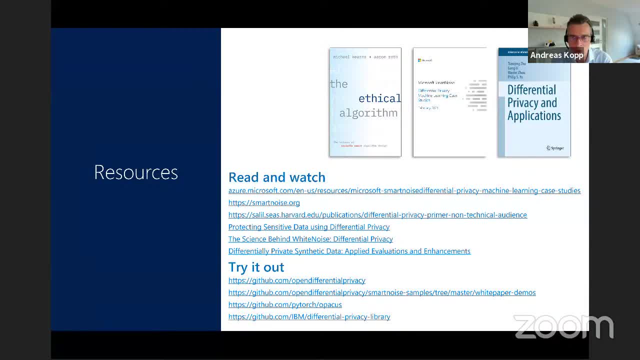 And yeah, with that I would like to conclude. If you have any questions, please feel free to ask them in the chat. Thank you, If you want to learn more about differential privacy and machine learning, I definitely recommend the white paper that we have published. 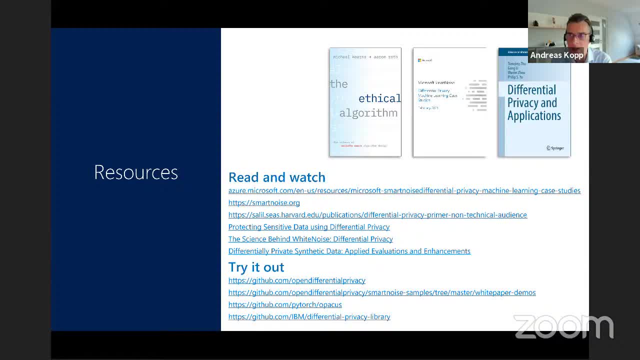 There are also some very good books about differential privacy, like Differential Privacy and Applications on the right-hand side. I also like The Ethical Algorithm by Michael Kearns, which is more a general audience book. There are a couple of recommendations that we have added here. 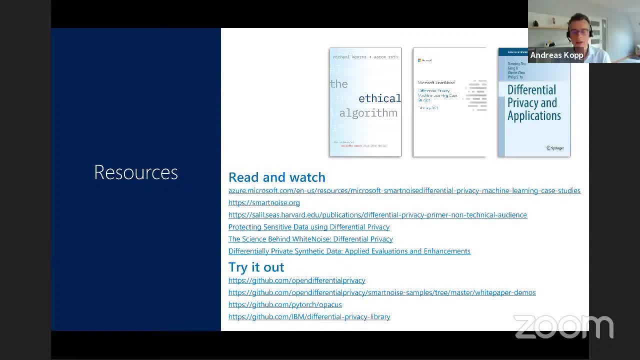 And, in particular, if you really want to understand the background, also the scientific background, behind Luca's work when it comes to the synthesizers, then definitely it's worth to look at Luca's paper And if you want to try it out, here are a couple of links for Open Differential Privacy: the initiative. 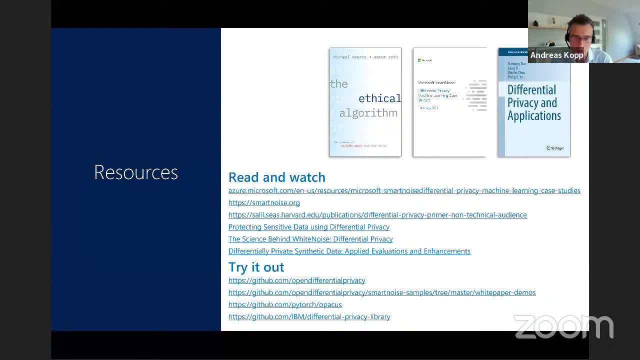 but also for smartphone And also for PyTorch upper-cost. there are a lot of information, there are a lot of use cases and samples. So I think, maybe to conclude, it has a very strong scientific foundation. It reaches more and more practical applications. 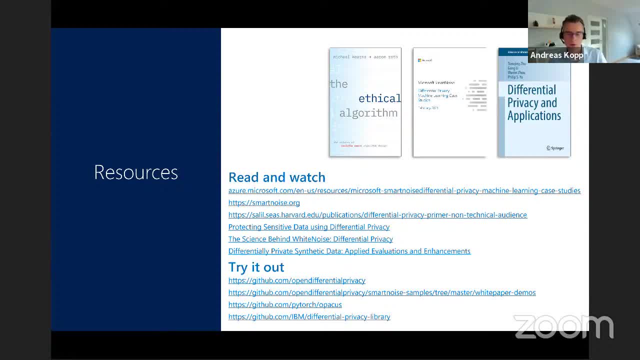 And it's not only the big companies who have a lot of data, like Microsoft, Apple and Google. It's more and more enterprise customers who are looking into the core. It's more and more advanced companies who are looking into the core. So I think that it's a very good concept, also combining it with other interesting and promising concepts, like Federated Learning, for examples. 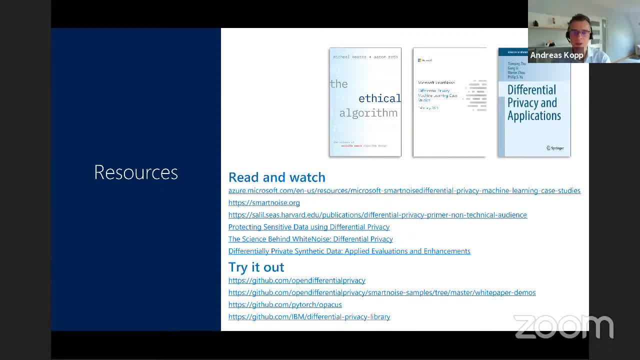 I think one kind of a moonshot application is the decision of the US Census Bureau to provide the release the results of the 2020 census, also based on differential privacy. It has not been released so far, but I think this will be also mean it give a big push for the technical and technical aspects. 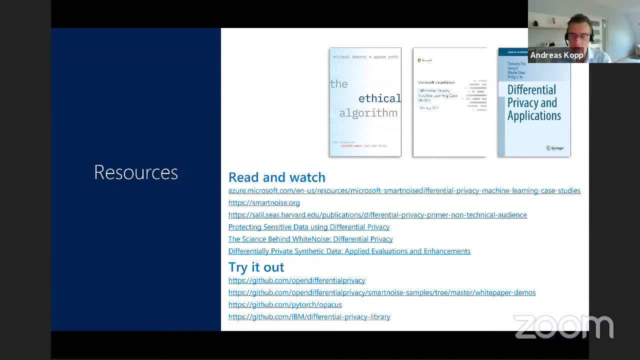 technology And, yeah, as I mentioned, so the evaluation is that a differential privacy is the, or at least the upcoming, gold standard for privacy protection, So it's definitely worth to look at the developments of this technology. Yeah, maybe, Lucas, is there something? 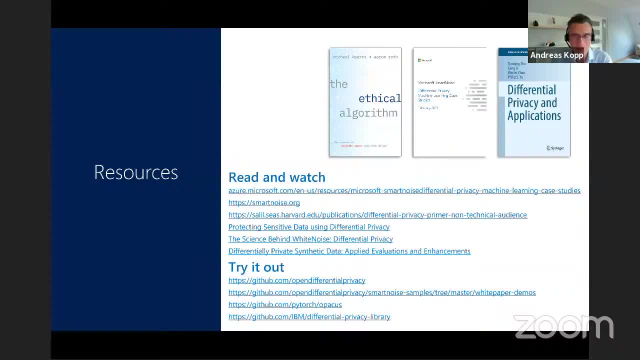 you would like to add: We have a couple of minutes to answer questions And also, if there is maybe interest to go a little bit more into your, into the paper, into your work. Yeah, nothing to add. I'm happy to answer more questions at this point. 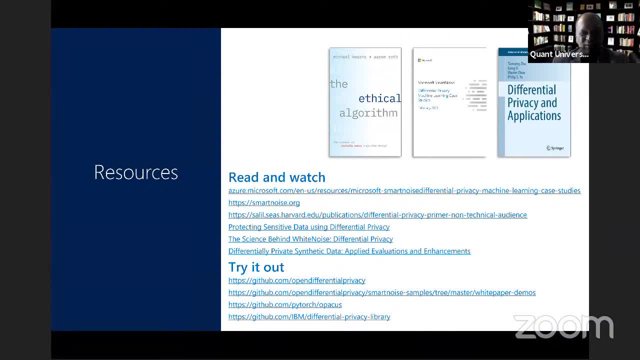 I think we have a thriving discussion board And thanks Lucas for, you know, parallelly answering questions as Andreas was speaking. This was very insightful And we will be posting some of the links You have shared with us, both the papers and also the slides- to the audience so that people can. 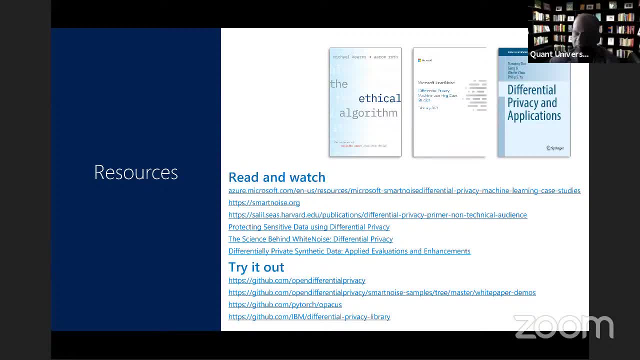 follow up. Now. I actually had a question, So this is all fascinating result of you know things you've been working on. Now, from a pragmatic perspective, you know if you're thinking about a bank, or if you're thinking about a healthcare organization and or even 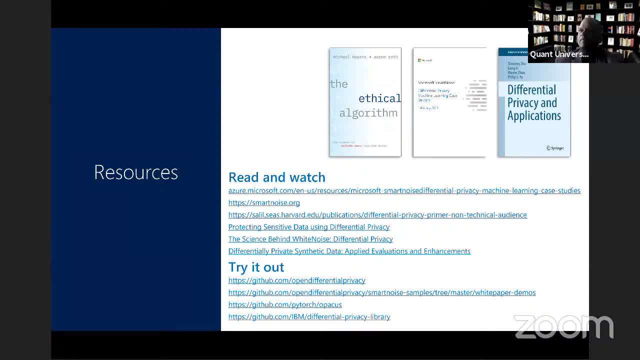 the government right. So there are a lot of you know defense and you know common use cases wherein this is going to be extremely useful. Now, with respect to the roadmap, where are you seeing? you know the, the progression, you know. 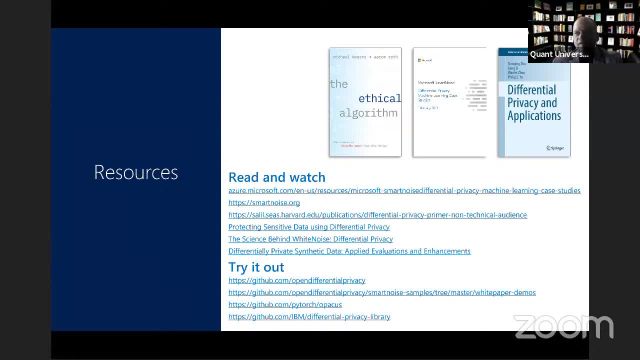 you have also talked about the IBM's efforts in this and also Harvard's efforts in there. So how do you see the roadmap for Microsoft and what you are building in terms of tooling Is it? is it more in the context of evangelizing it, Or you're thinking more package solutions to differentiate? 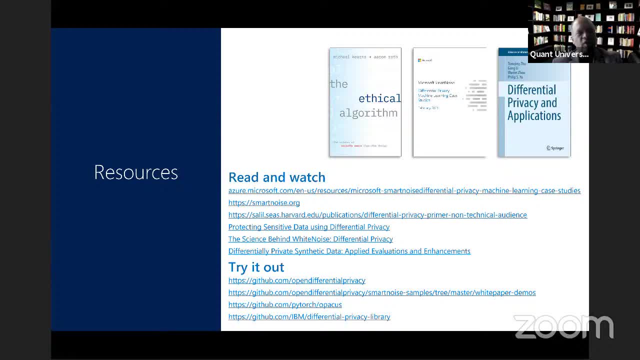 differential privacy as a service kind of notion, Or how do you see the roadmap for interpretation? Yeah, maybe let me try to address the question on a high level And maybe, Lucas, you can give them more details about the smart noise roadmap and specific about the synthesizers. So I think 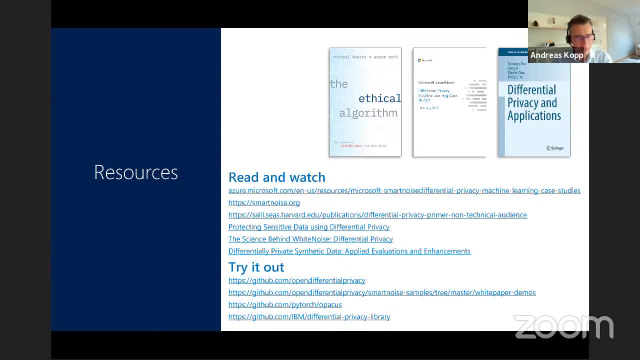 in general- but that's my personal impression- is that differential privacy will probably become more a standard for privacy protection, maybe to the same extent that we'd to de protect data based on anonymization. So the concept is relatively new. I think the first public publication was 2006, by Cynthia Dwok, So it's a 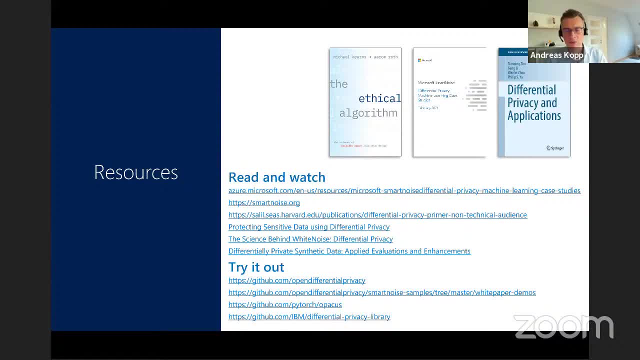 relatively new concept has a strong scientific foundation and not only, but also it also spares a lot of time. Now you know, the big companies started, like Apple, Google and Microsoft. Now it has already been more and more applied also in, let's say, non-technical enterprises. 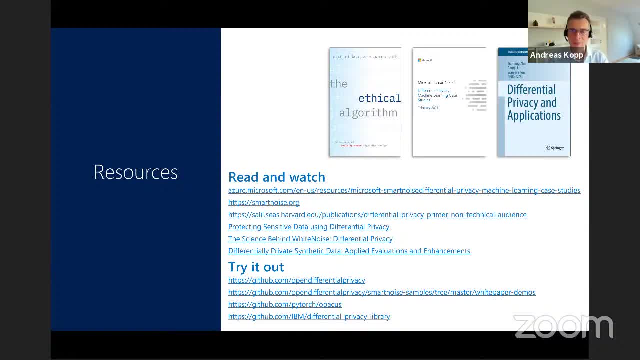 So for Microsoft, I think the trend that we already started is that we leverage itself for our technologies. everywhere where privacy preserving is important, like diagnostic data, This will continue, so it will be included definitely in our products, but also in our offerings. 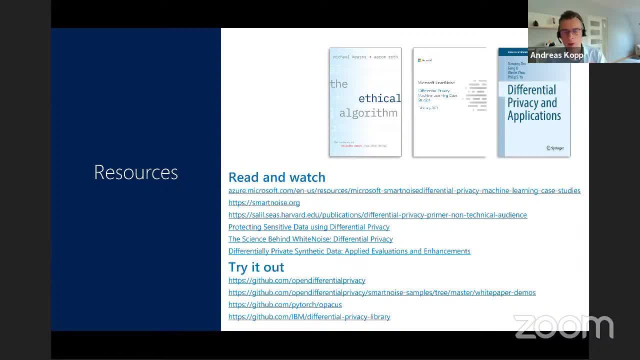 So the work that we are doing with Howard, with the community, this will go on and it will also be included in the Azure machine learning platform. So we typically start with with open source initiatives, but as for the other frameworks like Fairlearn or InterpretML, 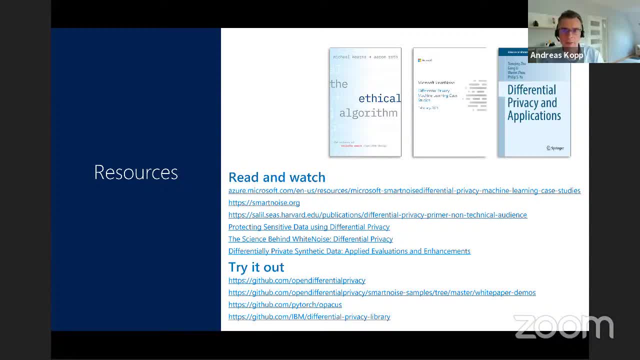 for fairness and for interpretability. it also comes into the machine learning platform. I cannot make any commitment for smart noise, but I think it would make sense to also include it to our, let's say, commercial machine learning platform, where we also start. 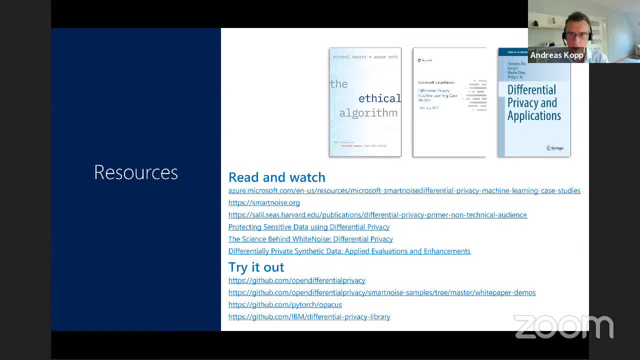 Generally, we start with the Azure machine learning platform, The open source work, and I don't know, Lukas, if there is anything you can talk about roadmap-wise for smart noise or for the synthesizers Beyond the early adopter program. I don't think there's anything else I can say, particularly except that 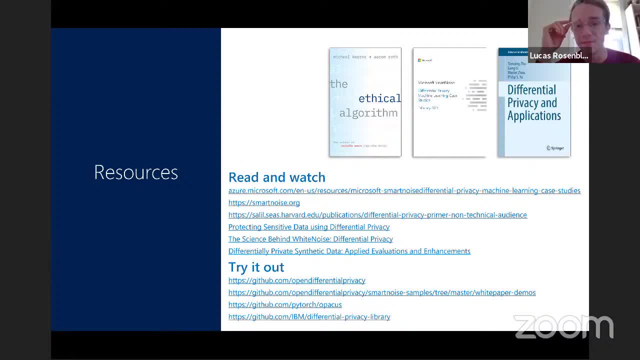 you know, I think one of the main goals is for customers and just generally data owners to ask for differential privacy or as a privacy guarantee when handling their data. So you go to a machine learning practitioner and you say: I have this data, can you do some data analytics on it? 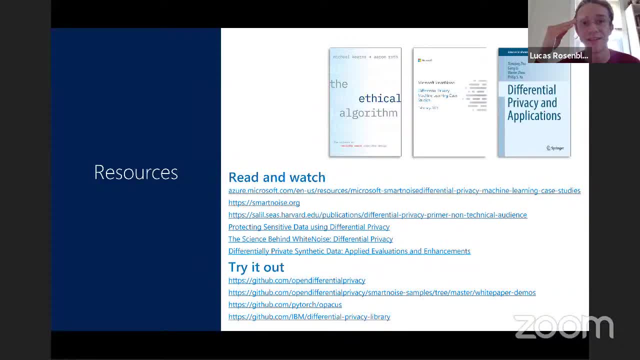 I would like for those analytics to be differentially private for these reasons- And I think you'll see that come to the fold in the next few years more and more. So you know, smart noises and similar efforts are just a way to provide toolings to people where those toolings don't exist. with you know, try to lift the abstraction. 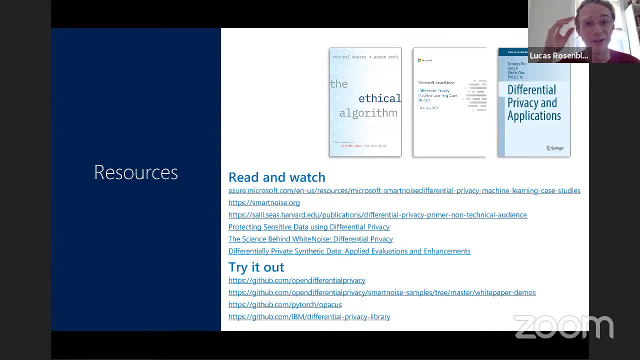 smart noises and similar efforts are just a way to provide toolings to people where those toolings don't exist. with you know, try to lift the abstraction. with you know, try to lift the abstraction off of the off of the scholarly literature and into people's hands and to make it open source. so people can, you know, look under the hood and see how the model is actually providing these assurances, because, you know, fundamentally, adding noise, according to you know, these, these definitions of these mechanism, proofs isn't, you know, it's not too crazy, you know most people can understand it, at the very least the intuition behind it. 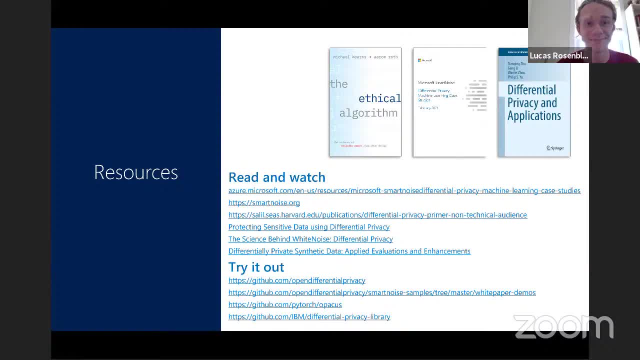 And so that's important And that's an important step to getting adoption. Yeah, absolutely. I actually have another follow up question. So we do a lot of work in this notion of auditing models, right? So? and when you audit models, you look at the whole pipeline, you know, look at the data which was used to train these models. 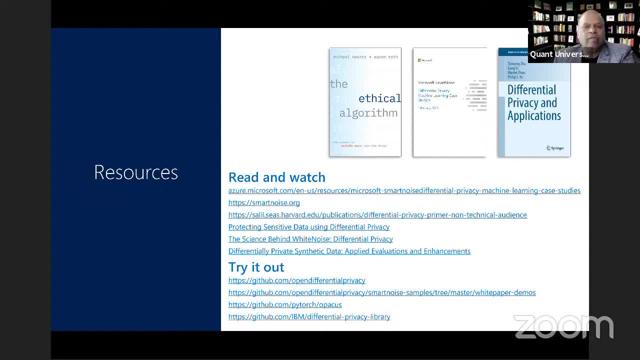 And when it comes from a third party auditors perspective, data sharing becomes an issue, And especially if you're working with private data sets Now. have you done any work in terms of replicability Wherein you know the data was trained locally with real data? 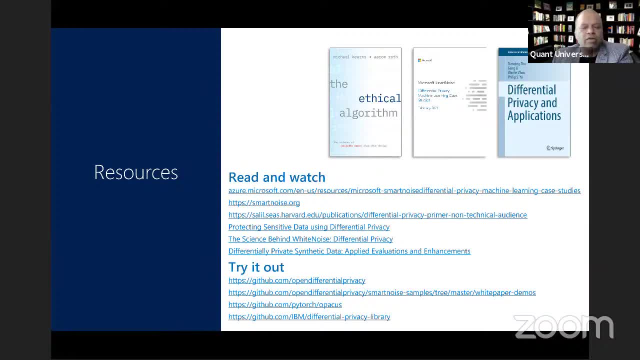 But when it comes to you know giving it to a third party, you want to be able to replicate, but they're potentially leverage. you know differential privacy and create synthetic data sets but have the same kind of paradigm. So I'm wondering, from a replicability perspective, comparing and contrasting, you know, for training. have you done any work on that area? 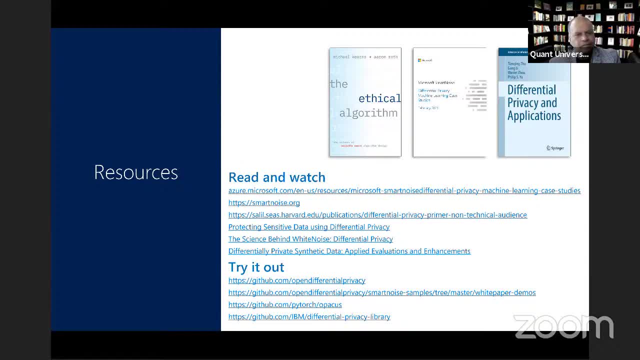 And is this going to be a potential solution there? So do you? Do you mean you've done some model training or data analytics on the original data and then you want to share it with the third party without you know, compromising anybody's personal information? 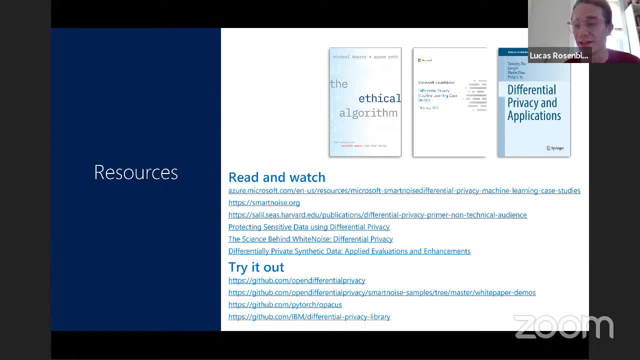 Yes, this is a very common scenario And I think that one of the questions I received in the chat sort of touched on this and on my answer, which is to say that some differential- it's scenario dependent- but there are existing differential, differentially private mechanisms that will give you a lot of data. 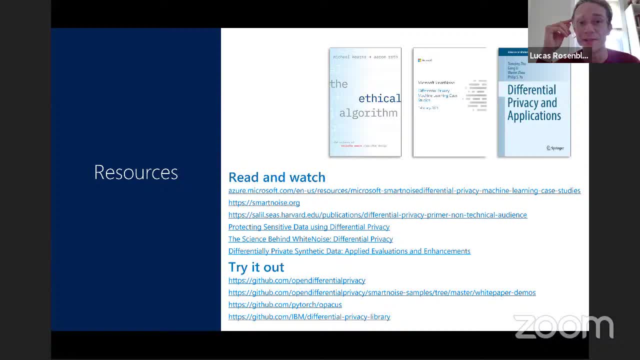 So do you mean you've done some model training or data analytics on the original data and then you want to share it with the third party without, you know, compromising anybody's personal information? And I think that one of the questions I received in the chat sort of touched on this and on my answer, which is to say that some differential- it's scenario dependent- but there are existing differential, differentially private mechanisms that will give you comparable, if not match, the performance you saw on your, you know, whatever your local machine or your local system on that third party system, without compromising person's data. 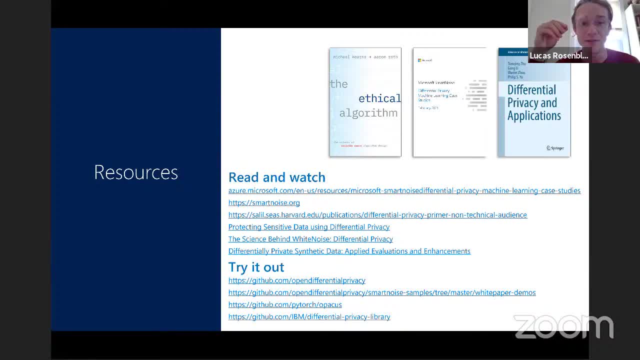 But you will see usually some amount of loss. you know there's some cost to that privacy And it just varies so widely it's sort of hard to speak to Now. there we did present some. I mean there are some tools that are pretty robust to a number of different scenarios. 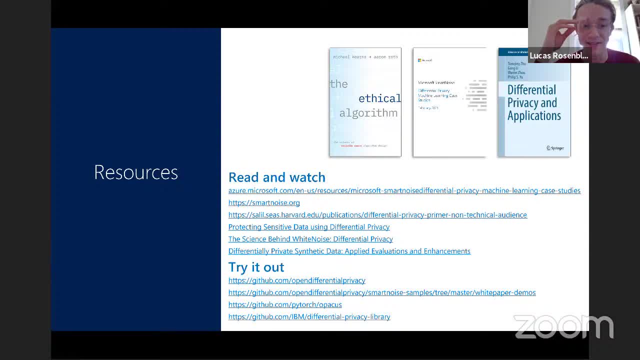 So, yeah, I think this is where the data synthesis is coming, because if you can create a synthetic data set that has, you know, aggregate utility and you can just share that one off with the third party, you know, without having to focus on specific, you know differentially private classifiers or models that you, that you feel will that you then have to work with. 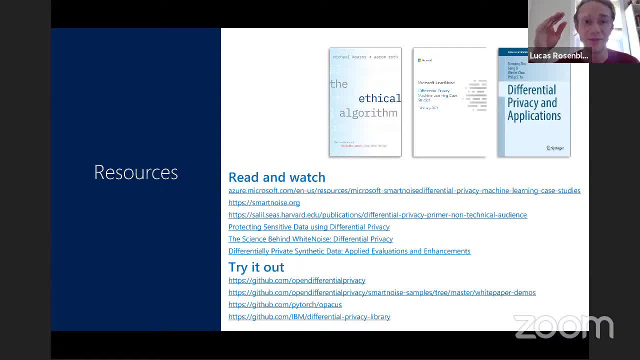 If you can just share the data one off, say here, use this, and it's good, then that sort of green lights a bunch of scenarios that that are common without you know the sort of handholding we currently have to do with: differential private classifiers and specific tuning and whatnot. 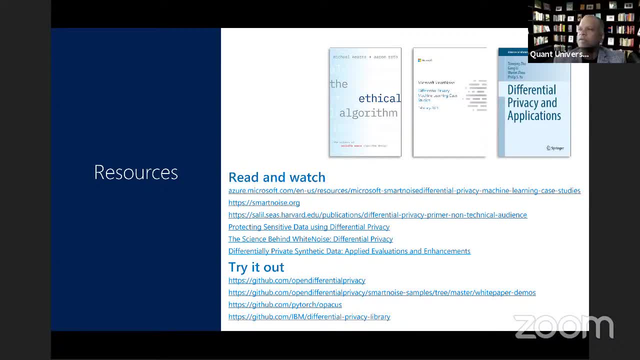 Okay, cool. And what are your thoughts on approaches for temporal data sets? I'm not hugely familiar with the literature on this. You know lots of models could be trained with temporal data Specific to that. I don't think I have enough background to say anything interesting. 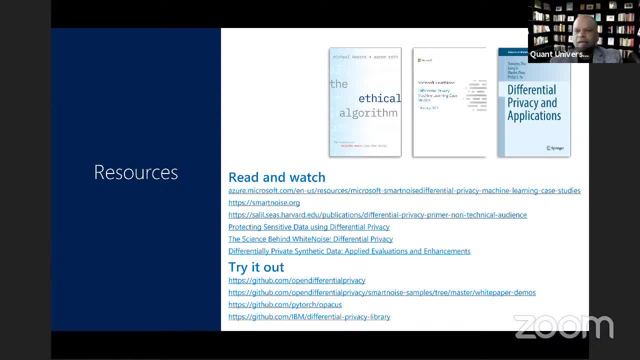 Okay, cool. I think there are a couple of questions on the web, So where can we see a definition of prior differential privacy? Well, Andreas did share his white paper and also textbooks and a couple of sources, So I think that's probably. 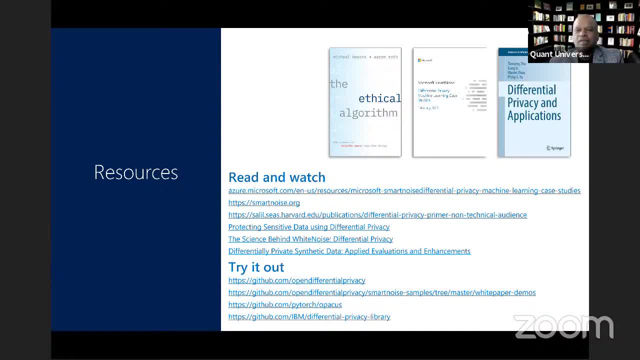 the answer And the final product of your implementation of differential privacy. I believe you know some of the links we posted earlier. should give you some references out there. Yeah, and I'll link the book that Cynthia Dwork wrote, which is open source. 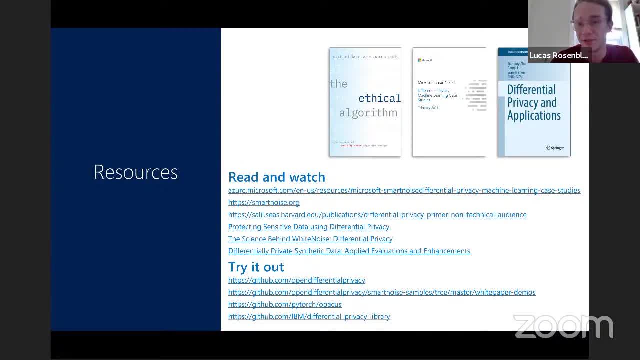 And it's a very good textbook. It's very good, So I'll just drop that in the chat as well. Okay, cool, Awesome. So it's exactly one o'clock. Unless there are specific questions, I think we'll take one last question from John Starr. 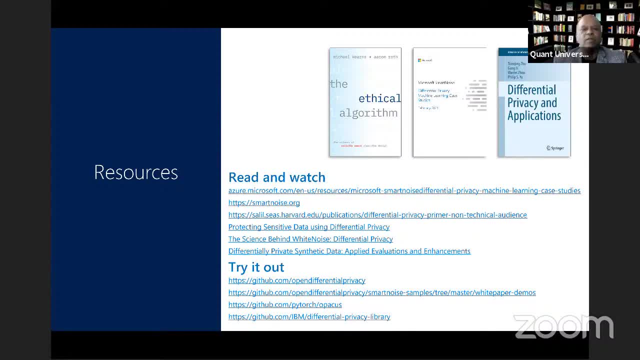 What am I missing with X-ray diagnosis? How is it possible to justify any loss of accuracy? Even 97% accuracy is not ideal, So I guess it's a skeptic question. Any thoughts on that? Yeah, I think it's really. 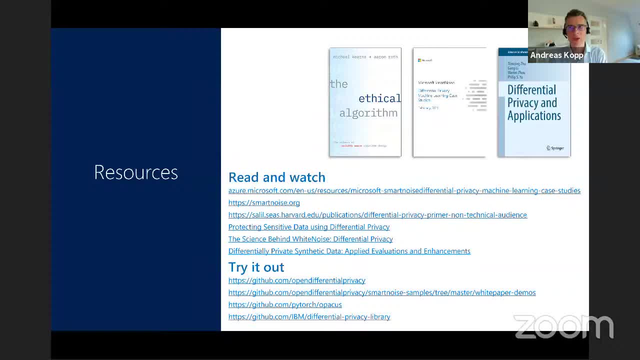 a question of perspective. If you already have a data set to motivate a data scientist to do differential private training and obviously losing accuracy, I think the motivation is not very high. but I think that's not really the story. The story is: 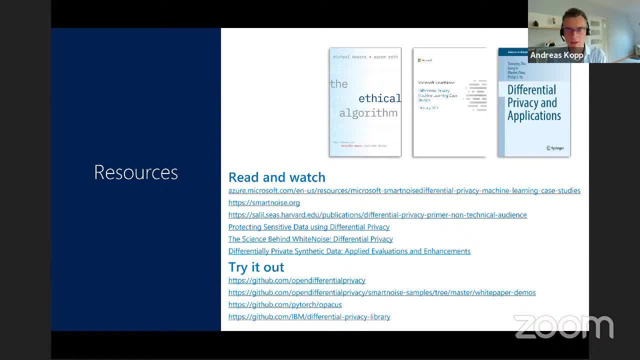 that differential privacy, if you consider it end-to-end, will enable use cases that you currently cannot do because you have not access. you get not access to the data set at all. So I would more consider use cases that you cannot do currently because the data owner is not willing to share the data. 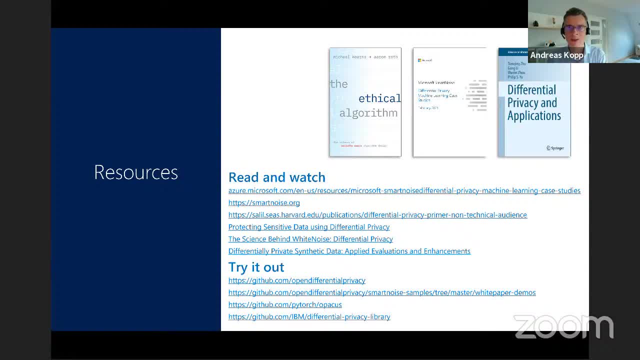 But if you can give a guarantee based on differential privacy, that there is no risk or almost no risk, If you can use the data for research purposes, for example- then this opens a door that you can use it at all. Or another alternative could be: 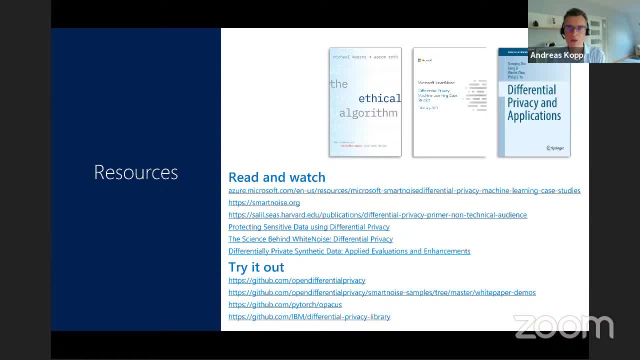 that the data owner requests the data anonymization because he or she is concerned. So it's really a question what the scenario is. If you have a data set and nobody is concerned about the data, then you will probably not use differential privacy, because then you just see. 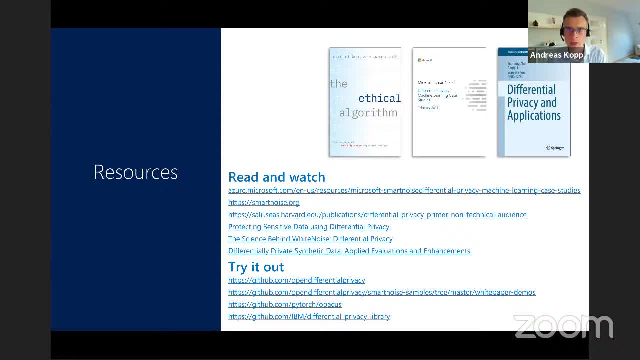 the data that you have. So that's really the impact on utility, But I would really more think of it as scenarios that are enabled because the data owner is not willing to share any data if there is no formal guarantee. Absolutely Yeah, thank you so much. 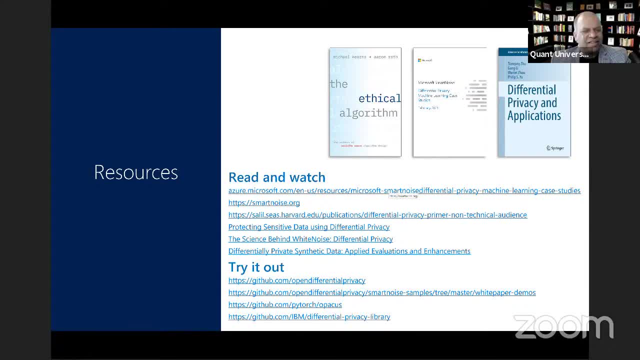 This was a very enlightening and a very fascinating discussion And I appreciate all the rigor which went into putting together this workshop. I again thank Andreas and Lucas for taking time of their busy schedules and presenting at the Quantity University Spring School And we will follow up if there are any questions.